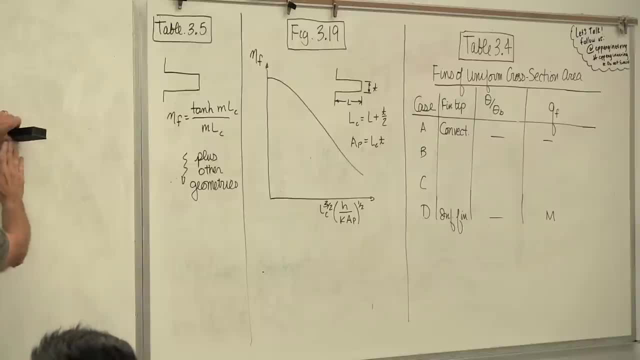 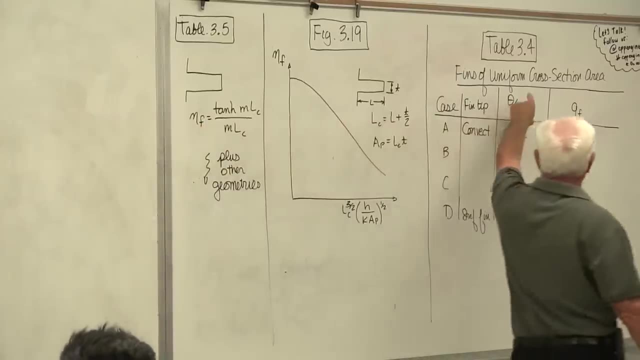 The area is T times W. Slice it near the wall. The area is T times W. A sub C didn't change. It's a fin of uniform cross-section. I can use this table for this fin. Okay, now there's an alternative. 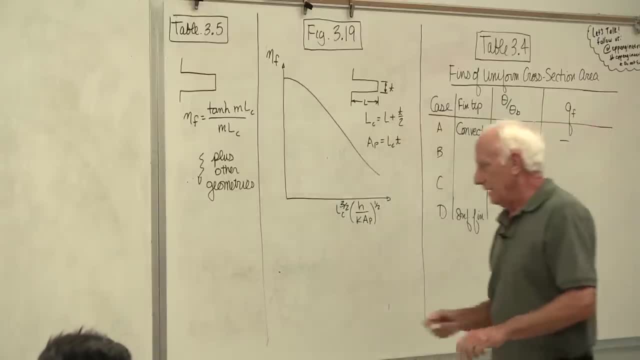 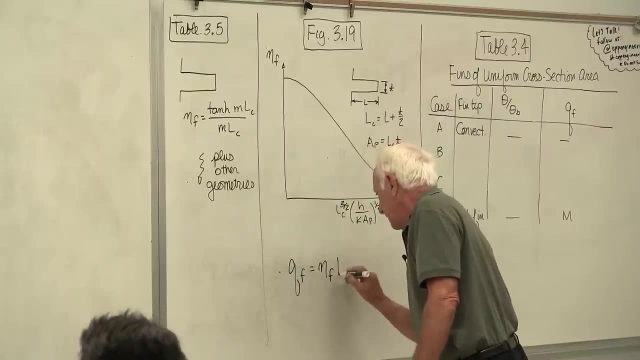 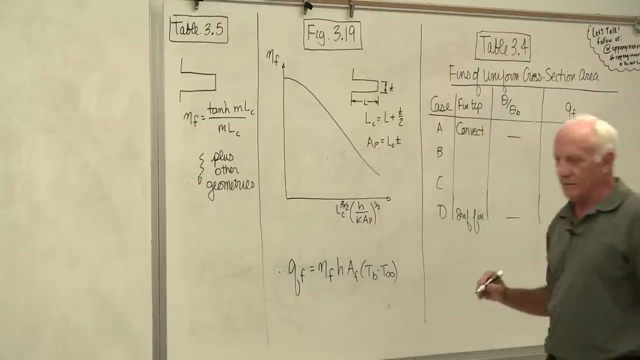 You can also determine the fin efficiency. The way you use the fin efficiency is to find the heat lost by the fin. Take the fin efficiency times H, times the area of the fin, times T base minus T infinity. That's how the fin efficiency is defined. 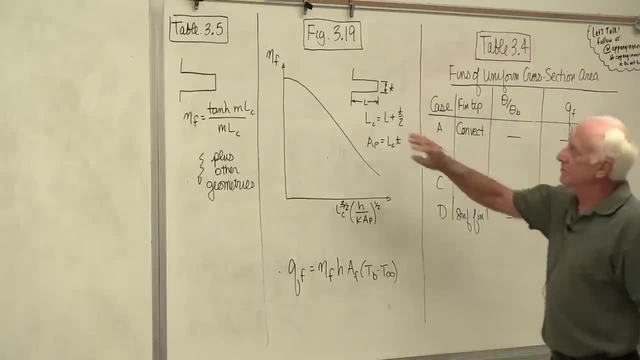 Okay, so to find the fin efficiency, let's say there are two graphs, figure 319 and figure 320.. We'll look at 319 as an example of this. This is for a rectangular cross-section fin like the eraser. 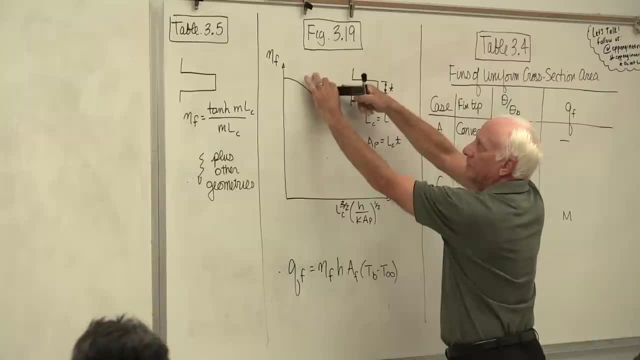 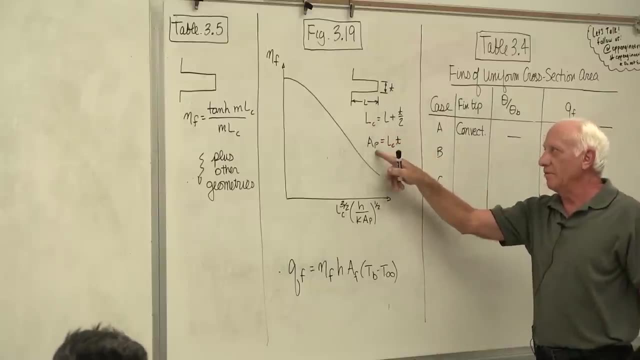 There's the eraser. Stick it out from the wall like that. This is L, This is T, This is W We talked about last time, the corrected fin length and the profile area. Here's how you calculate them. You put the L sub C. 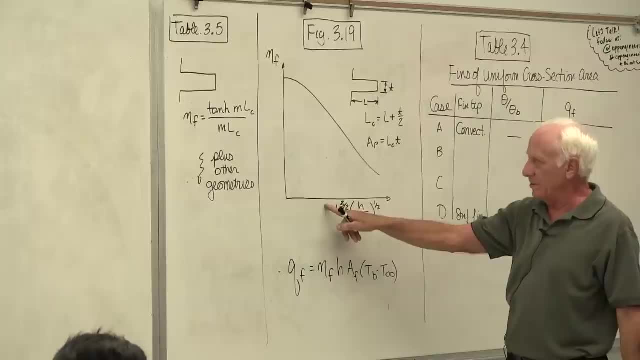 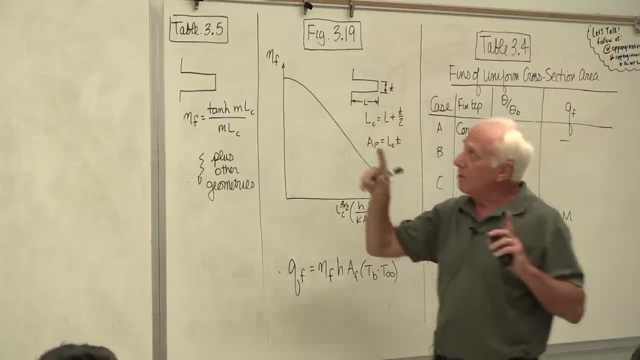 and the A sub P. down here You get the X value parameter and then go up vertically to the line, across horizontally and get the efficiency of the fin. There's also triangular fins on this graph besides rectangular fins, Or you can go to table 3-5.. 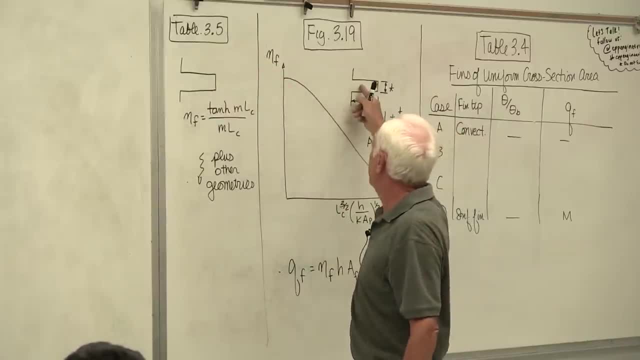 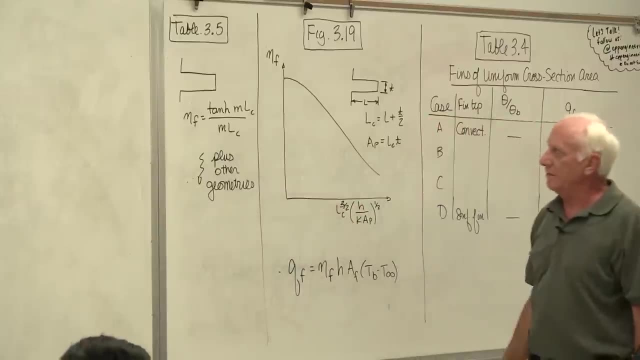 Rectangular fin right here, just like this one right here, except now there's not a graph, but an equation. Fin efficiency, hyperbolic tangent M-1.. MLC divided by MLC Plus. there's about seven other cases of different geometries. 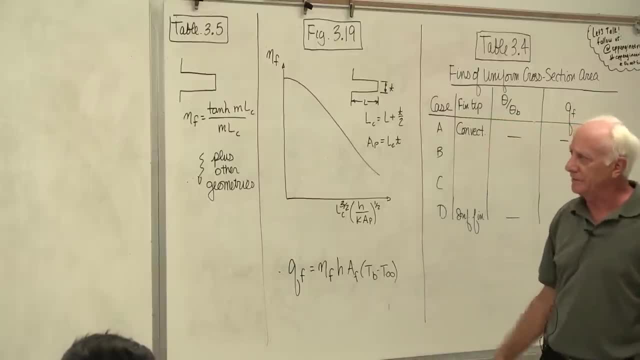 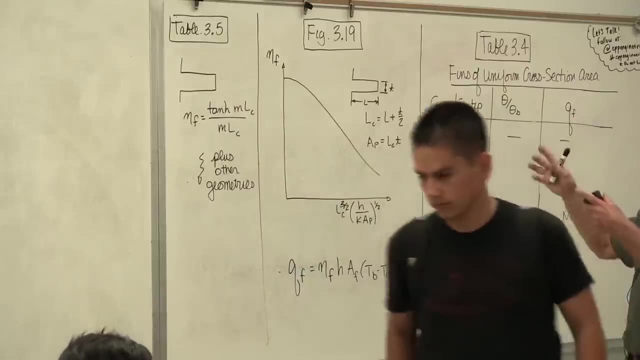 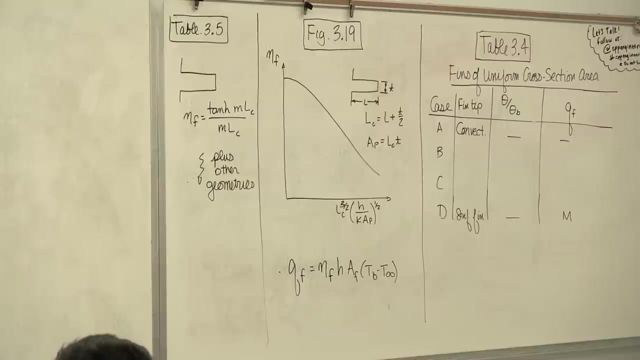 Triangular circular, so on and so forth, Pin fins. these are all given a picture and an equation. All right, so you've got three resources to kind of look at. there We're going to work a problem and see how we go in there and use those. 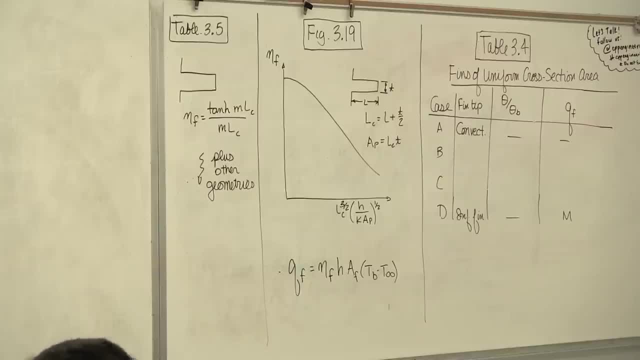 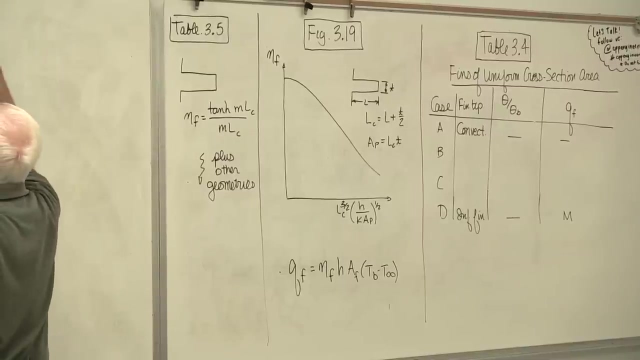 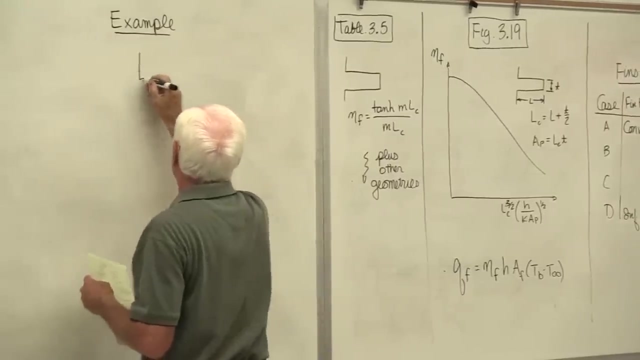 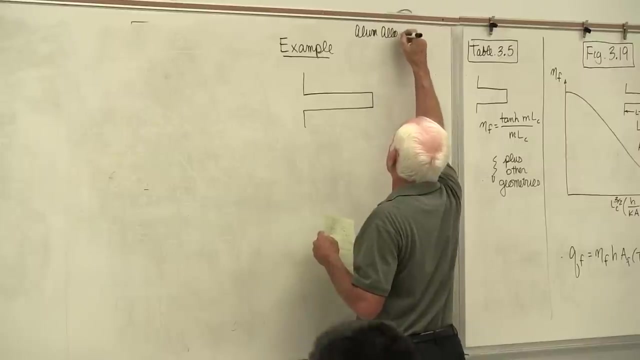 So let's start off. This isn't in the textbook, so All right, this is aluminum alloy fin. I think I'll put the picture over here. Okay, so here's our aluminum alloy fin. It's a 2024 aluminum alloy. 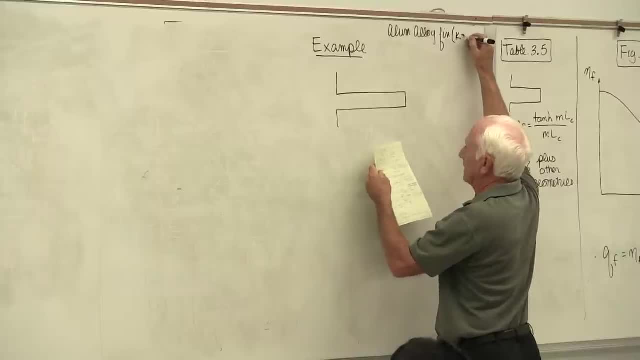 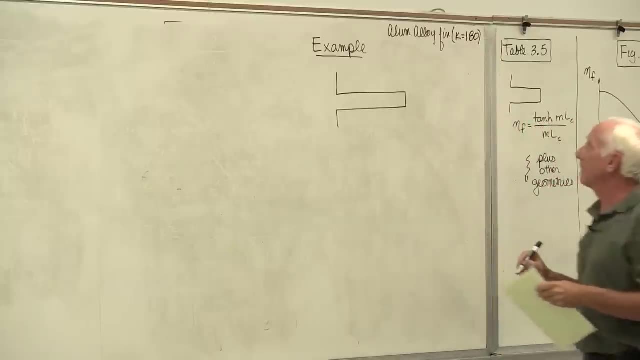 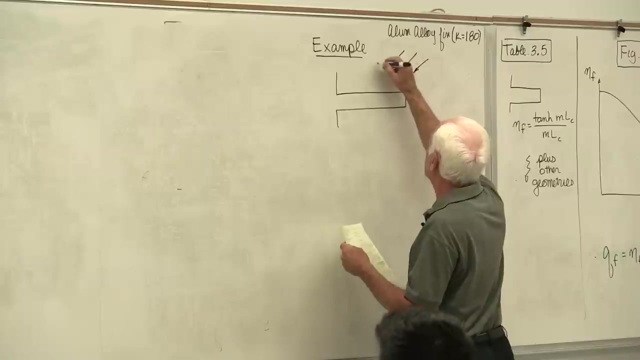 The K value in the back of the book for that fin is 180 watts per meter degree K. The fin is exposed to an airstream where the free stream temperature is given as 22 degrees. So that's a lot of air. So that's a lot of air. 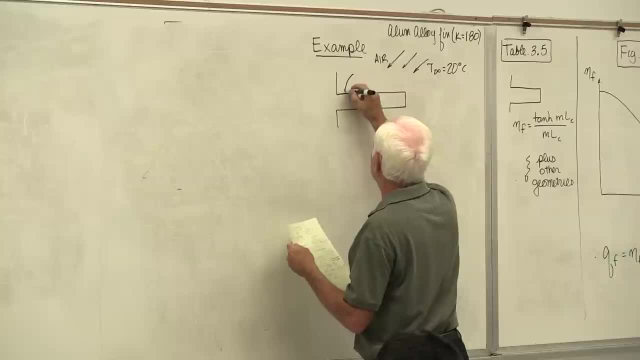 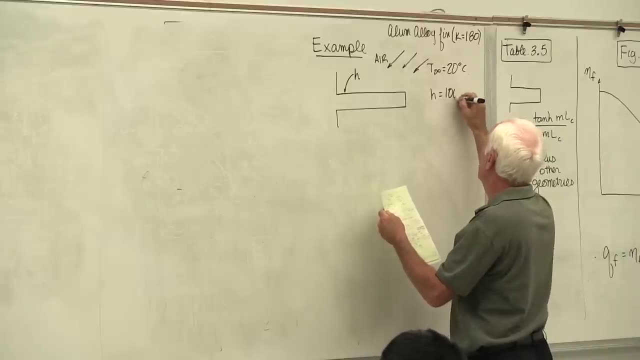 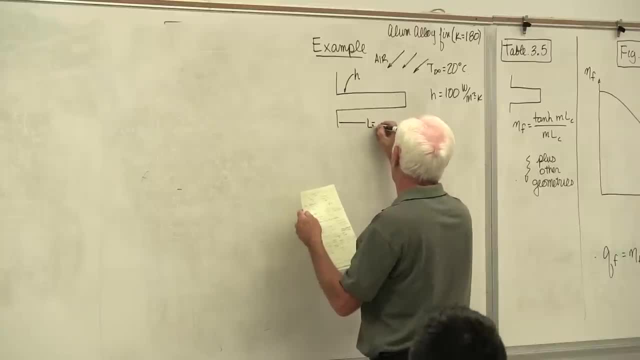 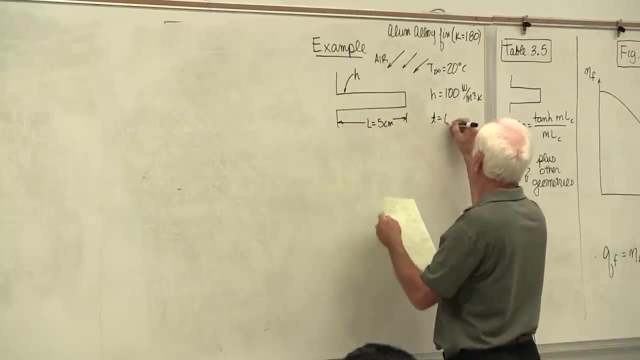 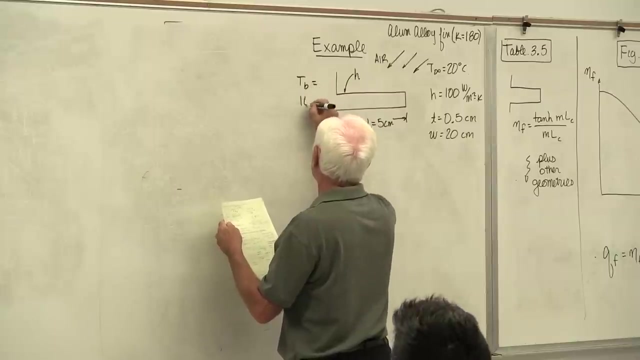 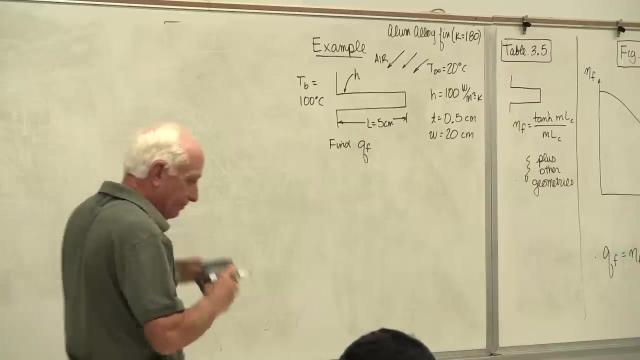 L is five centimeters, The fin thickness a half a centimeter And the fin width 20 centimeters. The base temperature is 100.. And we're supposed to find the fin heat rate, Find QF. Well, the first thing we want now, first of all, we're looking to say: well, what can we use? 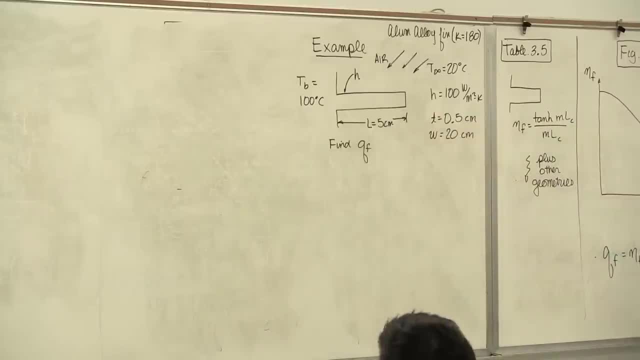 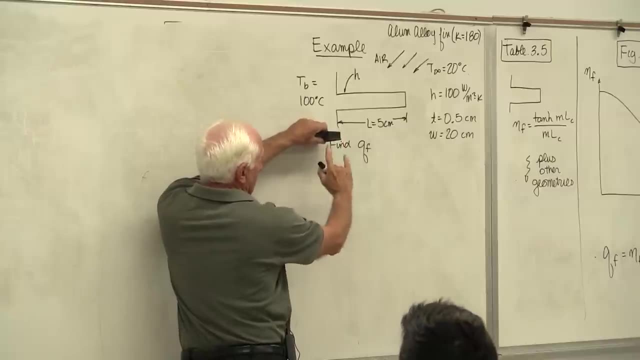 We're going to use a fin of uniform cross-section. Yep, This is just like my eraser: Five centimeters out from the blackboard. The width from here to here 20 centimeters. The thickness here to here five half a centimeter. 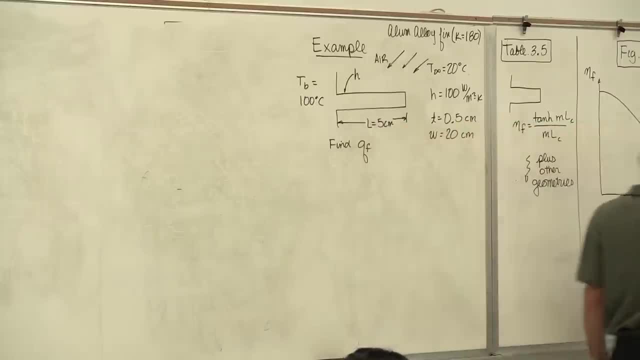 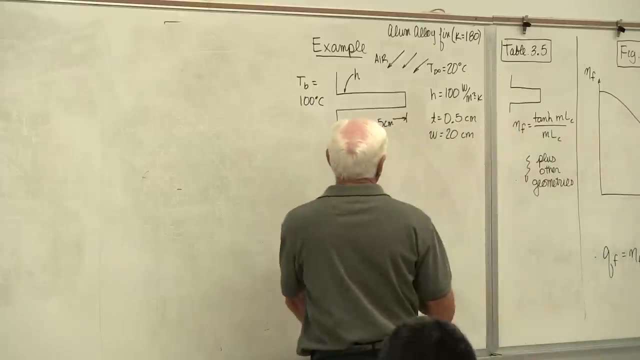 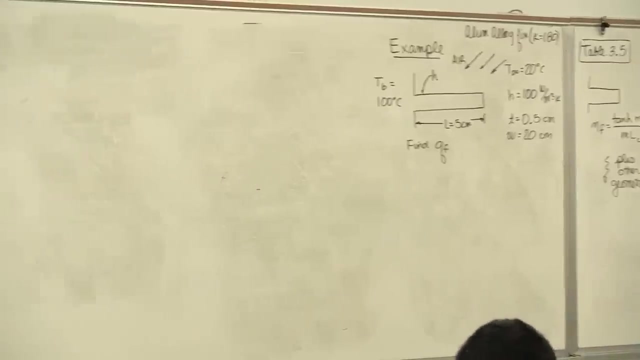 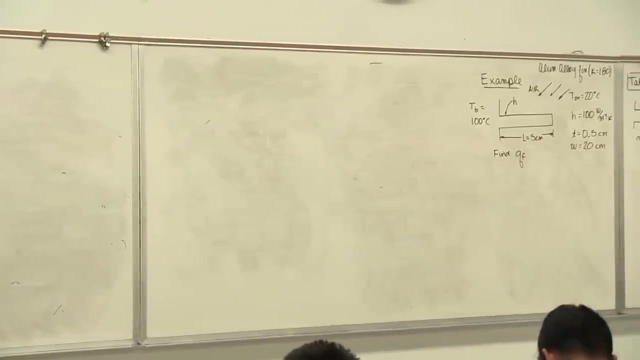 So, yep, that classifies as a table 3-4 application. So I want to use table 3-4.. And, uh, There's convection from the tip. But before I use that, because that equation has a lot of hyperbolic sines and cosines in it. 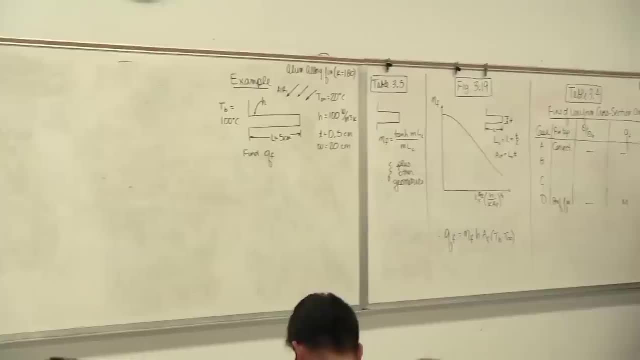 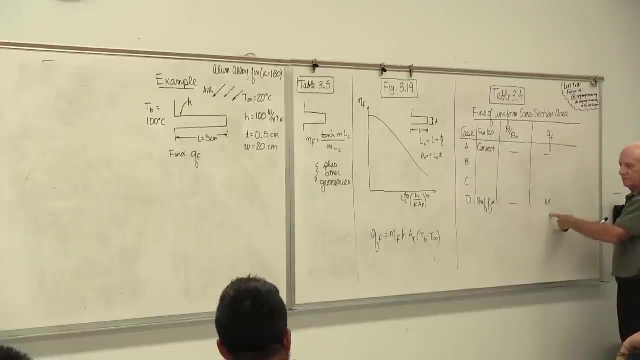 not a big deal, but it's rather lengthy. I'm going to try and take the easy way out. The easy way out is Q sub F, equal capital, capital M, if it can be modeled as an infinite fin. So I'm going to see if it can be modeled as an infinite fin. 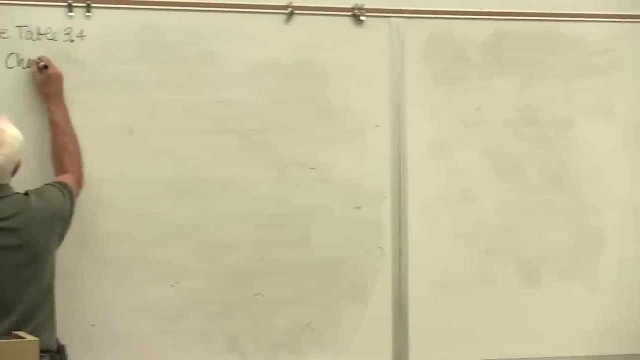 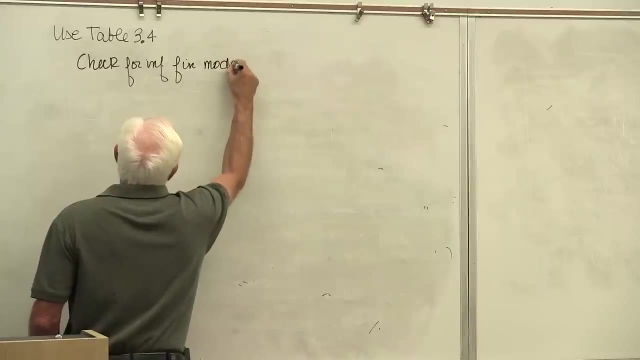 So I'll say: check for infinite fin. Okay, because if it is, I'll put the equation down here. If it is that capital M is really simple to get. All you do is take the square root of HPKAC multiplied by theta B. 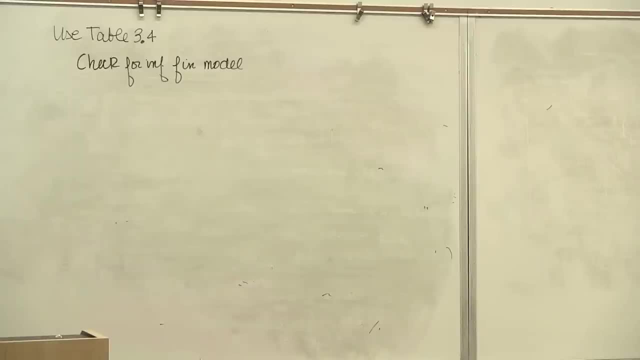 No hyperbolic sines, no hyperbolic cosines. That's it. And by the way, just to fill this in, little m is equal to the square root of HP over KAC. We'll need that, That little m right there. little m right there. 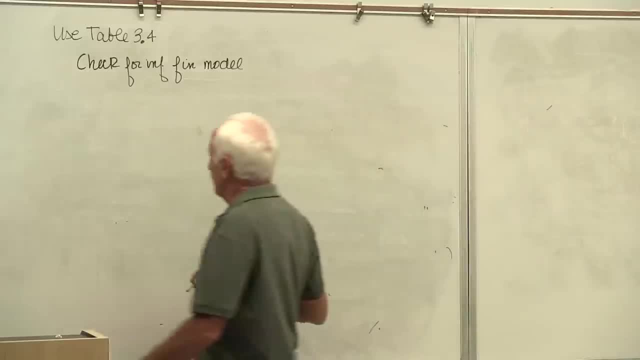 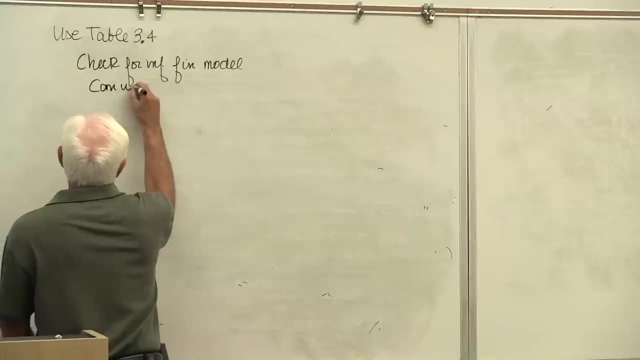 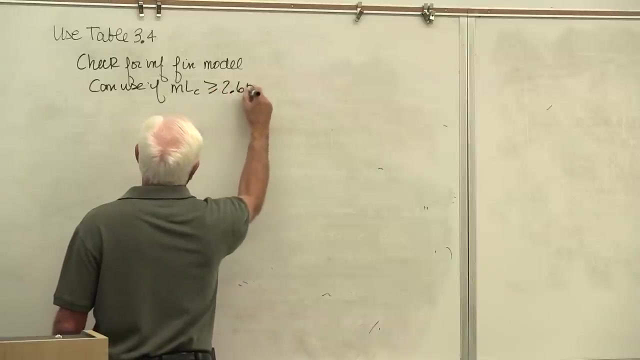 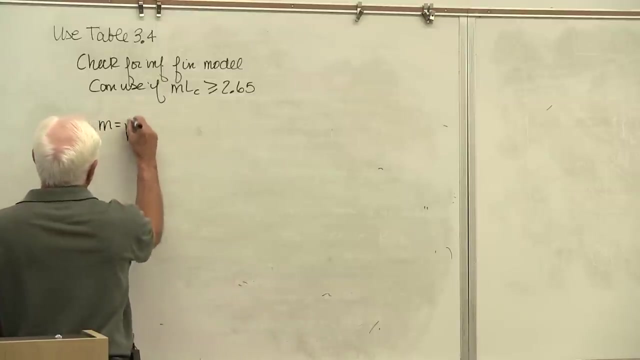 Okay, So we want to check that and see if can use if MLC is greater than or equal to 2.65.. Okay, So we'll get little m first. Square root of HP over KAC H is 100. 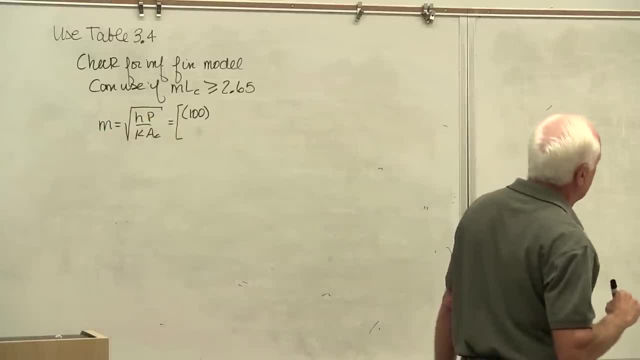 The perimeter: 2 times W plus 2 times C, 2 times 20 is 40.. 2 times T is 1.. 40 plus 1, 41 centimeters. 40 plus 1, 41 centimeters. 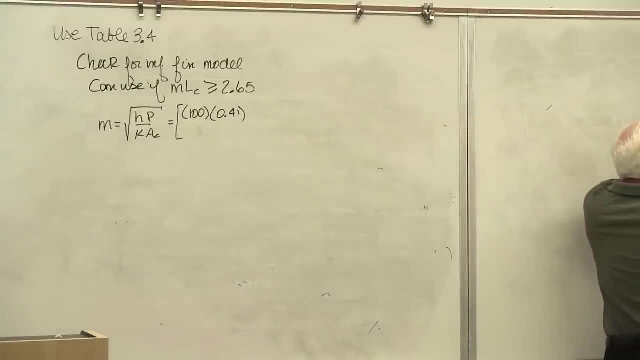 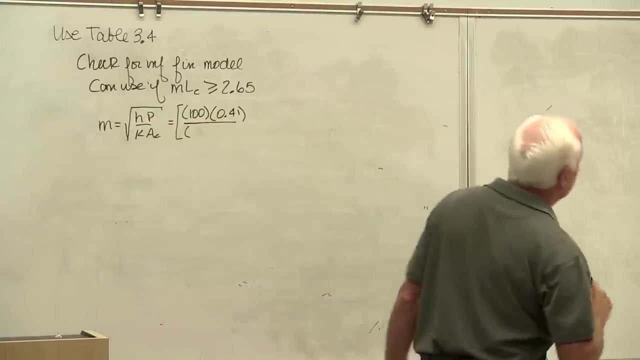 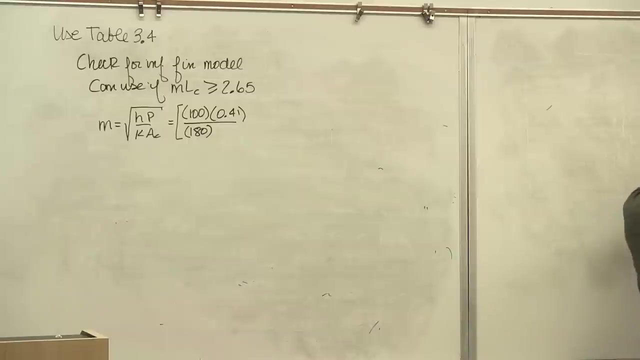 Here's the perimeter around it: T W, T, W, 2 times T plus W. Okay, Divided by K for aluminum alloy, 180.. Cross-sectional area: what you see, Thickness times W. Thickness times W. 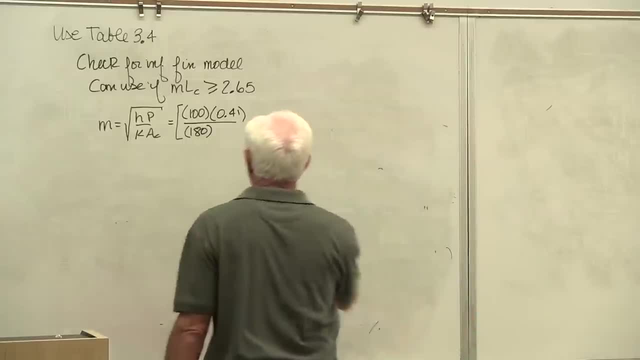 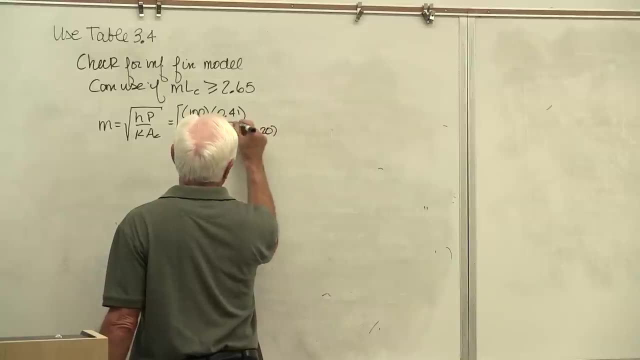 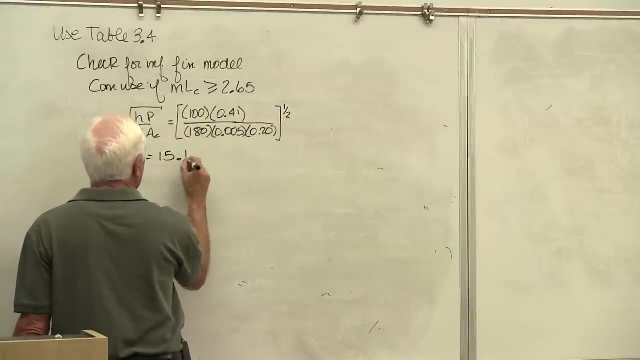 0.5 times 0.2.. Square root: Little m: 15.1.. MLC: 15.1.. Okay, L is 5 plus. Oh, I didn't put. Well, it's not? Yeah, thickness. 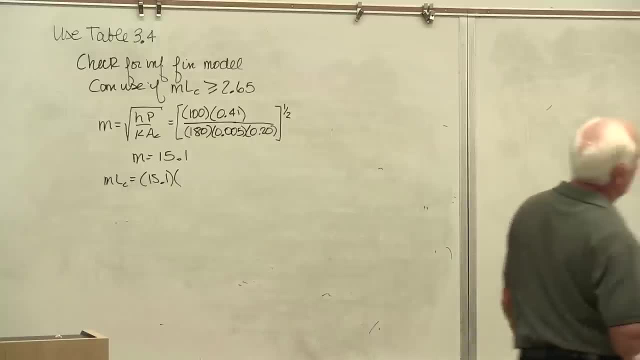 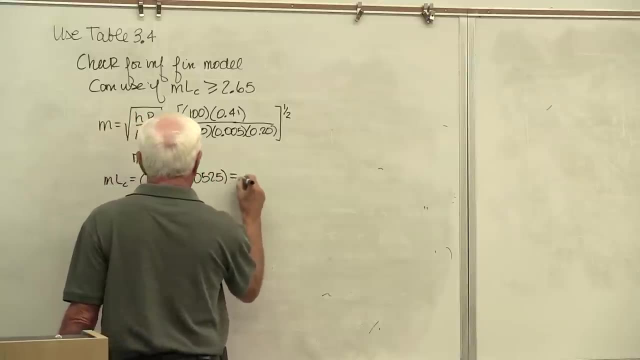 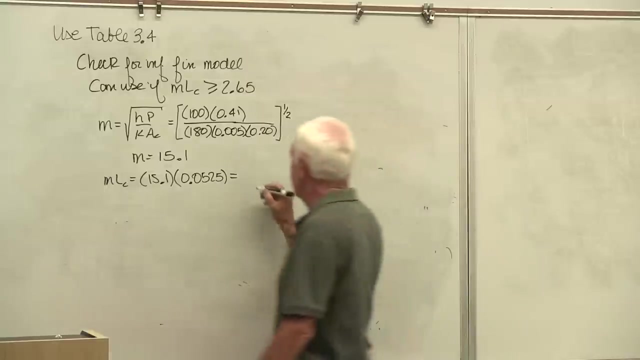 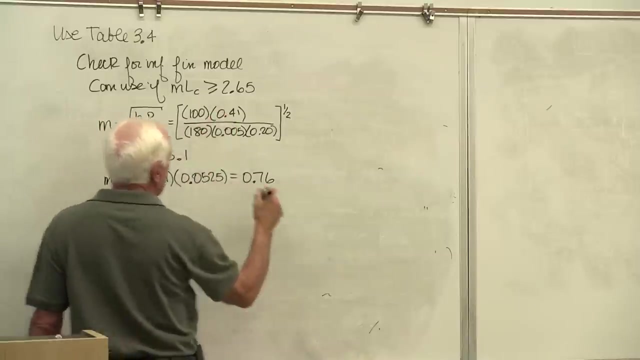 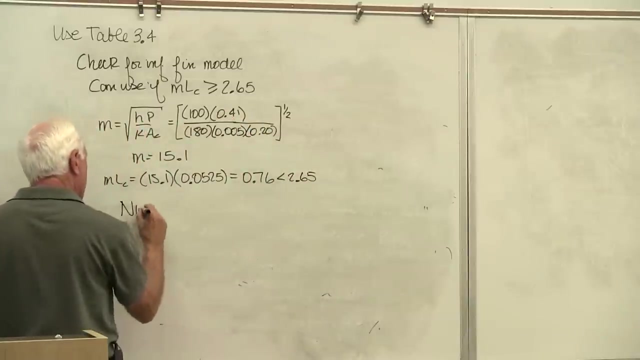 5 plus half of that guy: 0.25 centimeters, 525.. So that comes out to be 755.. Compare that to 2.65.. It's less than 2.65.. Not greater than no. cannot use case D. 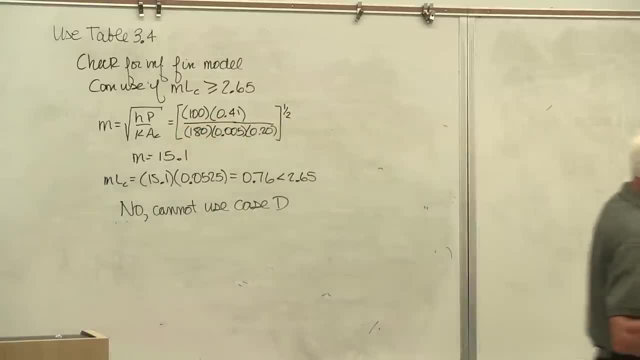 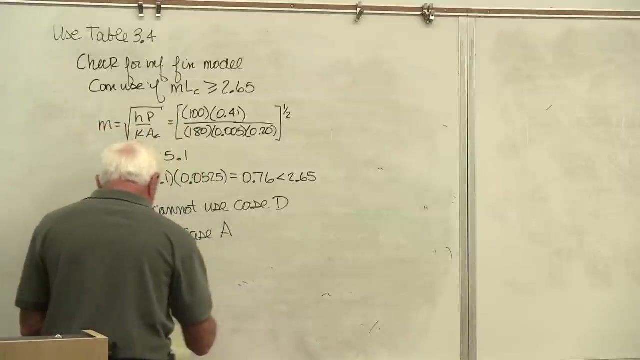 But it's worth a try because it makes life easier for you. If the answer is yes, there's the answer: capital M right down there: capital M. So we have to use case A. Okay, case A- QF. 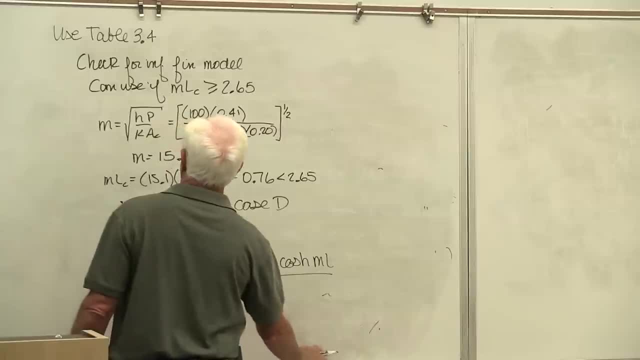 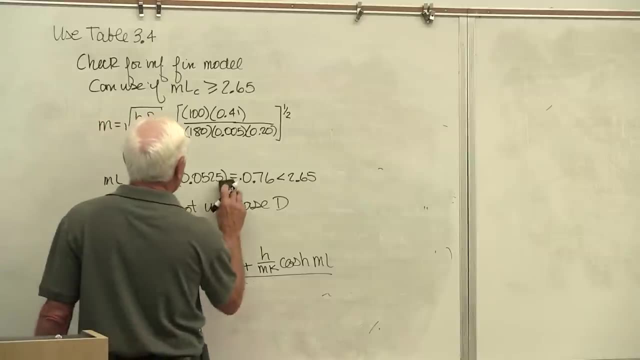 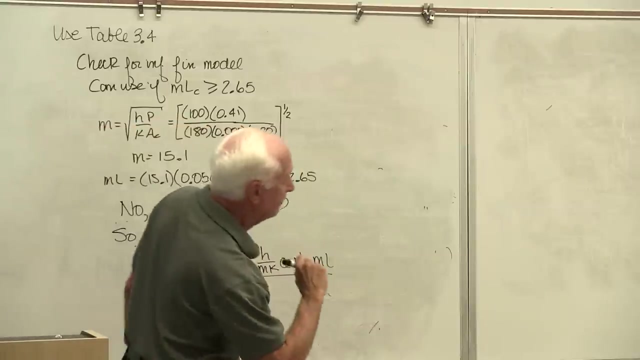 And, by the way, don't put that C in there, Not for table law 3, 4.. No, This is 5, 0.. That's table 3,, 5, and figure 319.. Hyperbola. 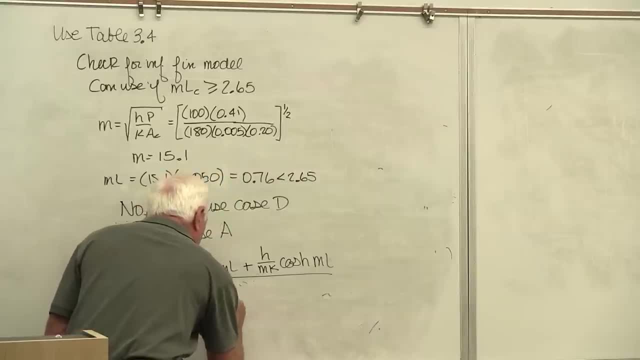 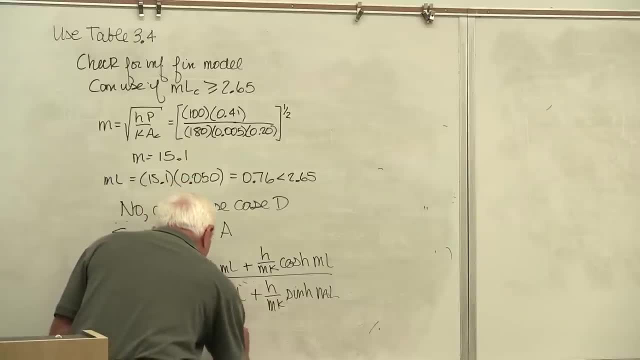 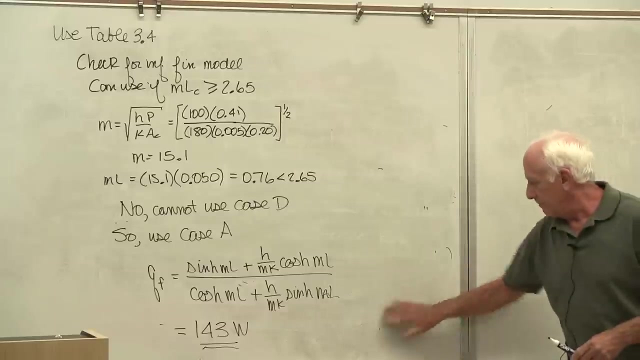 Here, There. This is here, Here Here. Now you got the choice: Use your handheld for the hyperbolic functions or table B1, for the hyperbolic functions in the back of the book. Okay, we plug the numbers in and we end up with 143 watts. 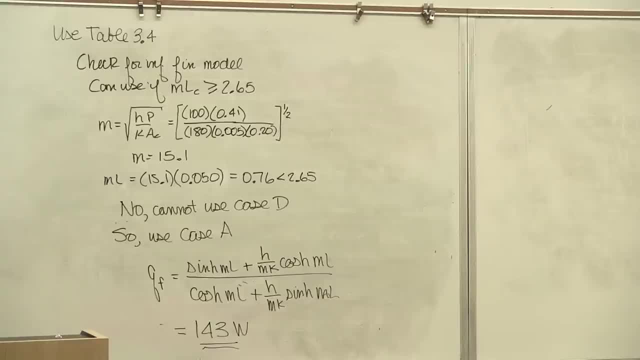 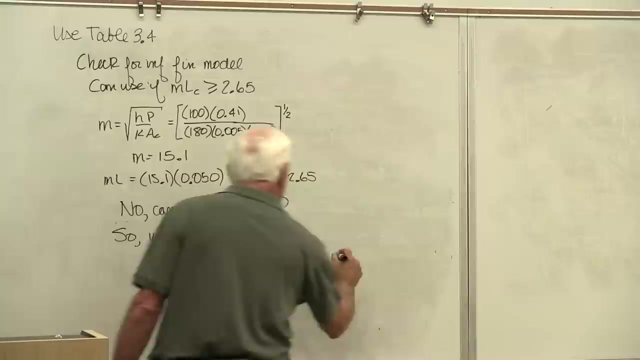 Okay. Oh, by the way, This is the power, This is this. Oh, by the way, one other thing, be real careful there. that guy in the book, table 3-4, there is- is multiplied by an M out in front here. there's a capital M out here, so I'll put the capital M there. I'll. 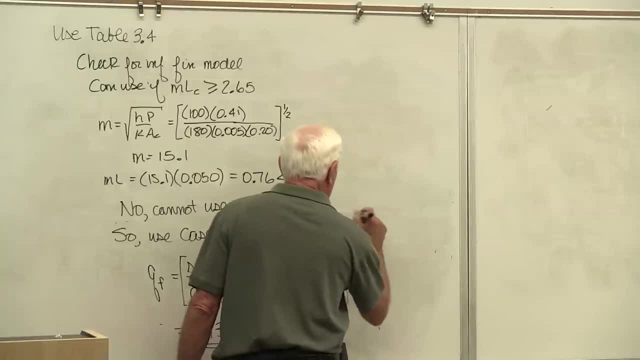 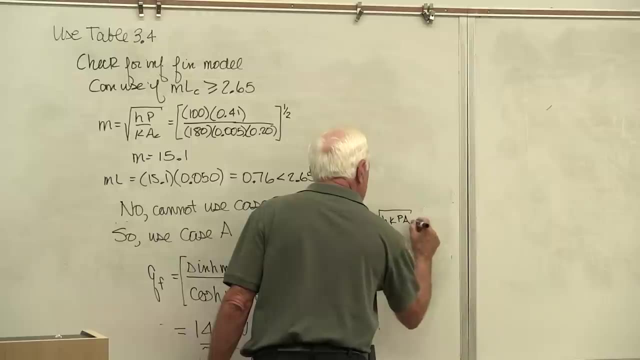 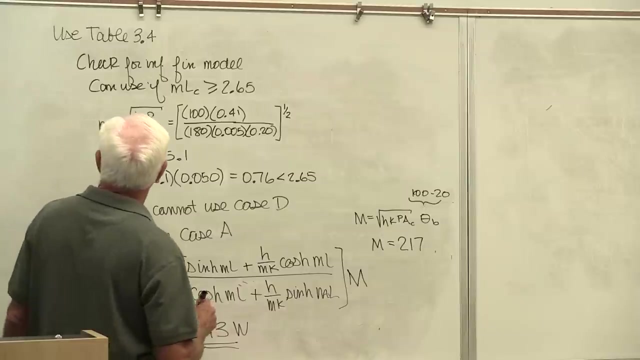 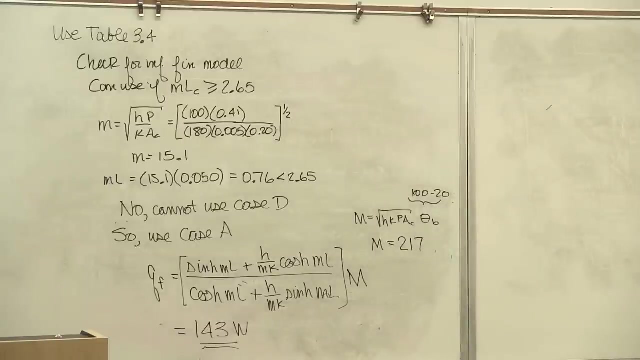 capital M: square root HPKAC, theta B. theta B is 100 minus 20, capital M: if you run the numbers through, 217, okay, All right. now we can say, well, okay, that worked out pretty good, but why not try figure 319, there's our rectangular fin. looks like that picture right there. okay, we'll use figure 319.. 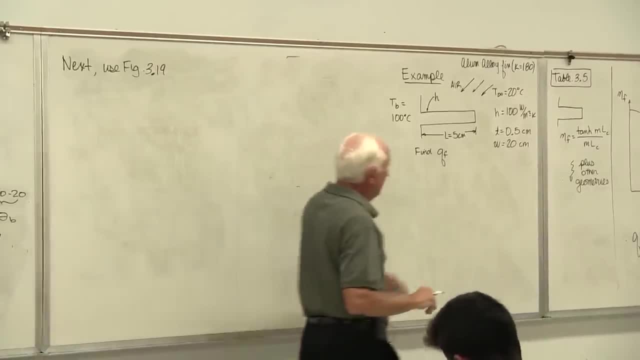 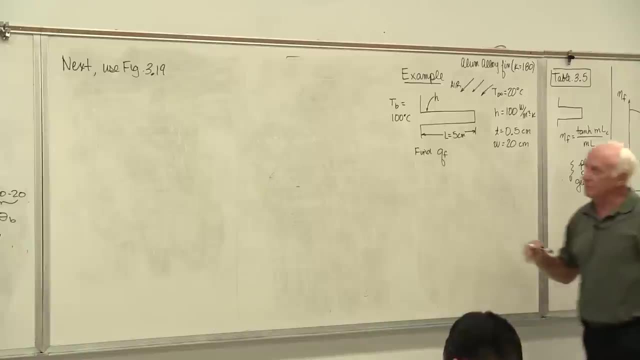 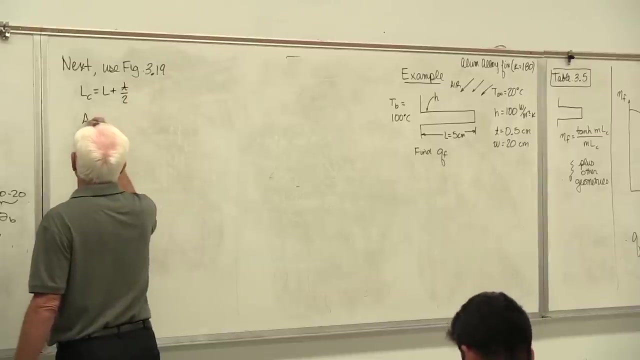 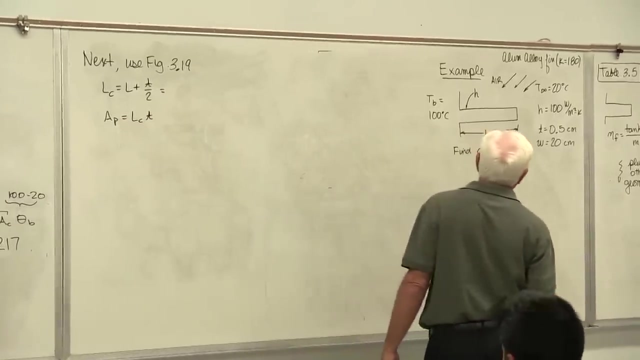 Okay, to use figure 319, here's what it says. if you want to use this figure, you've got to use LC. LC is L plus T over 2, A sub P LC times T. All right, so we've got. L is 5 centimeters. 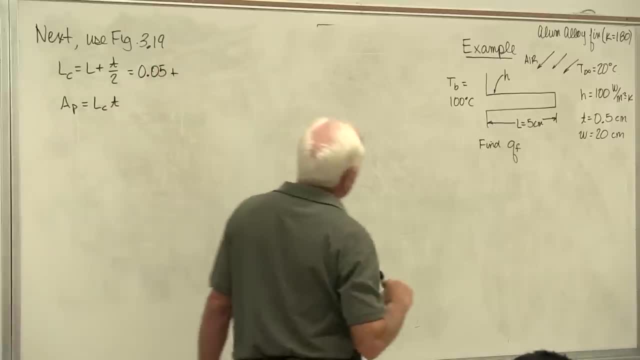 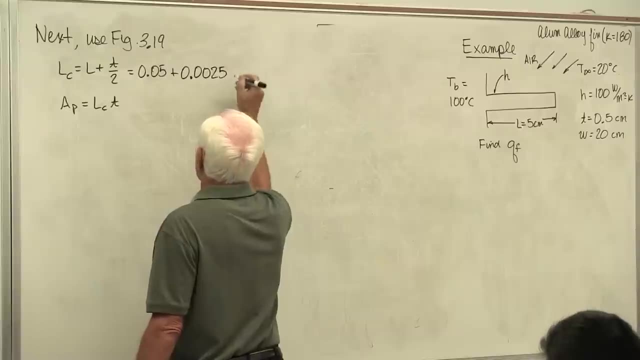 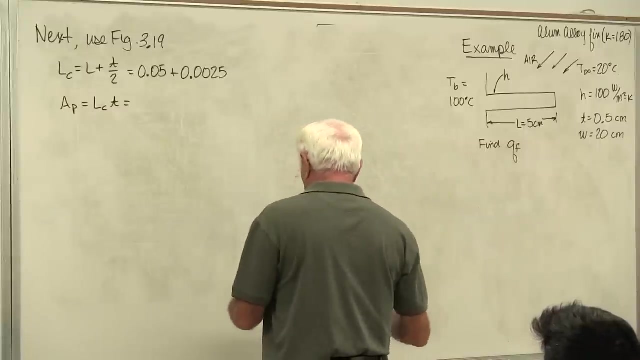 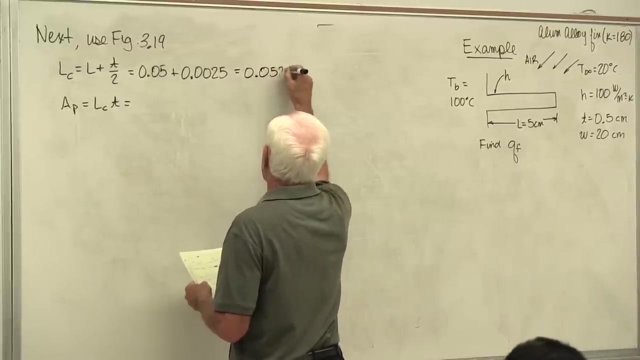 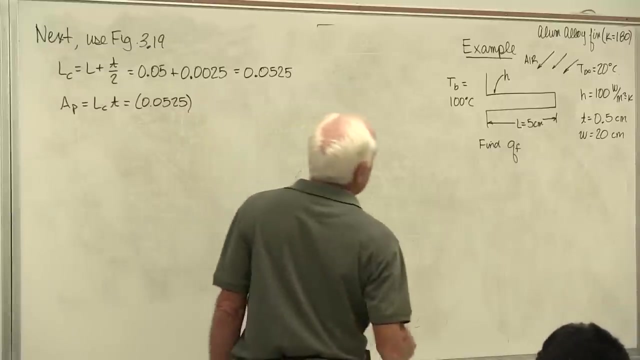 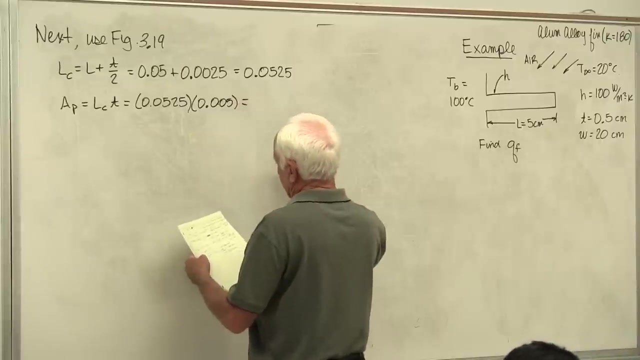 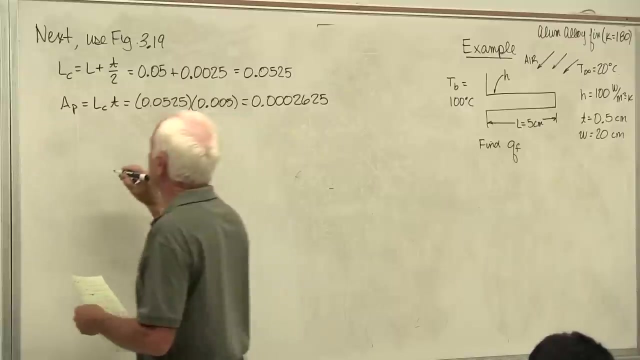 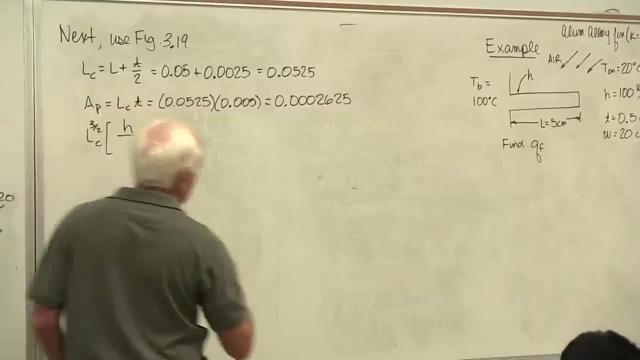 Half of T. T is a half a centimeter and our L sub C. then there it is: 0, 5, 2, 5,, 0, 5,, 2, 5.. T: half a centimeter, 3 zeros, 2, 6,, 2, 5,. the x-axis parameter, KAP, square root. 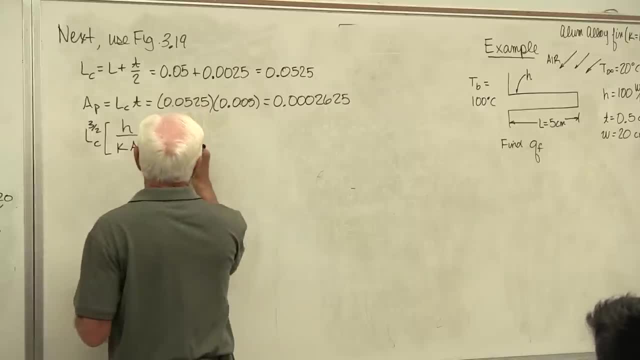 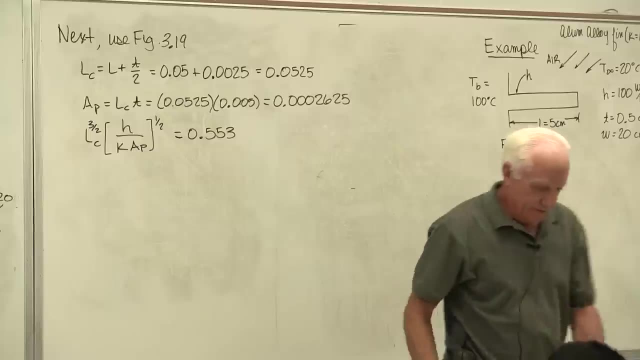 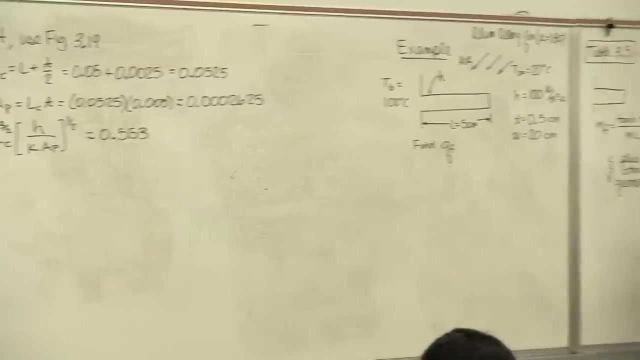 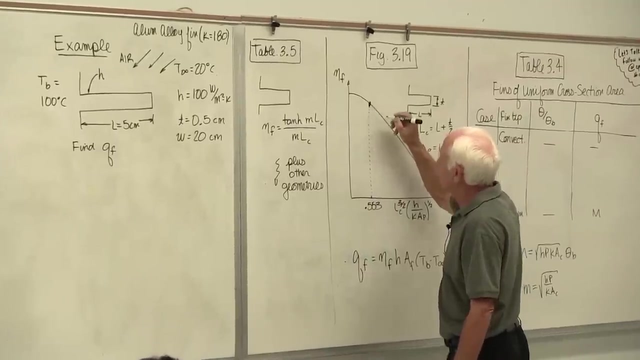 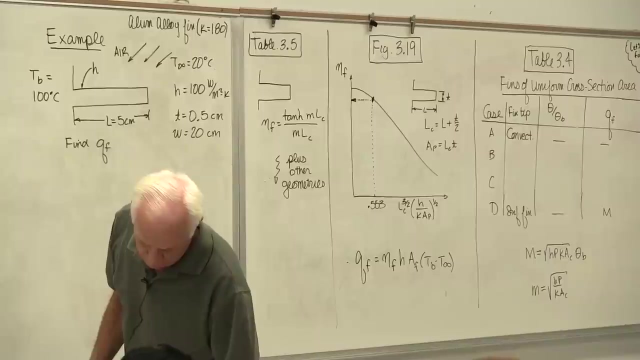 5,, 5,, 3.. Okay, so we go to the graph, the x-axis parameter value: 5,, 5,, 3.. We go up vertically to the line For the rectangular fin, we intersect, go across horizontally and it's somewhere between 0.82 and 0.83.. 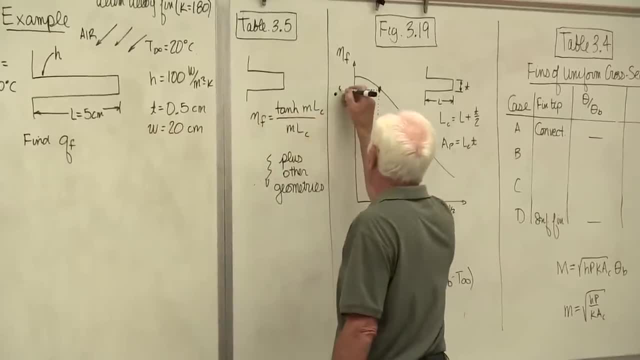 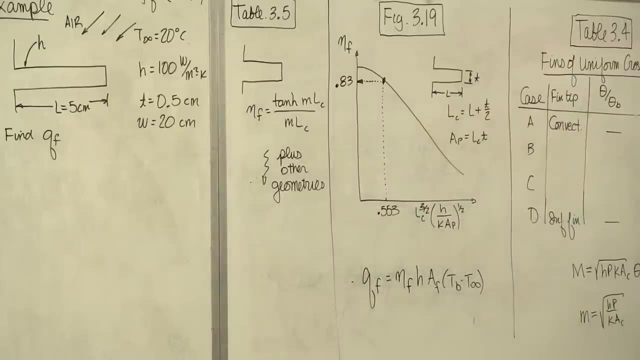 I took 0.83.. Well, you can read the graph reasonably accurate. It definitely is not 0.80. And it sure isn't 0.85, if you look at it carefully enough. So I took one in the middle like 8, 3, 8, 2 would be fine. 8, 2 or 8, 3.. 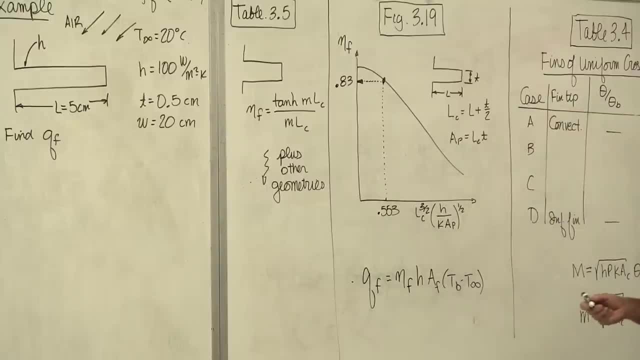 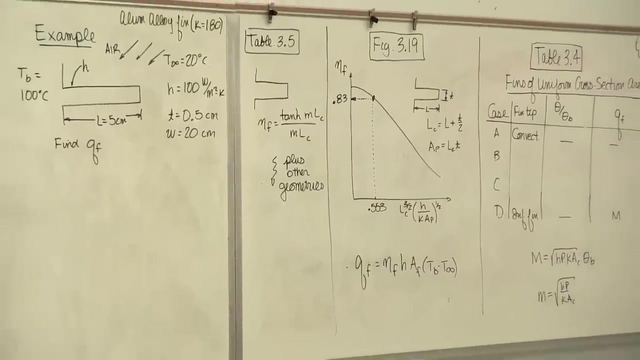 But you can get pretty close, close to 1%, 2% reading error. That's really good. Okay, now there's the equation. So QF A to F H A, fin T base minus T infinity. 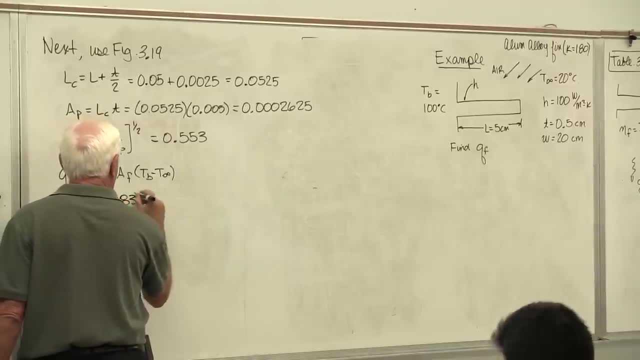 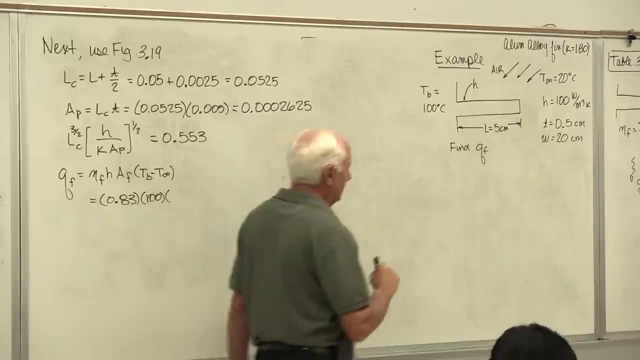 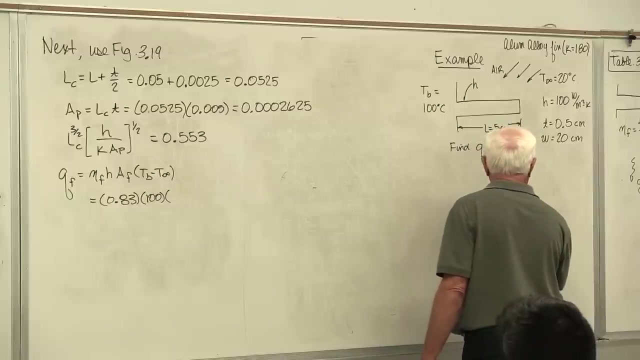 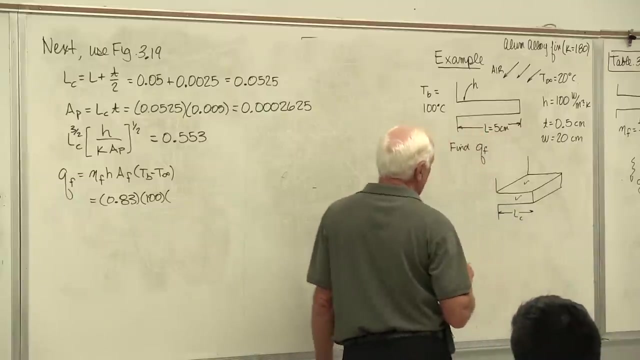 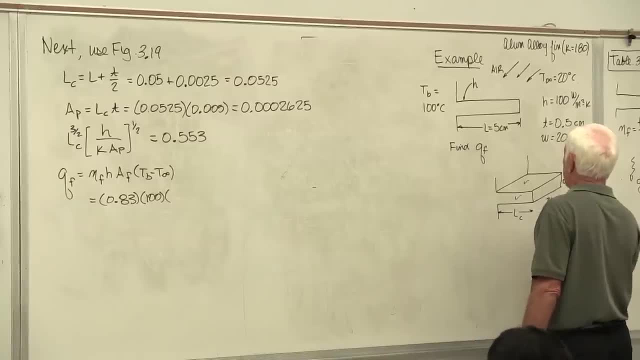 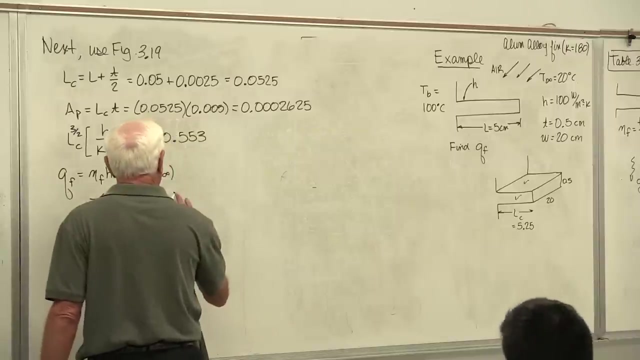 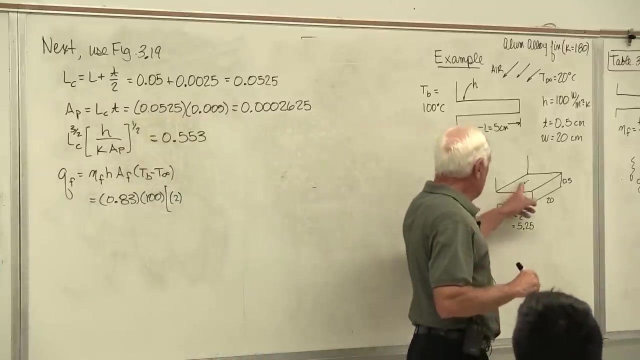 20, 1⁄2, L sub c 5.25.. All in centimeters. All right, let's do the top first. There's a top and a bottom too. Top is 20 by 525.. 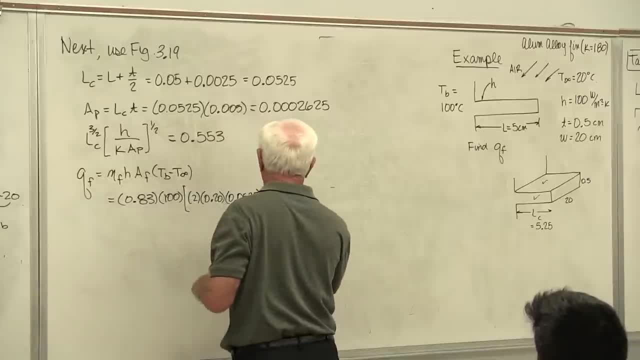 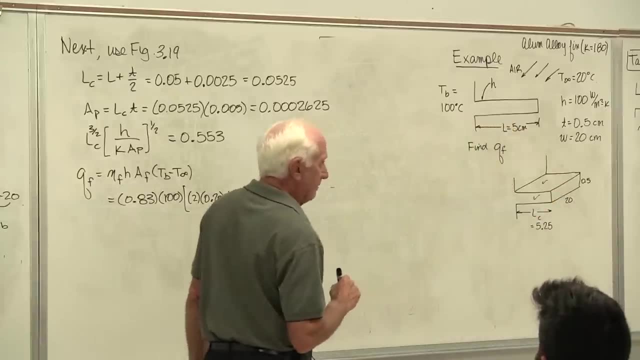 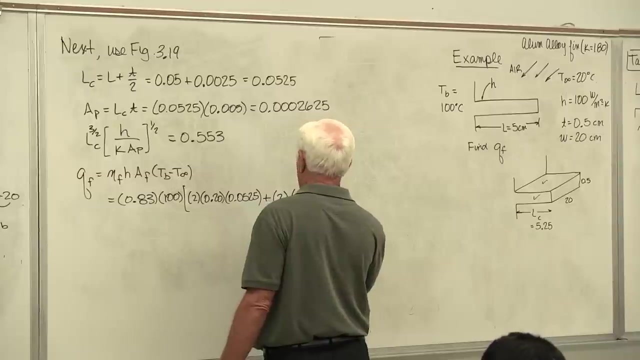 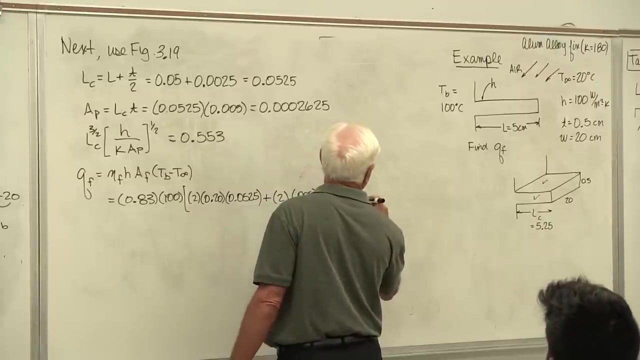 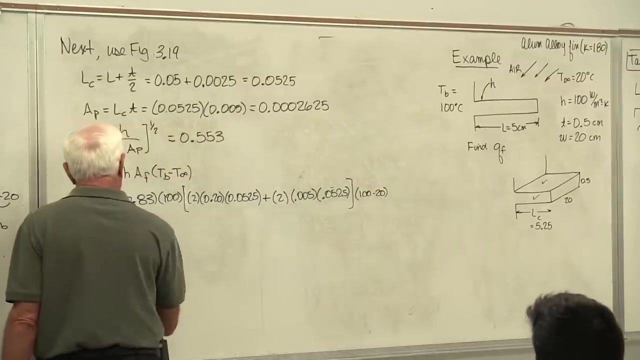 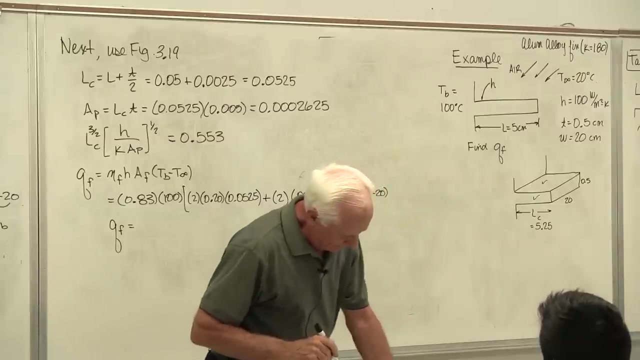 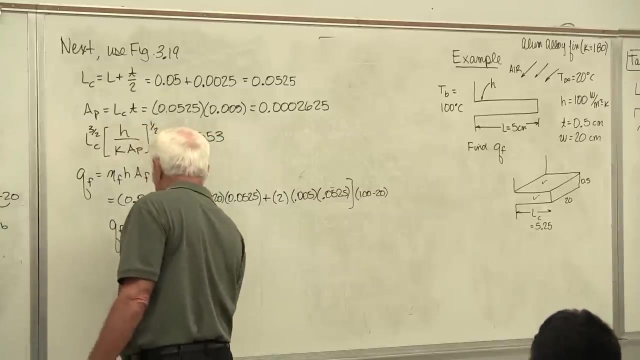 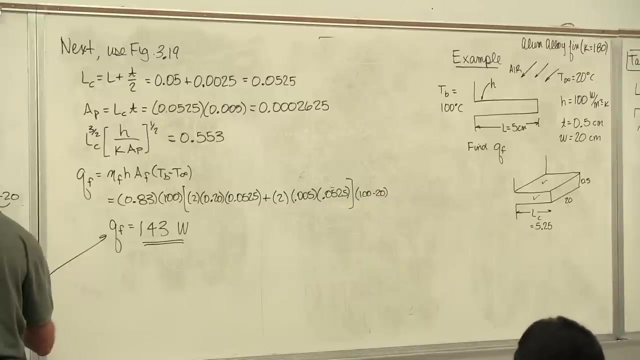 Yep Plus. there is a front side and a back side: 525 and 05.. Times the temperature difference: 100 minus 20.. Yeah, same answer. It's going to be close. It might be off a little bit, but this time it just happened. 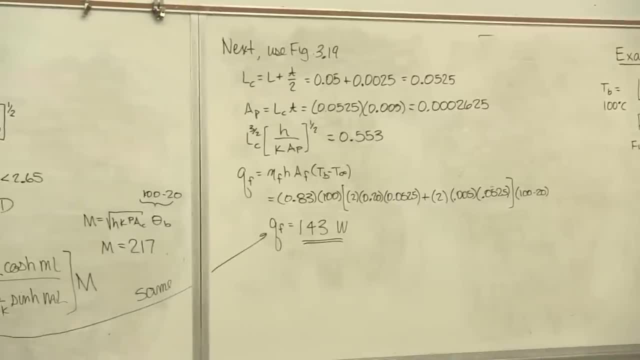 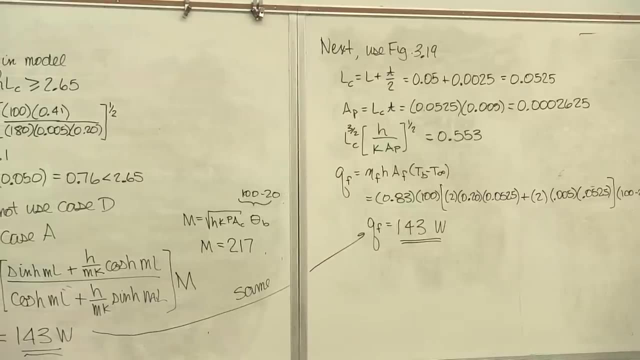 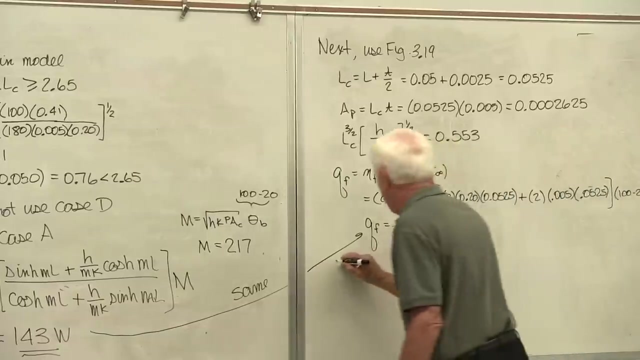 The number is crunched out, We're at the same answer. So whether you use table 3-4 or whether you use figure 3-19, you're going to get the same answer. Okay, you say: well, if I use that, I'll take it one more step. 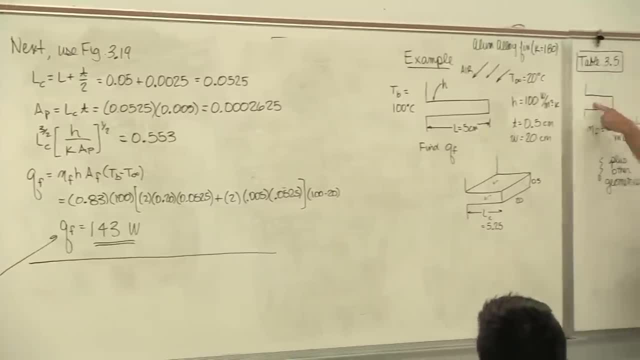 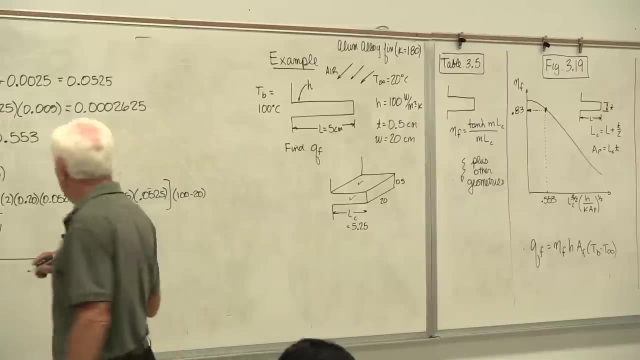 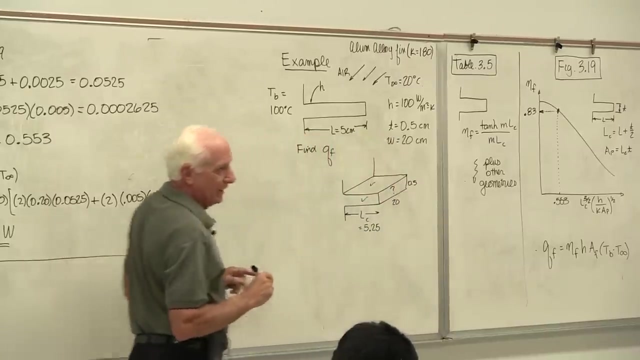 I'm going to try and use table 3-5, because that picture right there looks just like that picture right there. Yeah, you got it. That's it right there. Now, just to remind you, we didn't include the convection on the tip. 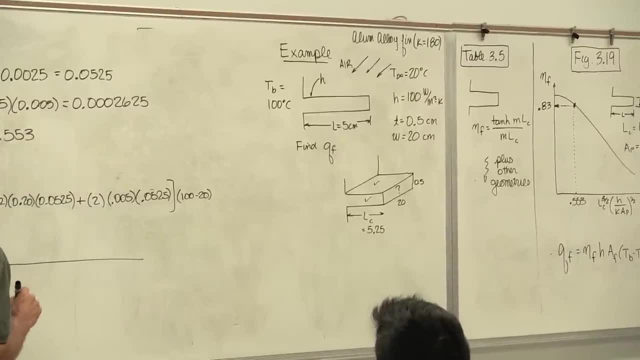 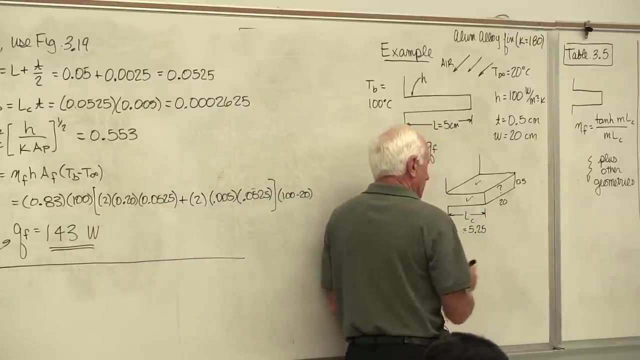 Why? Because everywhere, in every equation, we used L sub C. And what does L sub C mean? It means you made the fin a little bit longer, so there's no heat transfer. Assume the tip of the fin. now the heat transfer occurs around the top, bottom, front back. 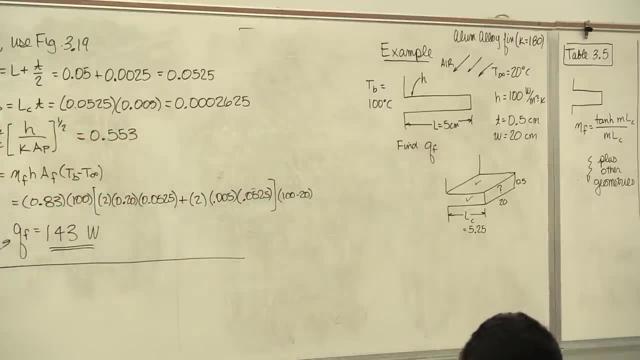 Can you hand your hand up? That was it, Okay, okay, Yeah, Because we used L sub C Whenever you go to figure 19,. we use L sub C. If we go to table 3-5, we use L sub C. 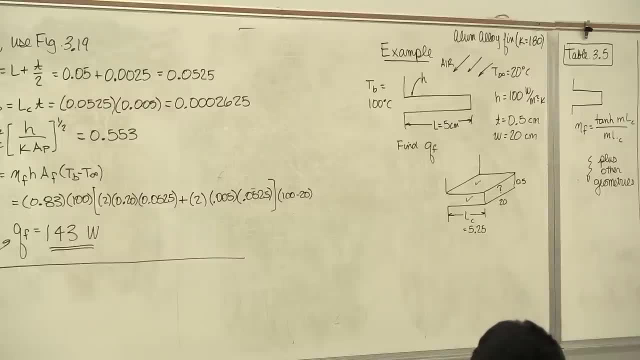 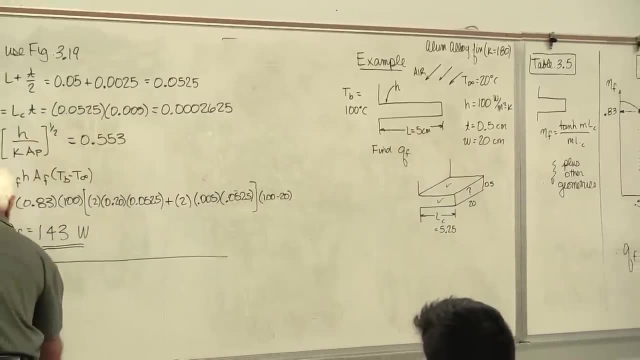 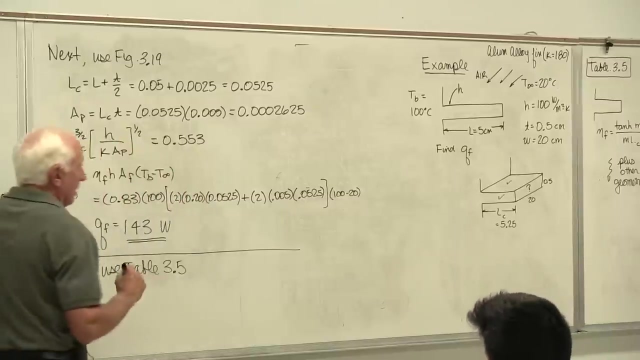 If we go to table 3-4, we don't use L sub C, L sub C, Okay. Next use table 3-5. You're going to find table 3-5. There, it is right there, okay. 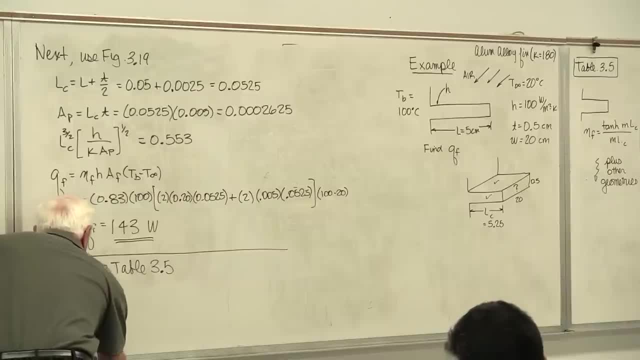 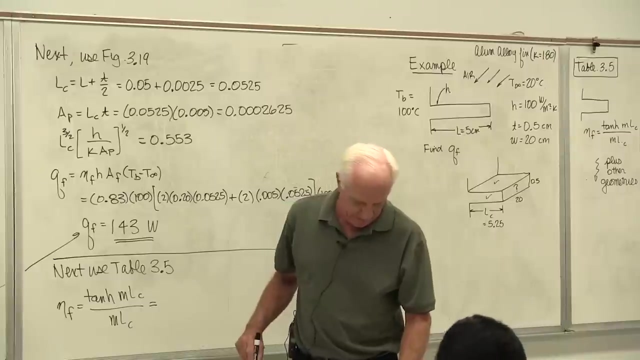 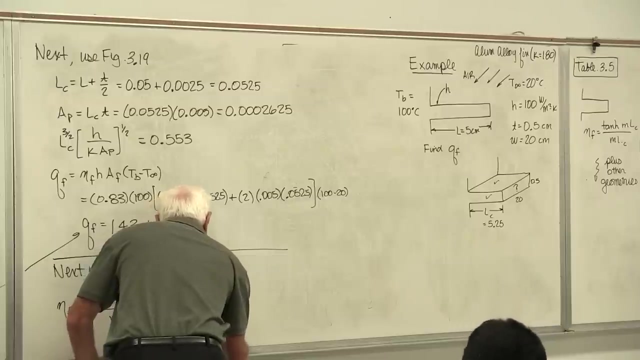 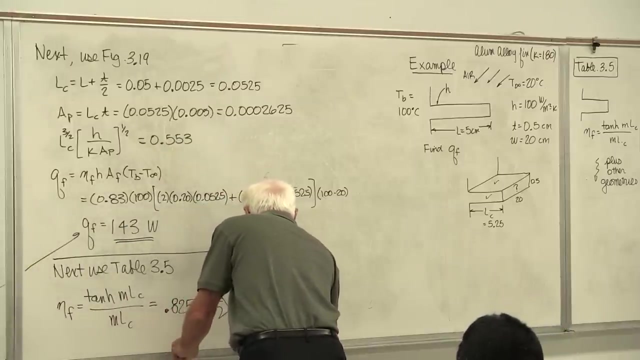 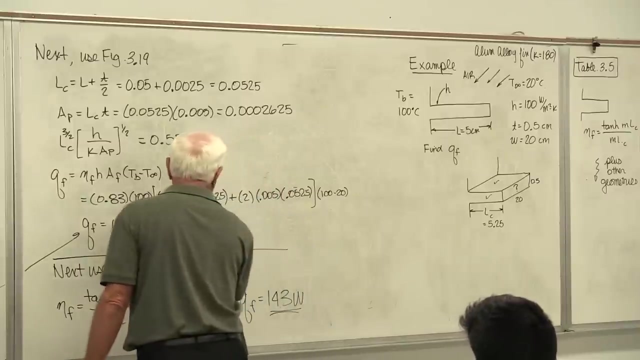 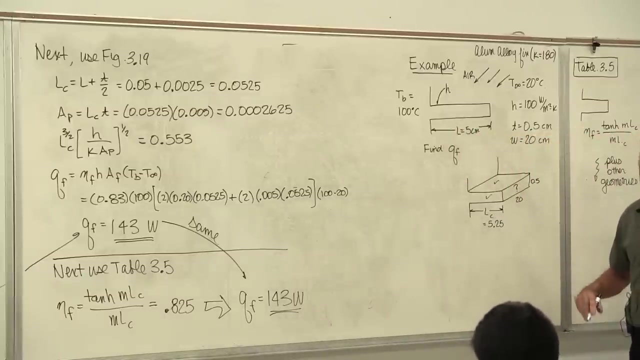 Fin efficiency. fin efficiency: hyperbolic tangent MLC divided by MLC, I got on this one 0.25.. If you round it off, I still get QF equal 143 watts. If you're doing a computer code, you can't put the graph in there. 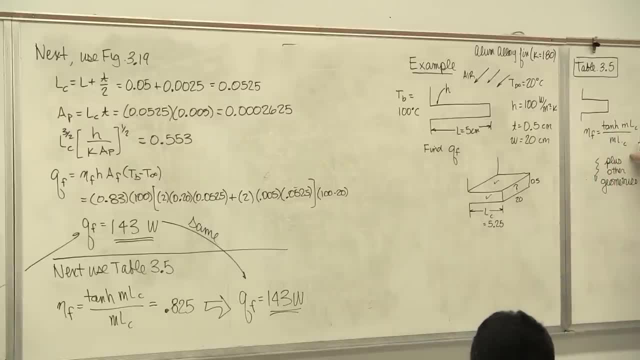 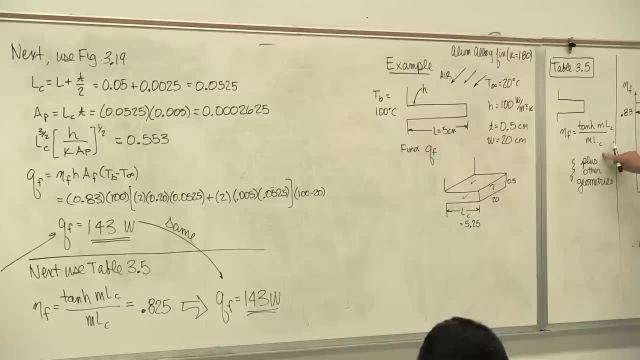 So a computer code, you'd use table 3-5. But for homework or an exam, your choice. Either read this guy or use this guy, It doesn't matter. Take your choice, Okay, it doesn't matter. then Three ways to do it. 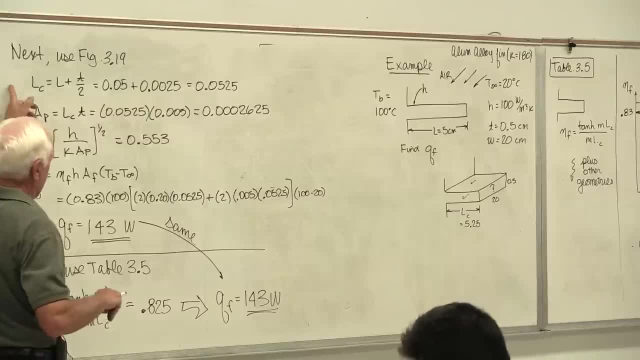 Table 3-4, 143 watts. Figure 3-19, 143 watts. Table 3-5, 143 watts. Doesn't make any difference. Okay, We talked about these other guys on here. We talked about case B, which is an adiabatic fin tip. 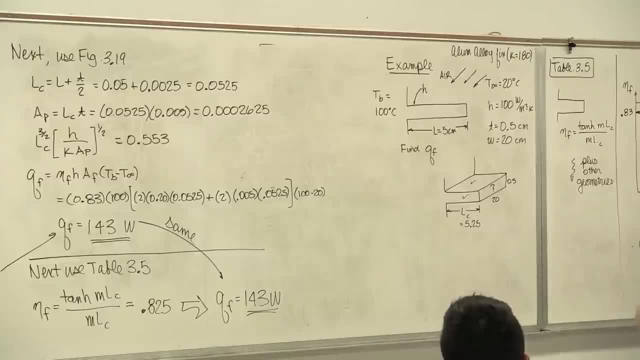 Nobody makes fins where they put insulators on the tip of the fin. The purpose is not to stop heat transfer, It's to cause heat transfer. So nobody wants to insulate the tip of a fin. That's nonsensical. But we talked about that, about the fin between two walls: 100 degrees C here. 100 degrees C here. 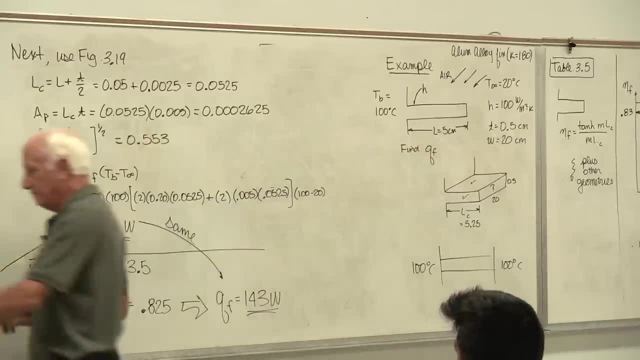 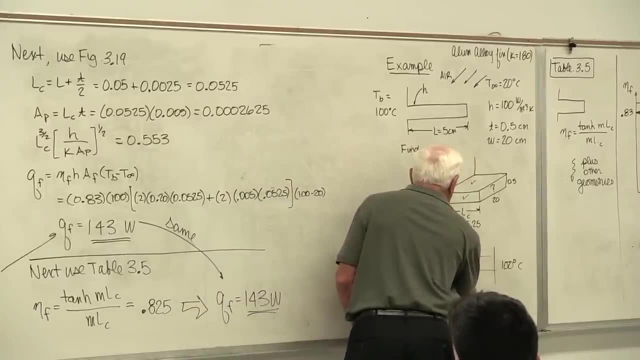 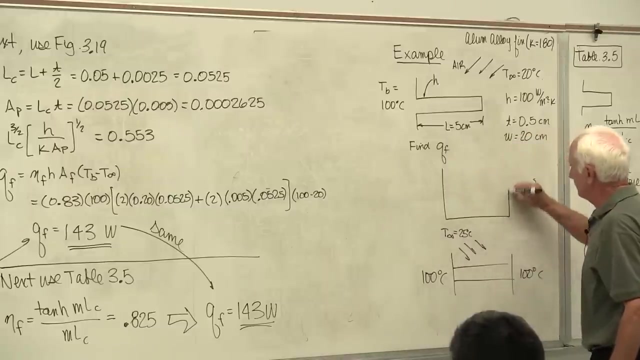 And if you want to plot the temperature- let's say the air is blowing over the fin at 25 degrees C- And if you want to plot the temperature from zero, out here as a function of x, and this is L, 0, L over 2, L. 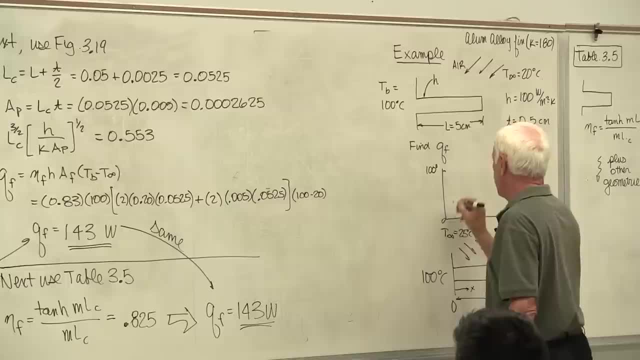 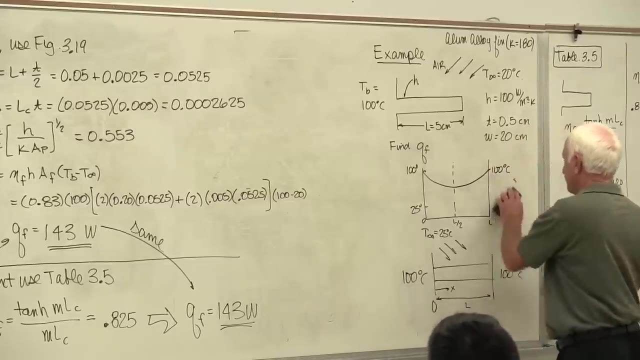 Here is the base temperature is 100.. The air is at a temperature of 25.. Here's the middle. Here's how the fin temperature looks. You say, wow, That's interesting. Look at the middle of that. You know what that middle looks like. 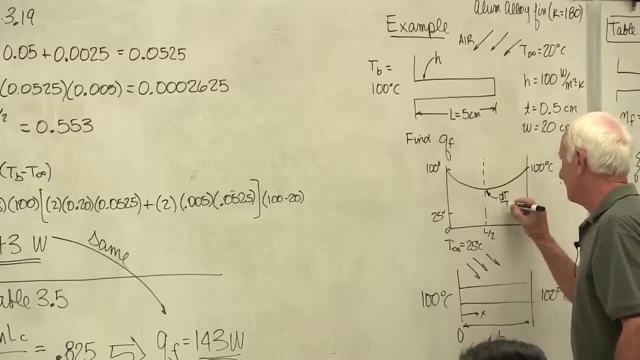 It looks like the slope is zero. Well, of course it's zero. DTDX there is zero. And if the slope looks like it's zero, that means it's behaving as if it were adiabatic. And if that's the case, I can use case B. 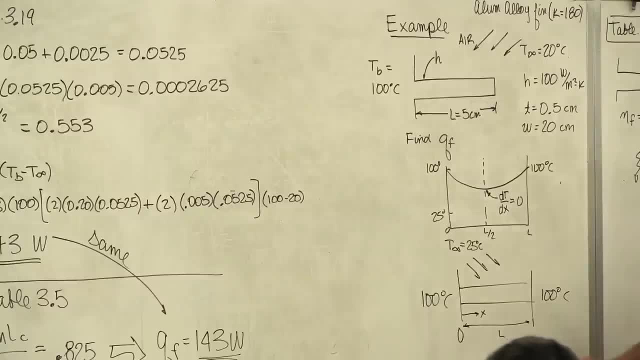 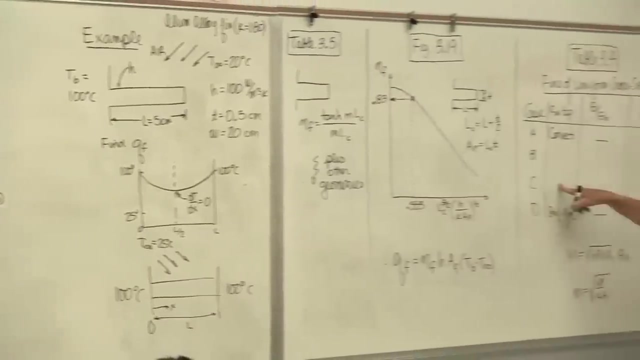 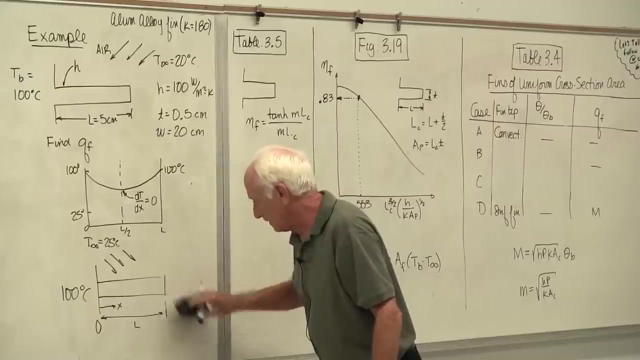 Yep, you got it, So now you solve it. Half the fin, case B, Both sides, two times case B. Find Q sub F from here. Multiply it by 2.. A prescribed temperature. Okay, prescribed temperature. Maybe somebody tells you that this side of the fin is at right. here the temperature is 75 degrees C. 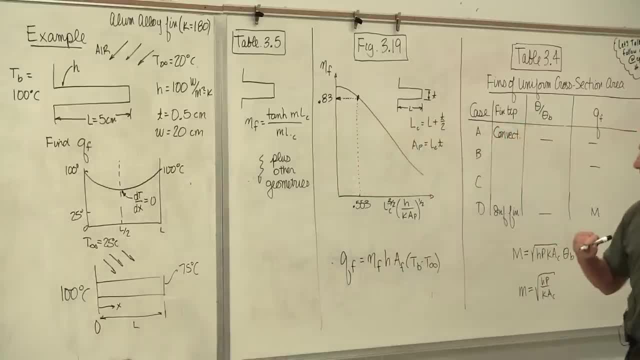 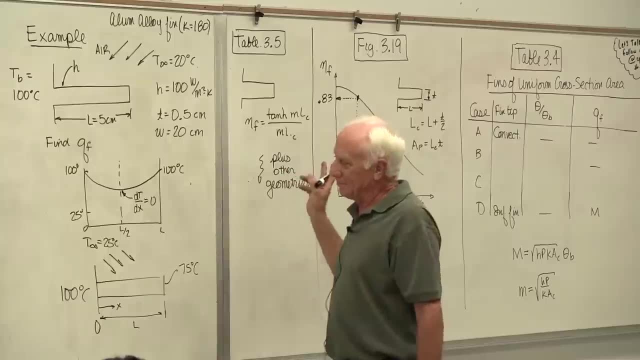 Okay, The base is 100.. The air is 25.. That is a case. That's the seat that you use, All right. So just so you know what that table 3-4 is going to give you. Now I'm going to take another example. 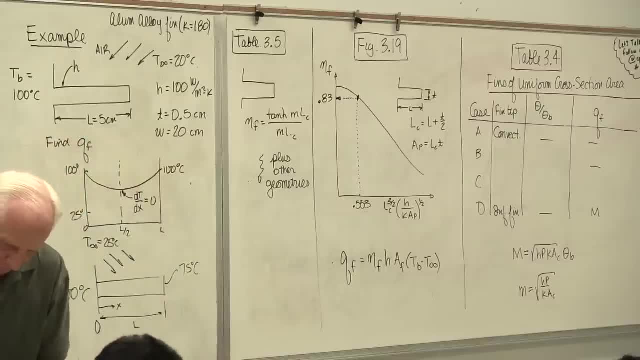 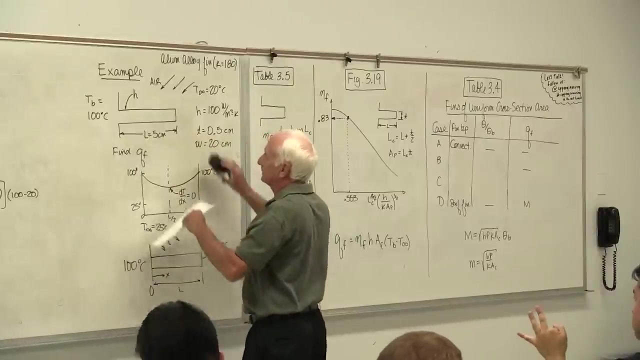 And this one is going to be a triangular fin. All right, Let's see. I'll put the picture right here. Example: Change the geometry. It's going to be triangular, It's going to be a triangle. It's going to be a triangle. 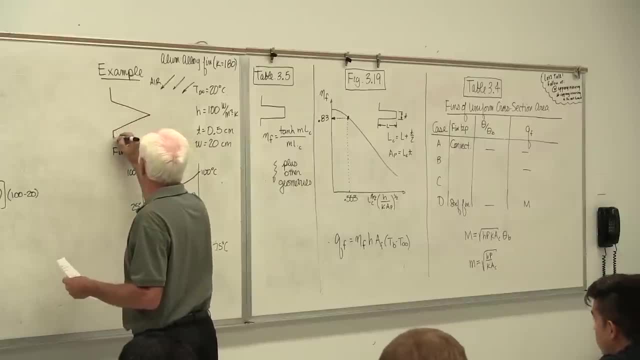 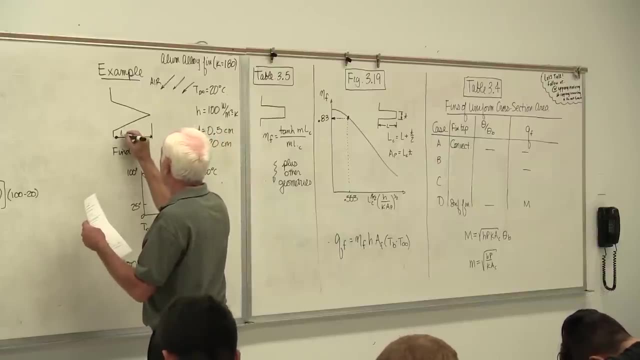 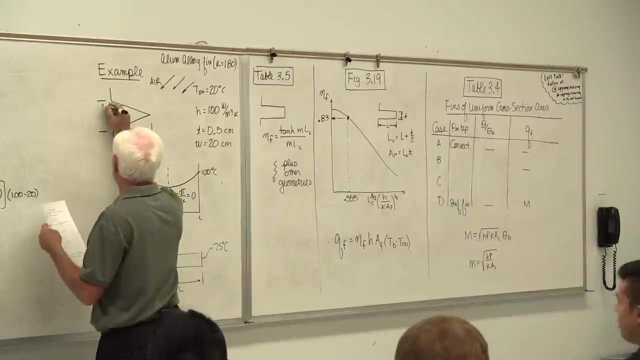 It's going to be a triangle. Okay, L distance. Okay, The L distance here: Six millimeters. The thickness of the fin: Two millimeters. Two millimeters. The base temperature of the fin given: 250.. The air temperature is 20.. 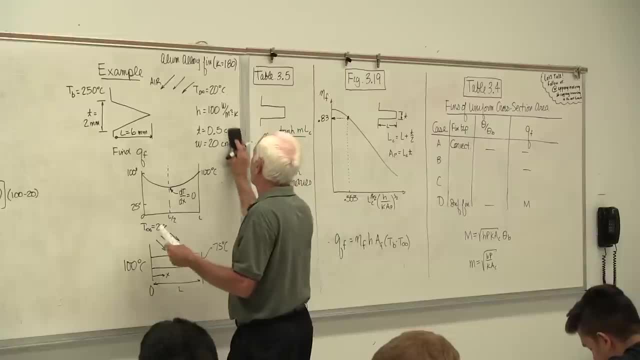 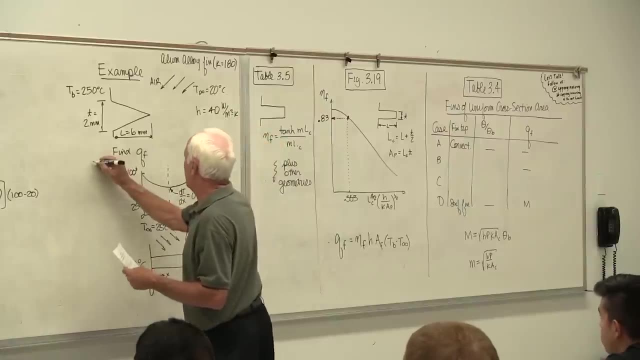 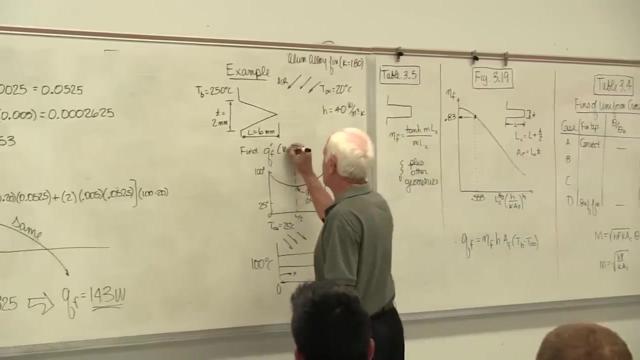 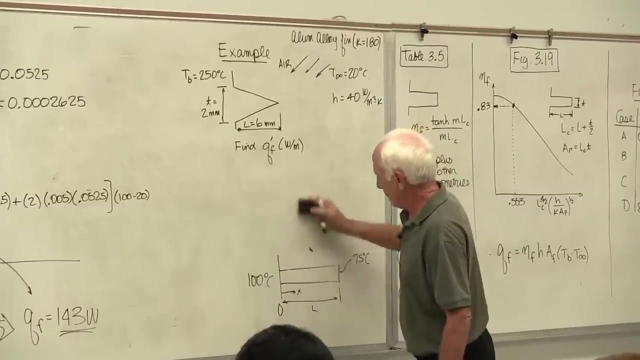 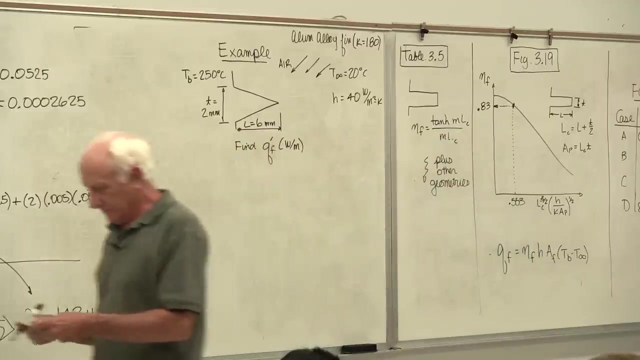 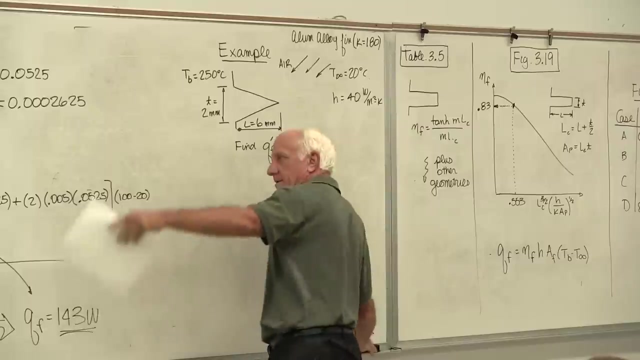 Got it. H now is 40.. Find Q sub F. Oh, find Q sub F, prime Watts per meter. Okay, Start over there. Use table 3-4.. Go to table 3-4 and read the heading. 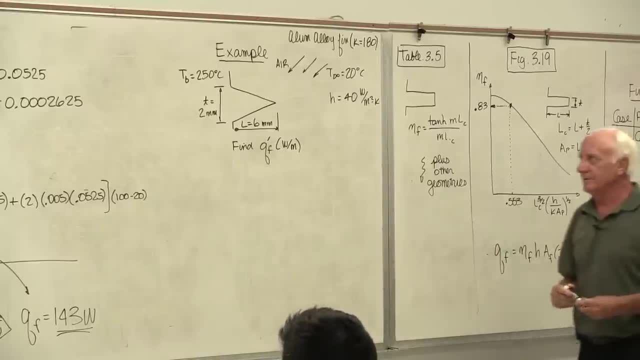 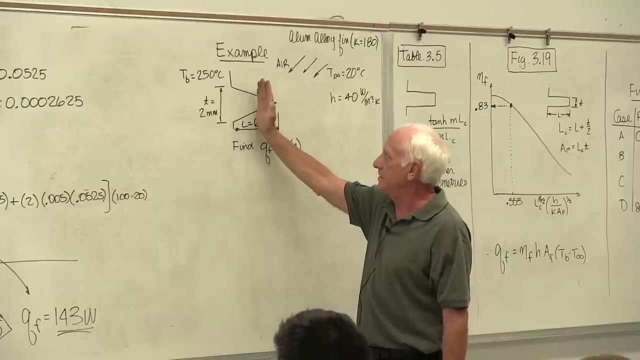 Fins of uniform cross-section area. Oh no, If I cut the fin here at that X location, I get a big area. Cut the fin in the middle at that X location, a smaller area. Cut the fin near the tip, I get about a zero area. 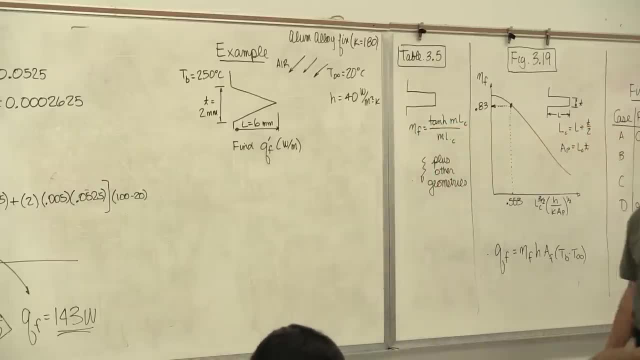 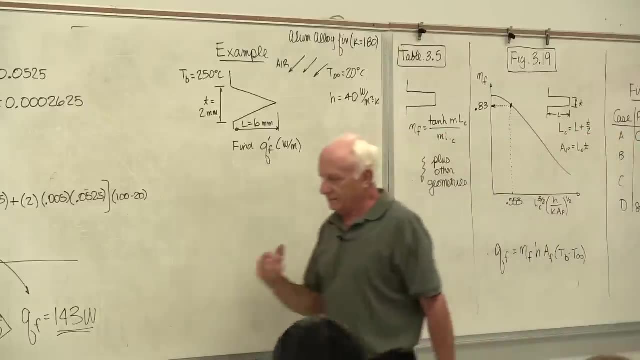 So it's not uniform cross-section area, I can't use table 3-4.. Okay, keep going. Let's see Table 3-5.. Oh, yeah, On table 3-5, I didn't plot it on there. 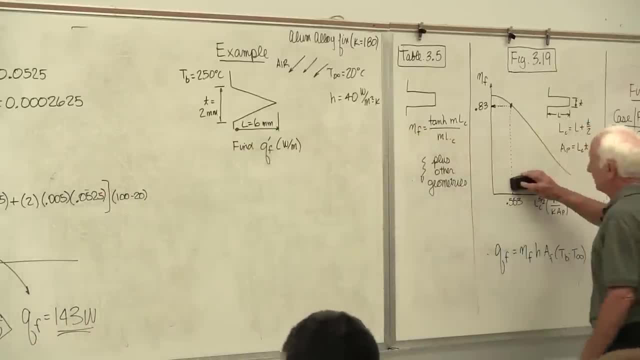 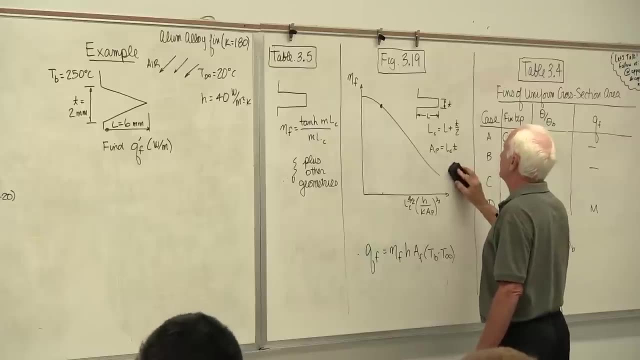 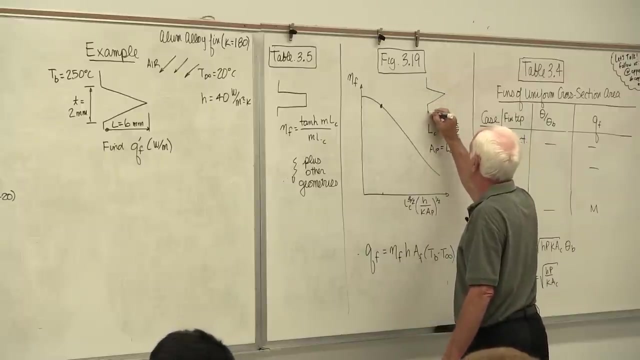 It gets too crowded. But there's another A line, There's a second line on table 3-19, figure 3-19.. That particular one has the picture of a triangular fin. Okay, L sub C, he says, is equal to L. 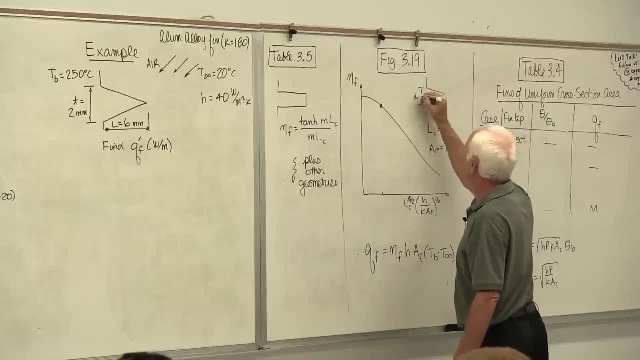 This distance here is T, So profile area L sub C times T, which is just L times T over 2. It's half, One half base times height. What's the base T? What's the height L? We can leave L sub C out of there. 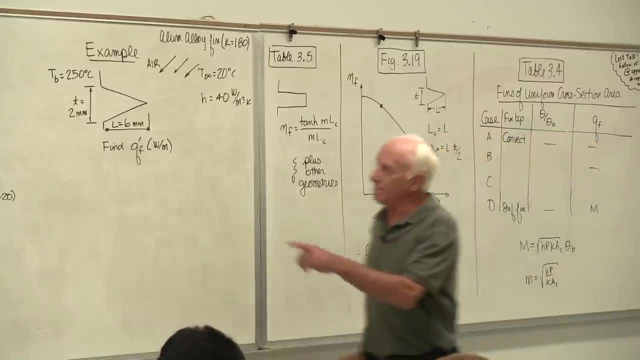 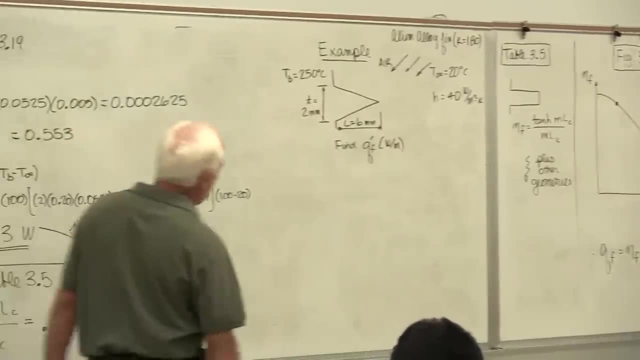 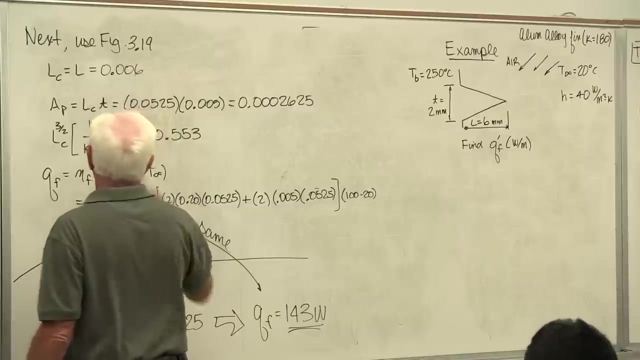 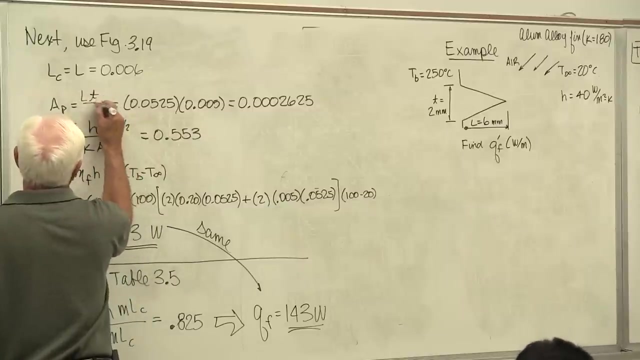 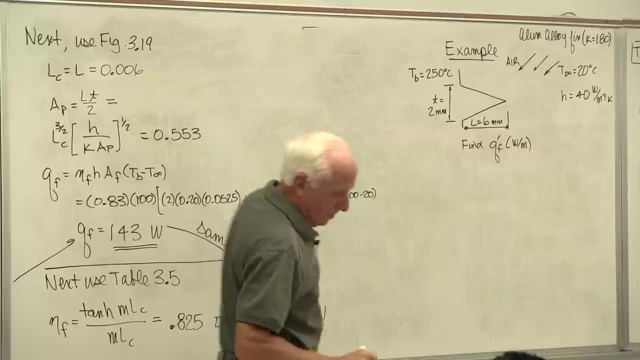 Okay. So let's go over here and say use figure 3-19.. Let's put some numbers in there. Six, okay, Okay. L, T over 2, profile area: Okay, It's small, Everything's in millimeters. 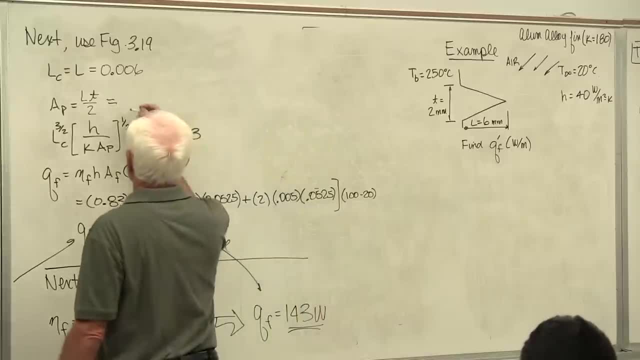 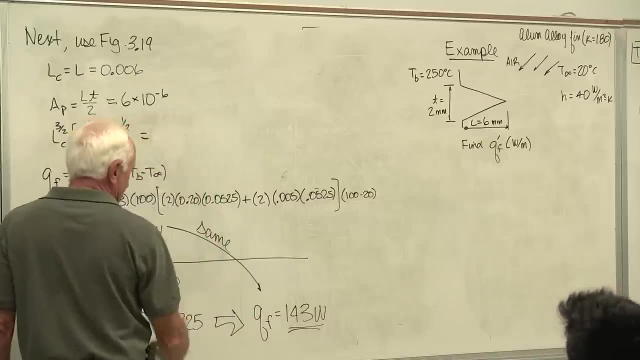 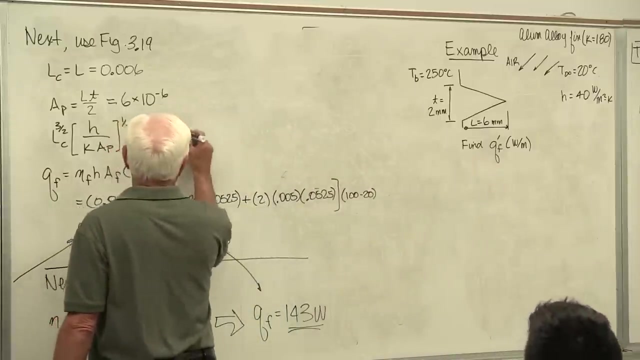 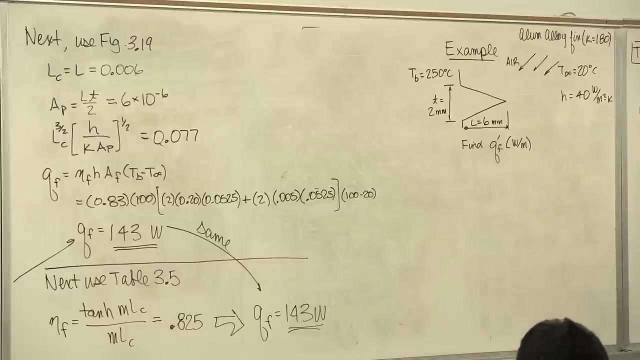 Two times 10 to the minus, or 6 times 10 to the minus 6.. Okay, Same x-axis parameter. There it is 0, 7, 7.. Okay, Okay, We go to the graph. 0, 7, 7.. 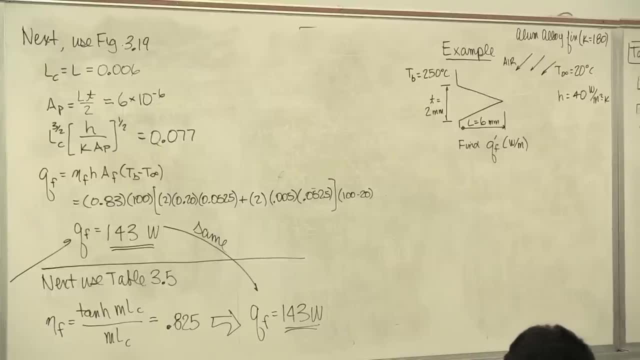 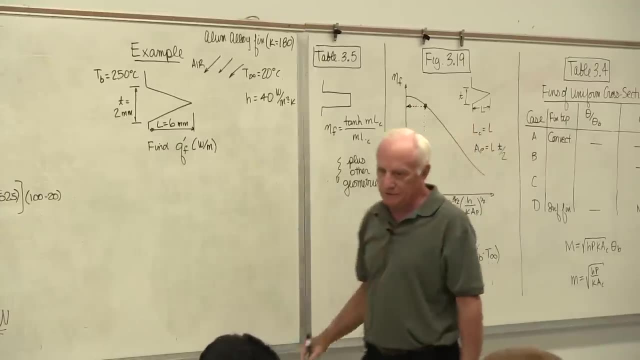 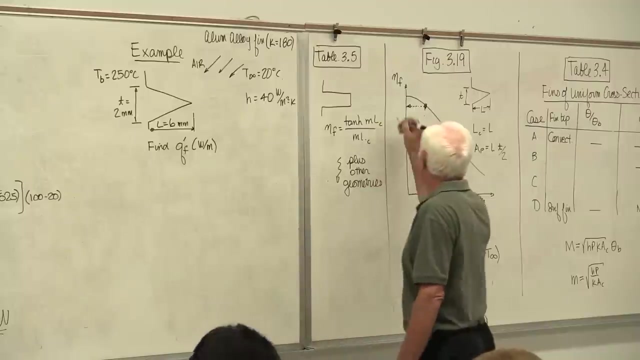 We read up vertically to the line for the triangular fin, We go across horizontally and we read The fin efficiency. Oh, it's somewhere between 9, 7 and 9, 8.. I use 0.98.. It definitely is not 0.95, and I'll tell you it's not 1.0.. 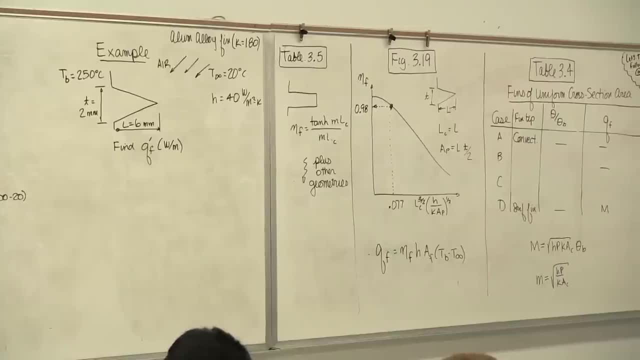 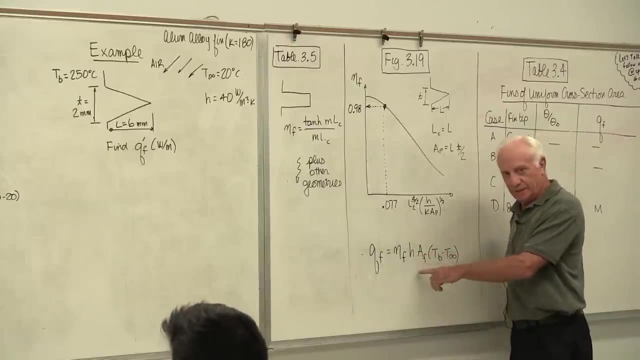 I can read closer than that. So I know it's between like 9, 7, 9, 8, around that area. All right, So now I know the fin efficiency. I again put it in the same equation. 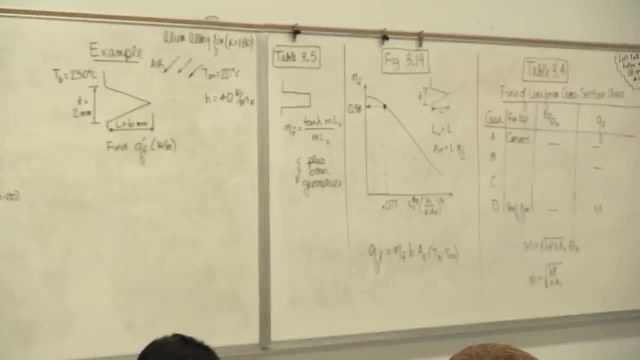 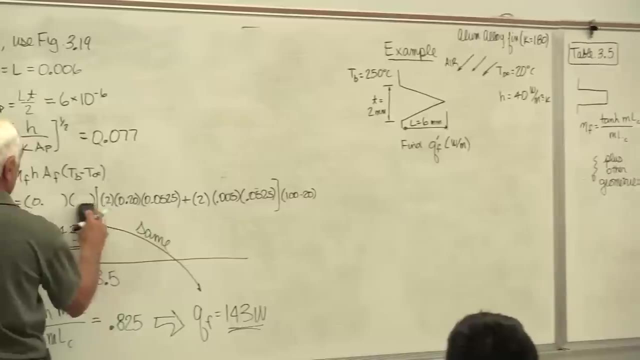 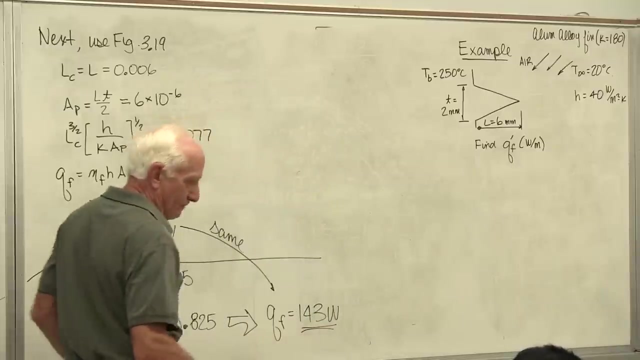 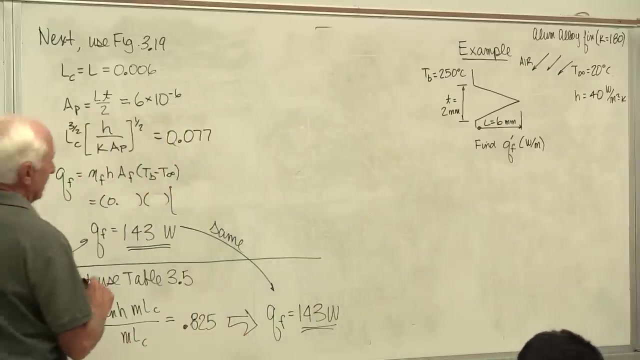 Okay A to fin H A fin T B minus T, infinity. So here we go. Okay, Let me just double-check my base temperature: Yeah, 250 and 20.. Yeah, Okay A to fin on 98.. 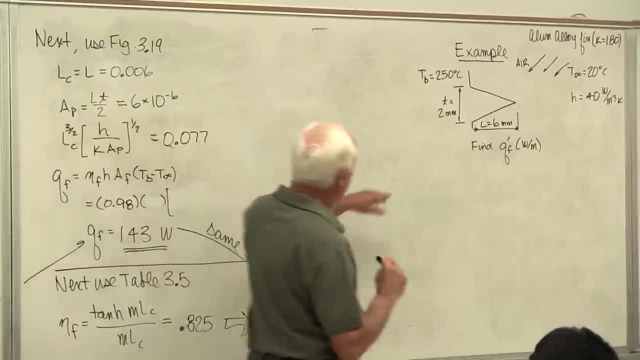 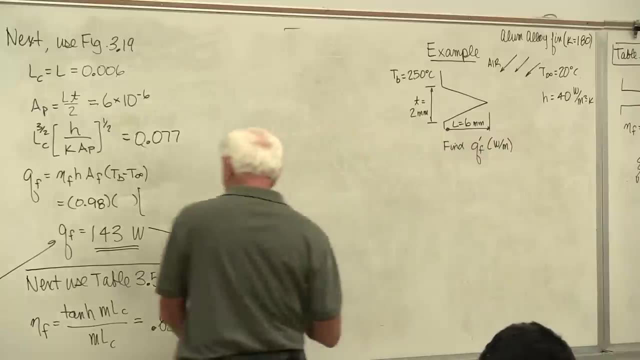 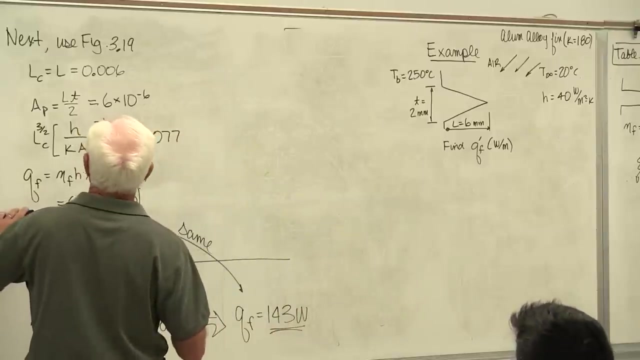 I read off of there: Oh, by the way, if you want to do it this way here, you can do it that way too. Oh, that was our table. Oh no, Okay here, Let's put that here. 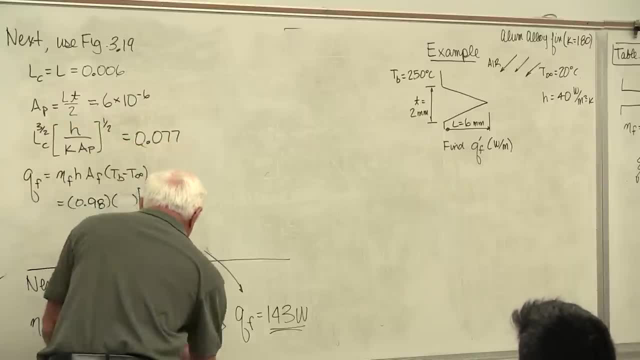 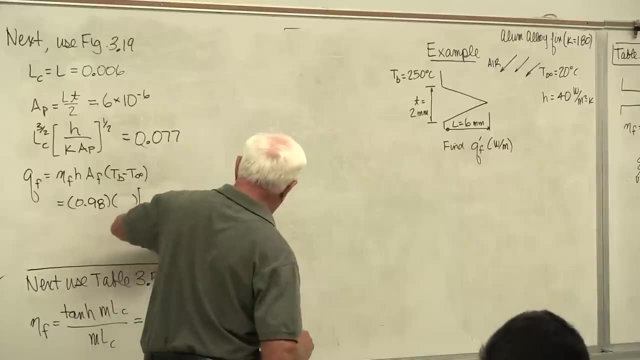 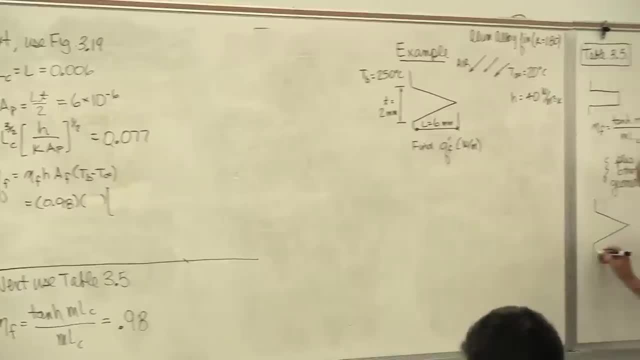 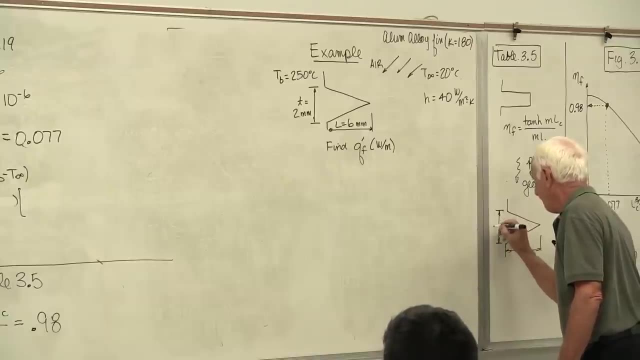 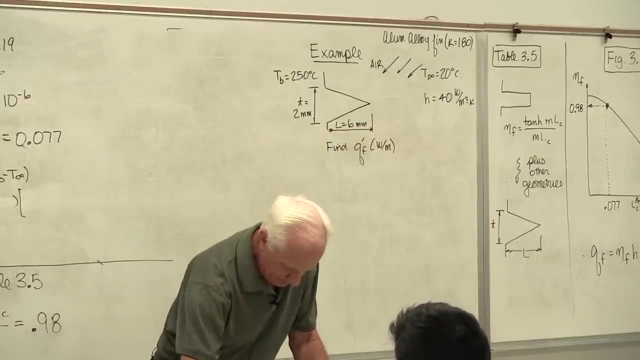 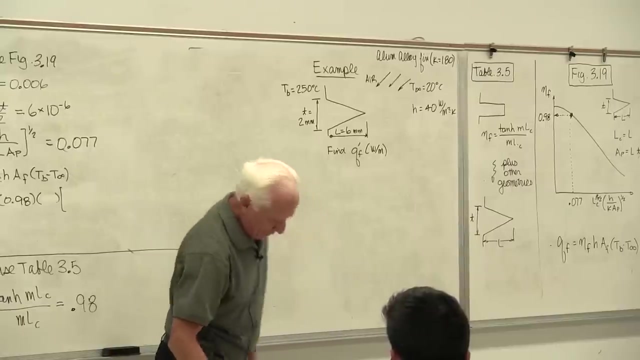 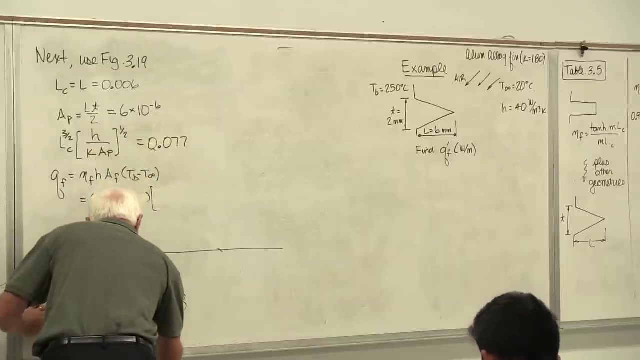 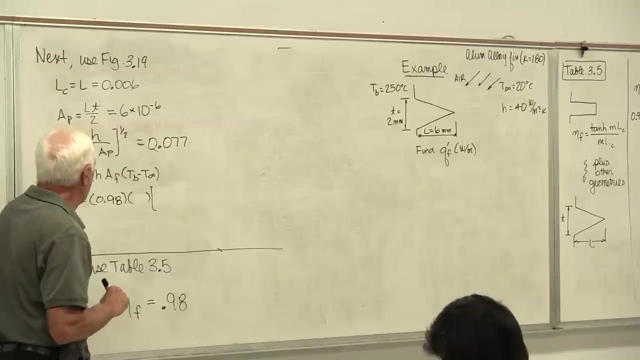 There is a triangular fin here. okay, Okay, Okay, Okay. so this is not the right equation anymore, But if you put the numbers in the equation in table 3-5, you'll get 0.98.. Okay, and here is 0.98. 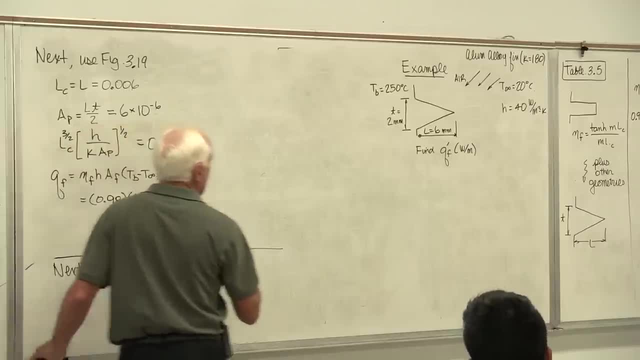 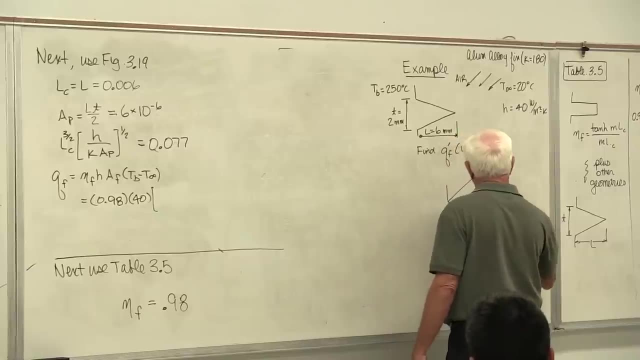 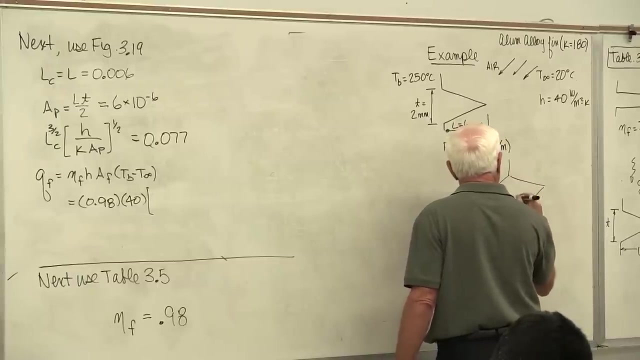 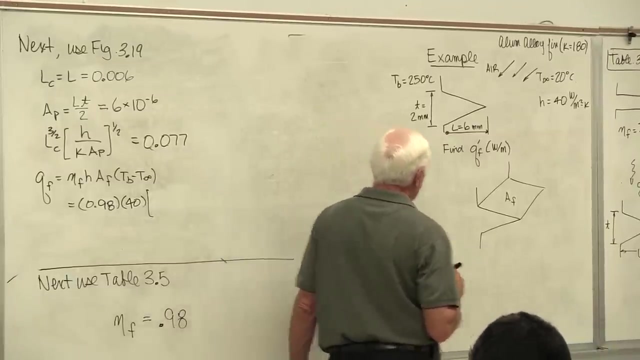 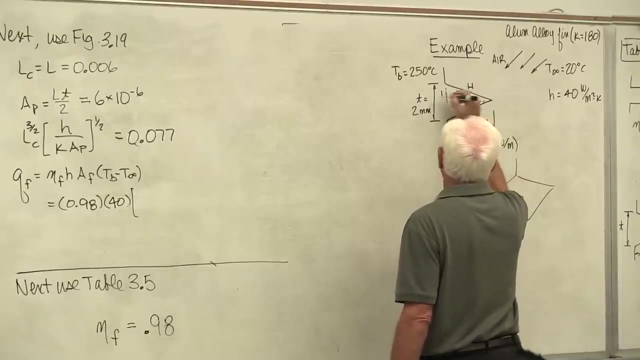 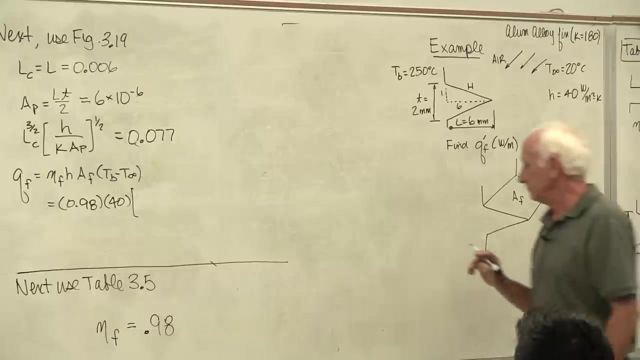 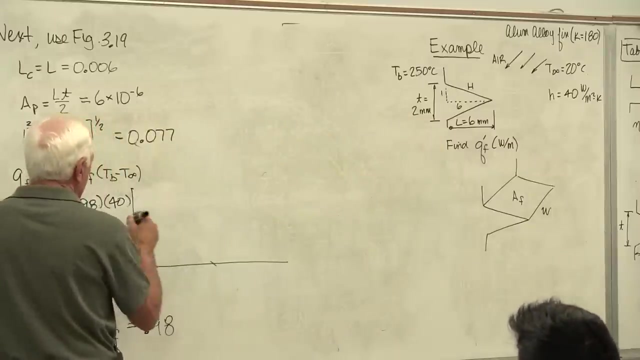 H was 40.. Okay, there's AF. That's the top surface of the fin, Hypotenuse 1 and 6, right triangle. If I want AF, AF is this distance, Distance multiplied by that distance, W. So the area of the fin, first of all, top and bottom. 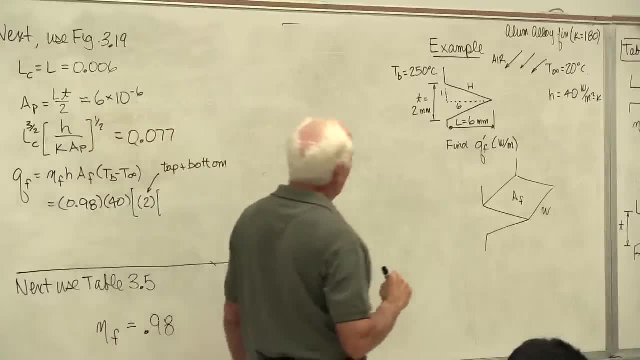 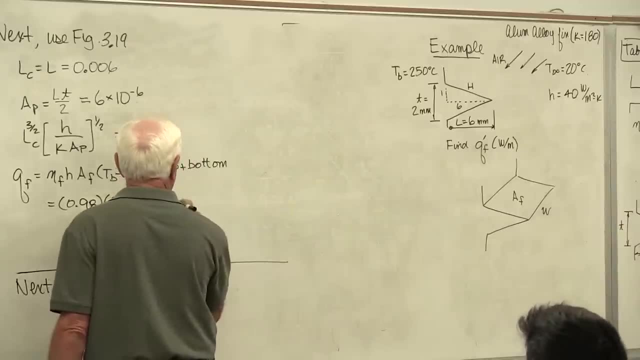 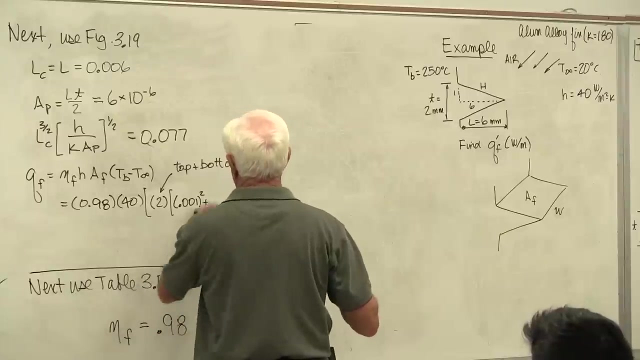 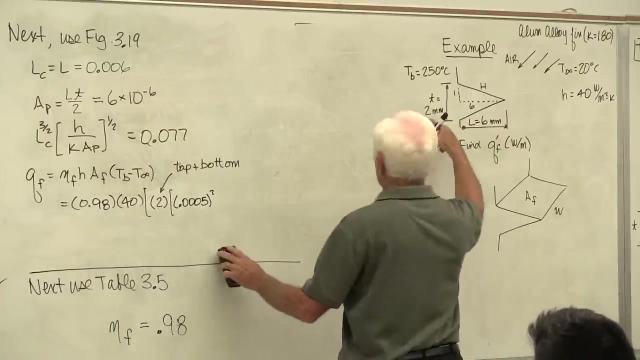 Now comes the hypotenuse: The square root of the sum of the squares, point 0,, 0,, 1 squared Half, three zeros and a 5.. Oh no, it was. I'm sorry, That was 2 millimeters, excuse me. 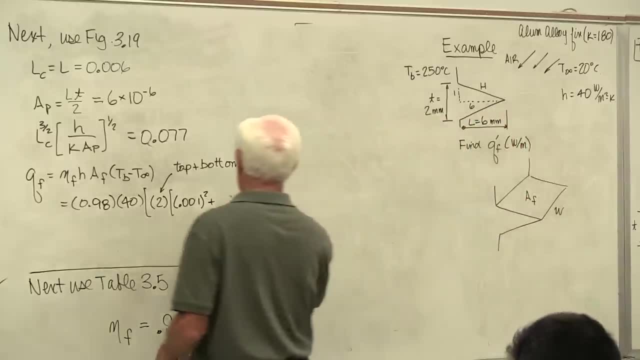 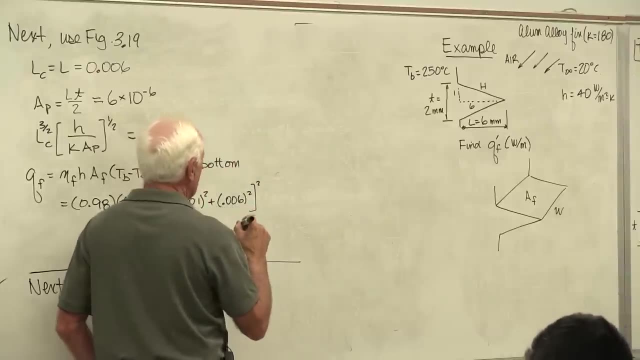 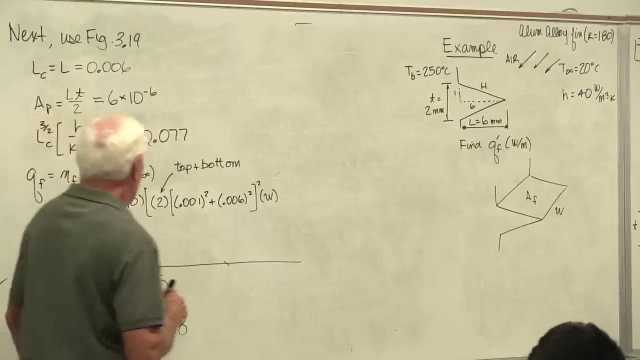 Plus, this distance is 6 millimeters. Take the square root, That's hypotenuse. Multiply that by W- I don't know W. Leave it in there. Oh, which one? Oh, thank you, I sure do. Thank you so much. 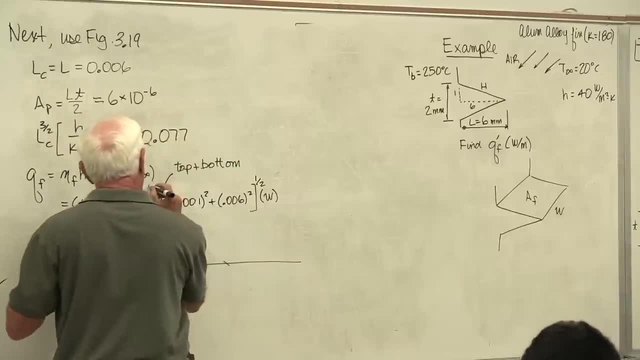 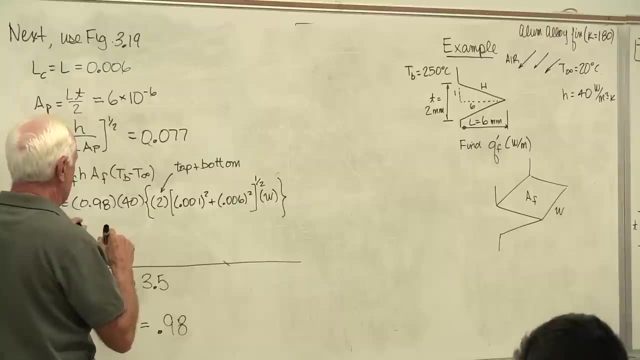 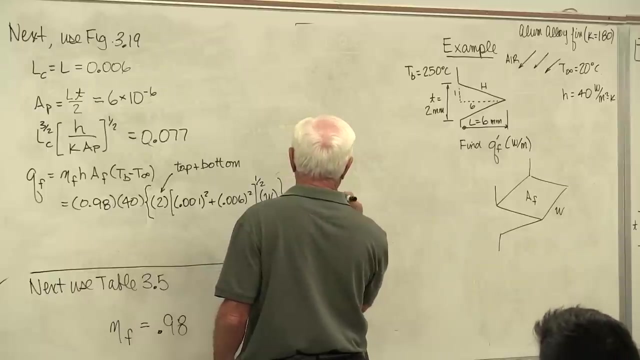 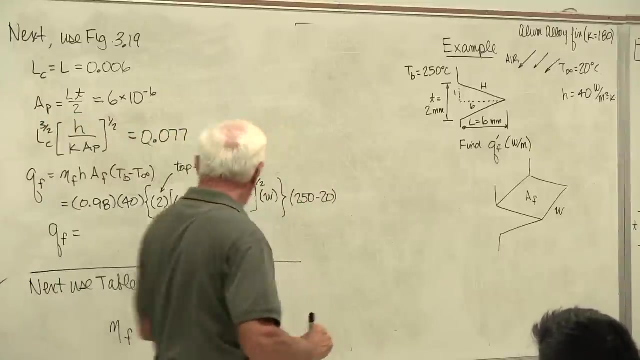 Okay, let's see how we're doing on that. Let's put a big bracket here. Yeah, so there's the area of the fin, And in the big brackets times T, base 250 minus 20.. Now I'm going to divide both sides by W. 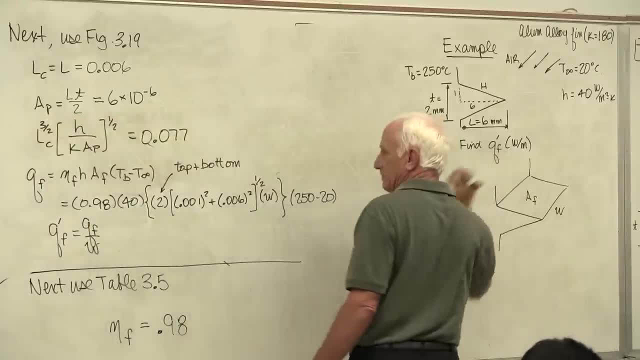 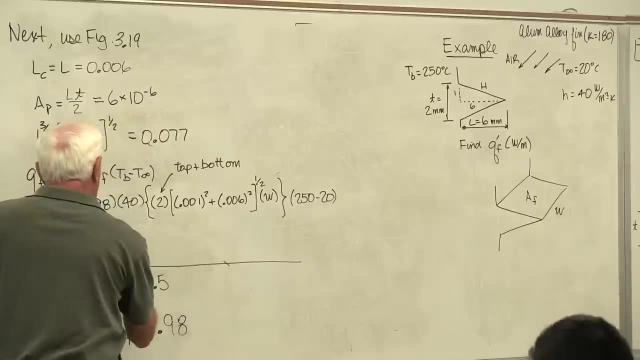 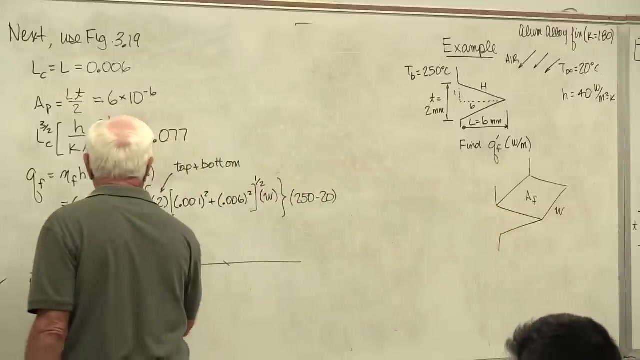 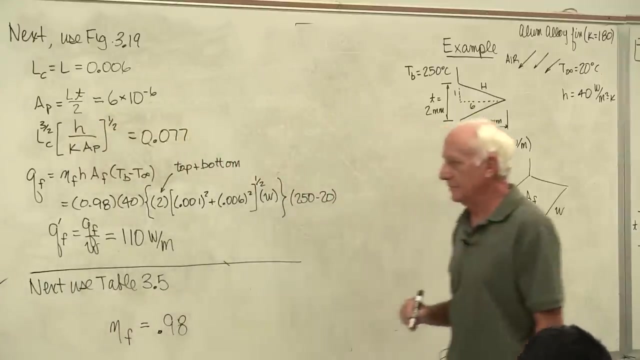 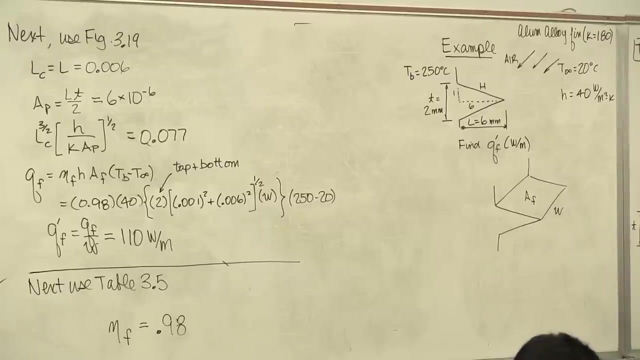 Because the problem said Q, prime watts per meter, divide by W the fin width, the W's cancel out And I'm left with 110 watts per meter. Your choice is: you can use figure 319, triangular fin, or you can use table 3-5.. 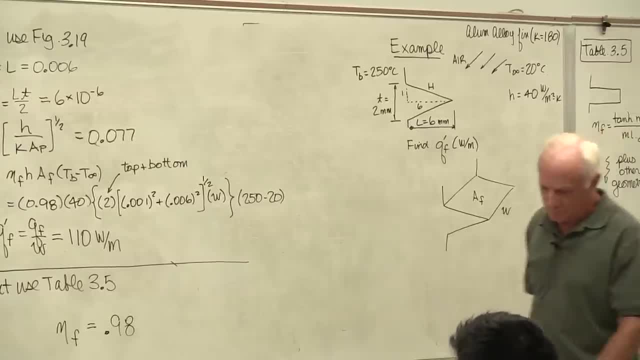 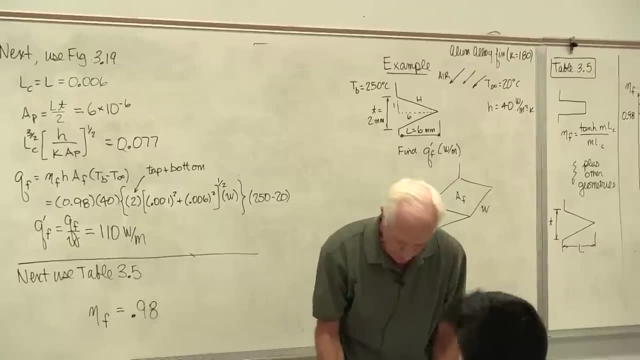 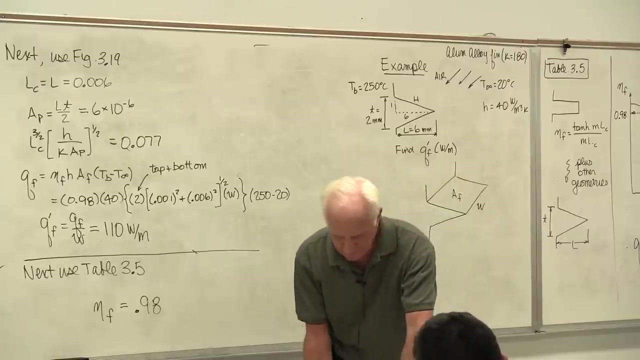 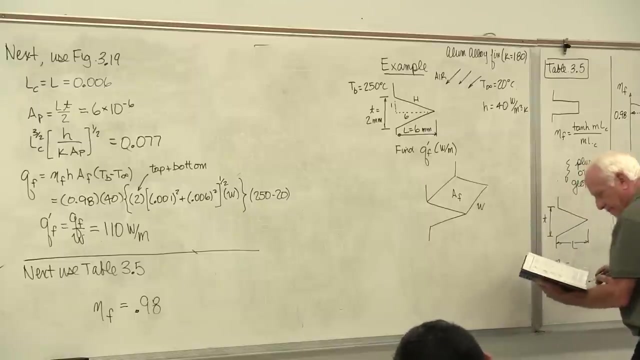 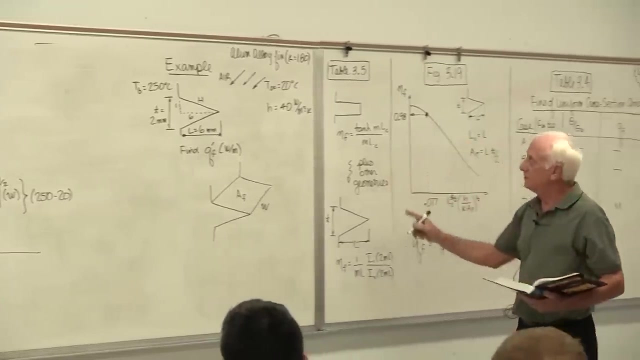 It looks like that: Yeah, now let's talk about that real quick, But before I do, I'm going to mention what this thing is here. Okay, I'm just going to put that down here. If you want to use table 3-5, there it is. 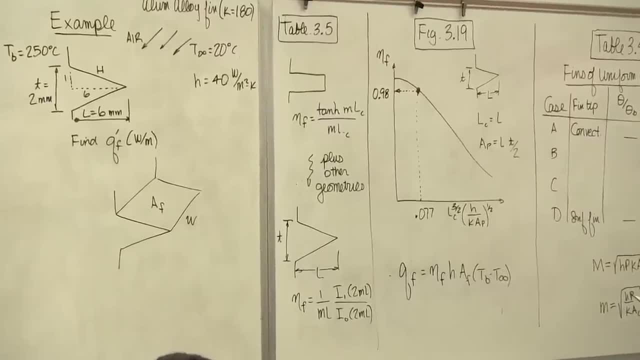 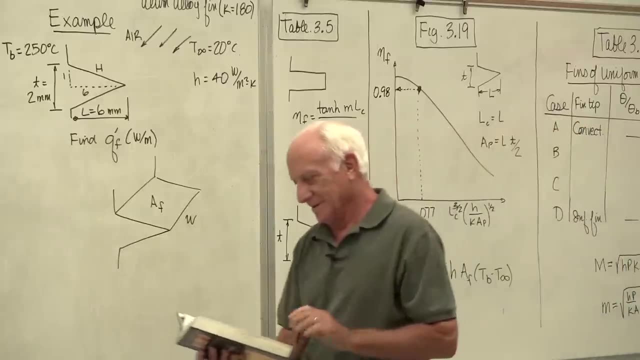 Yeah, oh, no, right, That's what I'm saying. If you want to use it, that's fine. It'll give you that, Okay, the right answer. but the oh-no part is here. they are Modified Bessel. functions of the. 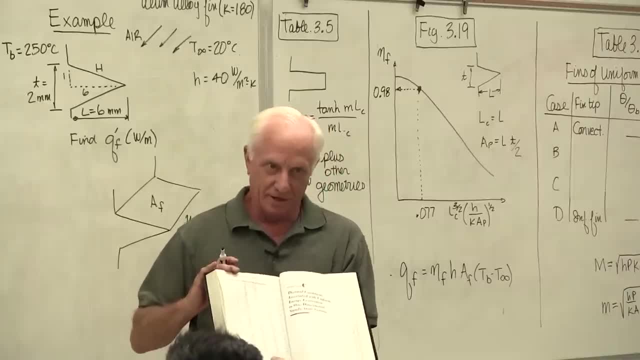 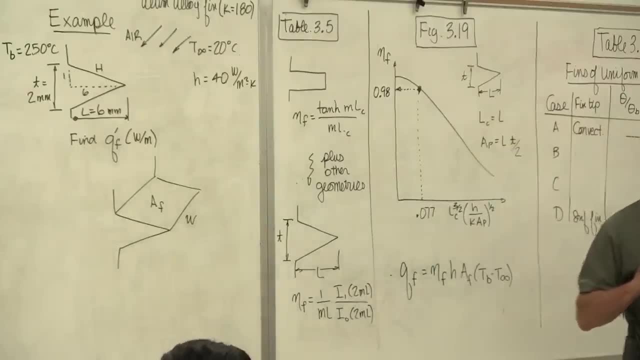 first and second kind, and the table is even difficult to read. I guarantee you it is not straightforward unless you know the code. So if you want to use Table 3.5, you will have Table 3.5 on the midterm, or you can use the graph. Most people like to use the. 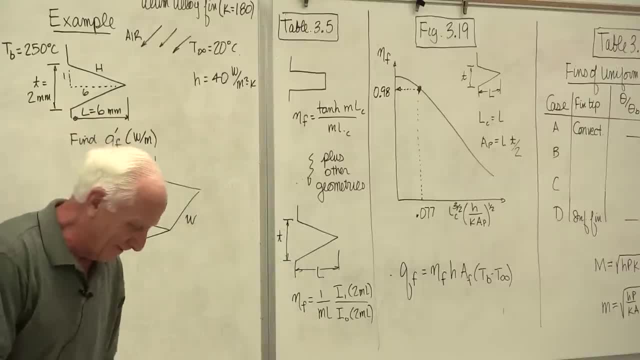 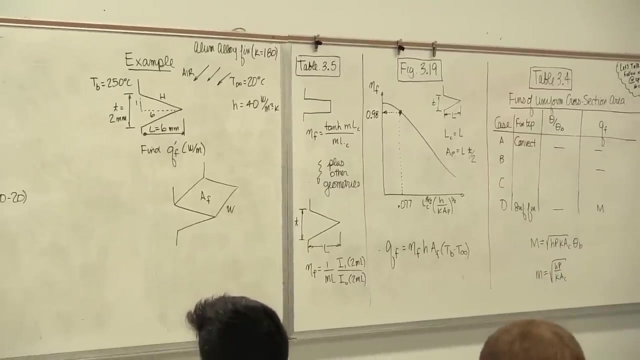 graph. But those are modified Bessel functions in the back of the book, in the appendix. Okay Now, so if I put them in there, I get the same thing For practice. go ahead and try it. You better get 0.98.. Okay now, why didn't I include the front and the back area? 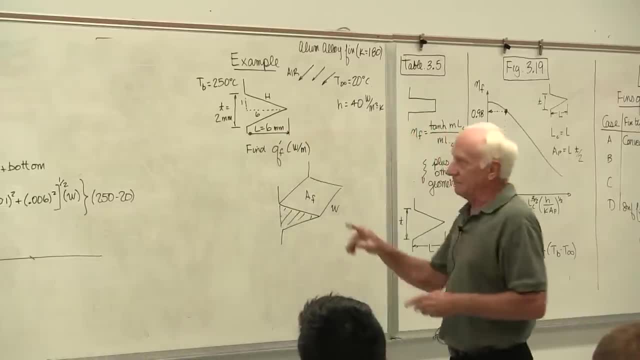 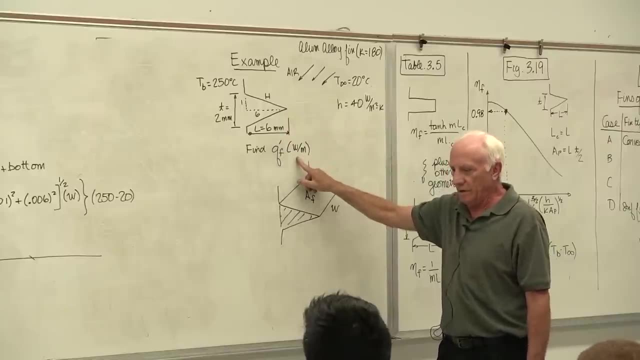 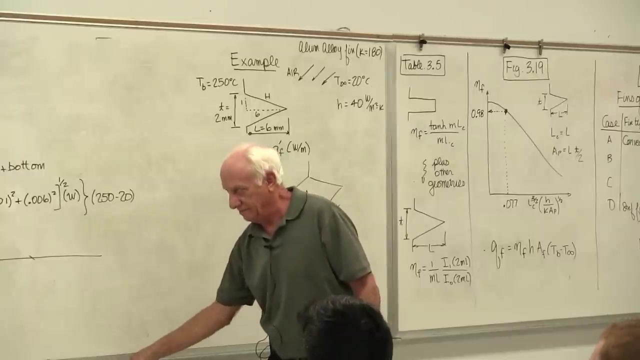 for convection heat transfer. Well, the problem said, I have got a long fin on the bottom fin. I want to know how many watts per meter are lost by that long fin. Well, what does a long fin mean? Here is a rectangular fin. It is like a pen holder. It goes from over. 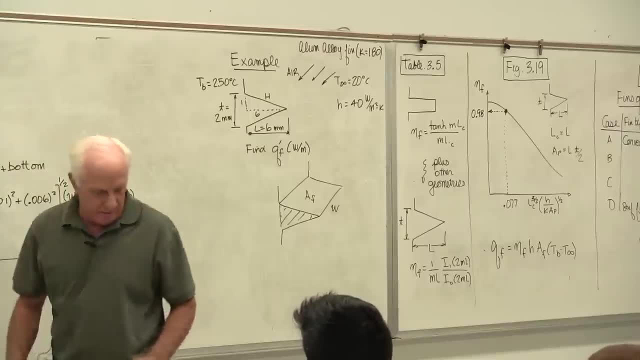 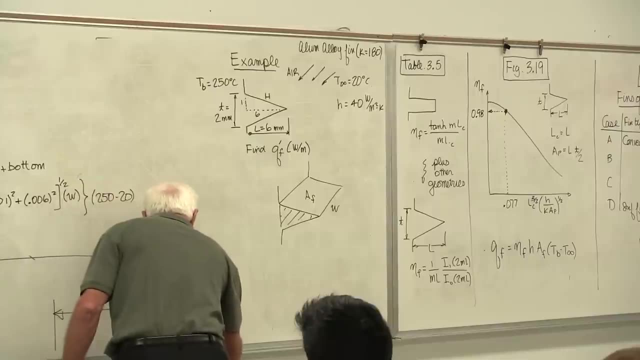 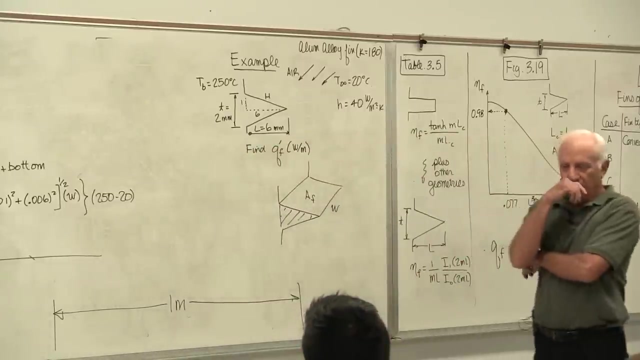 there, all the way over to there, If I take out a tape measure and say to you, I want to know how much heat is lost per meter of fin. There is a meter, I want to know how much heat is lost per meter. You tell me What area touches air. Okay, there is no. 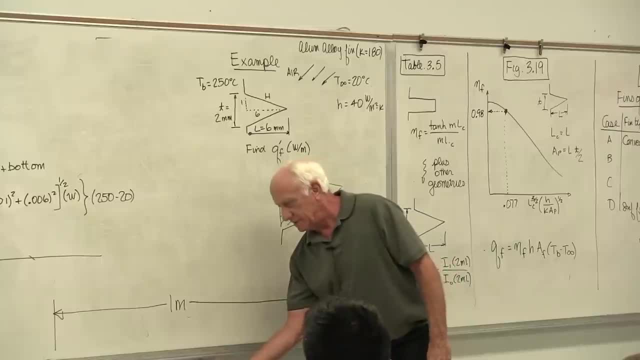 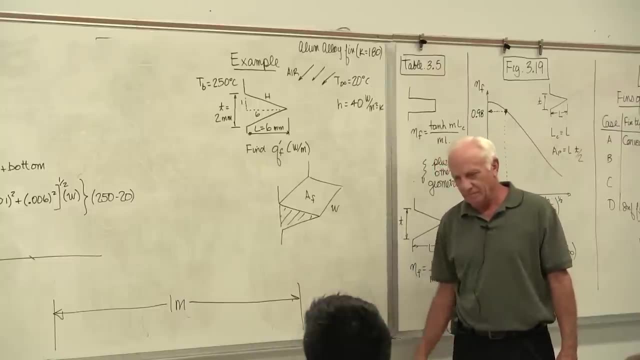 doubt about it. The top does, The bottom does. Does the left side? Of course not. Does the right side? Of course not. There is aluminum. It keeps going on. So that is why you don't include the front and the back. This is a long, a wide fin. We don't know how wide. 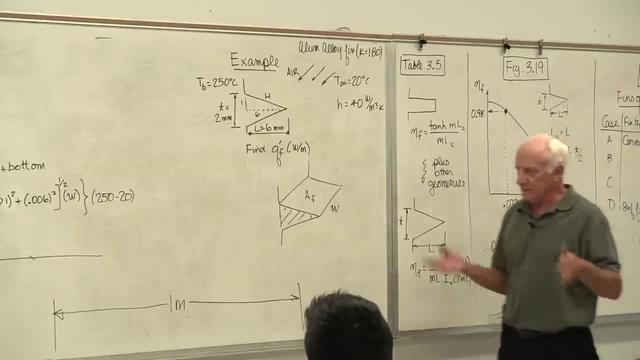 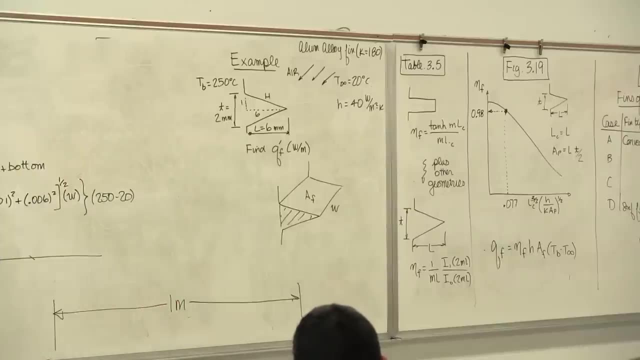 We are taking one typical meter out and the only part of that fin that touches air is the top and the bottom. Okay, now let's take another one. Let's take a circular fin. Okay for a circular fin. we have done triangular, We have done rectangular, Now we will do circular. 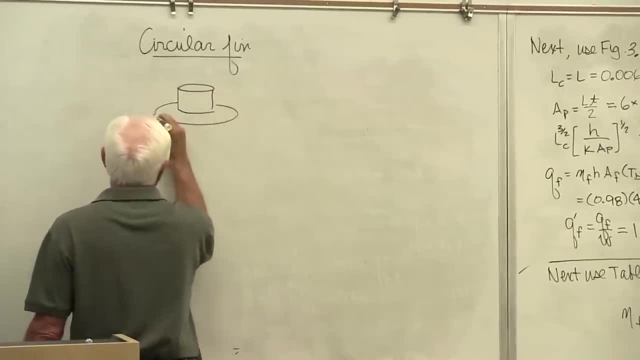 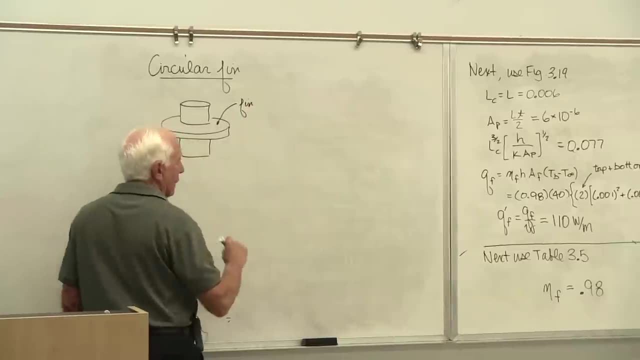 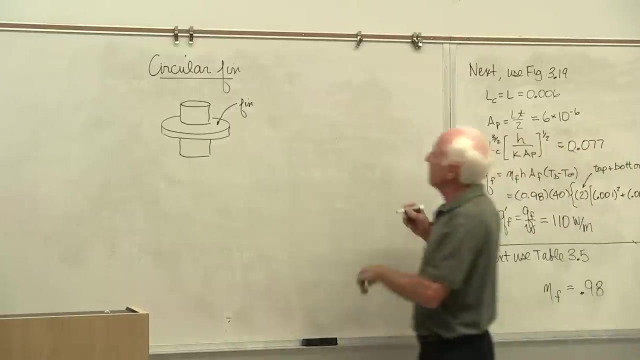 Okay, so there is a circular fin. Try and use 3-4.. No, you better not. You would be dead wrong, Because if I make a slice through that fin at different radiuses, starting at our inside and going to our outside- 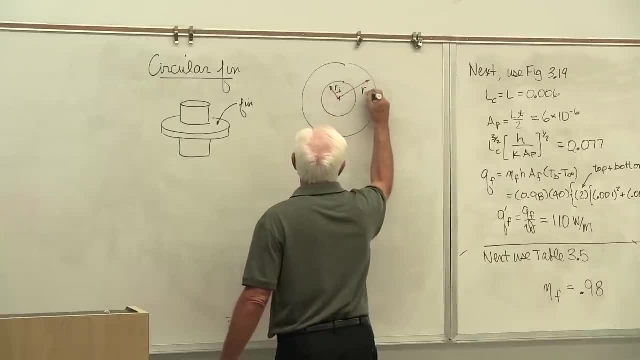 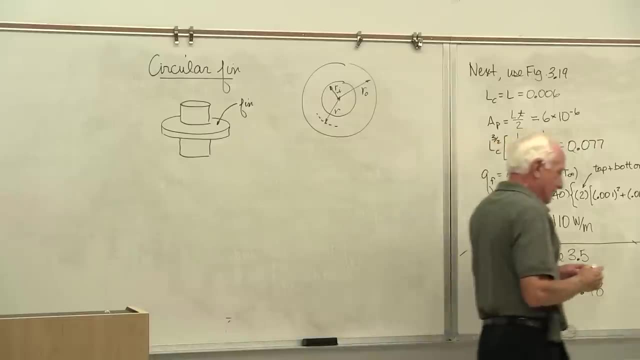 And if I look at a particular radius right there, as the radius gets larger, does the cross-sectional area for conduction get bigger? Yes, it does. Yes, it does, It gets bigger. It's not constant. So no Conclusion: You can't use table 3-4 for circular fins, Can. 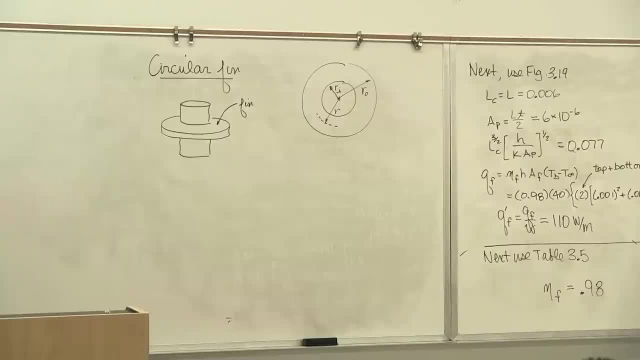 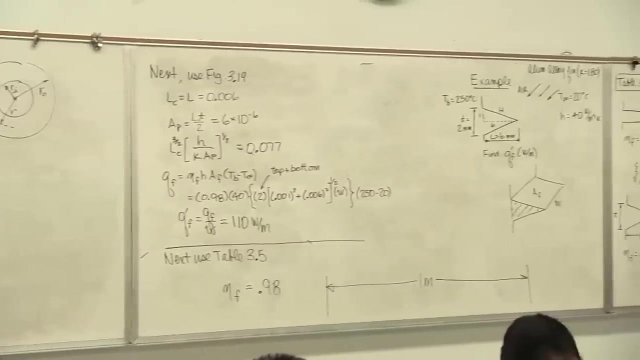 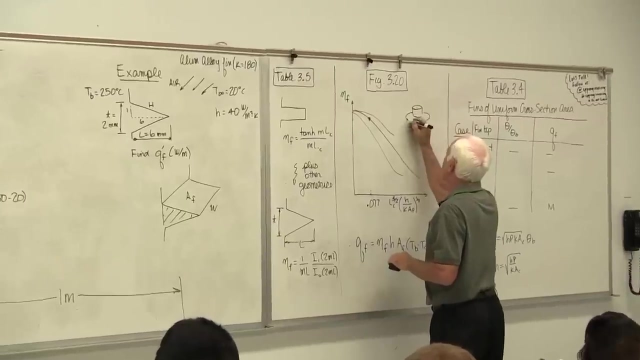 you use a graph for circular fins? Yes, you can Go to figure 3-20.. Figure 3-20.. And it has a bunch of different graphs on here, But it is for the picture shows you there. it's for circular fins. Yeah, it's. 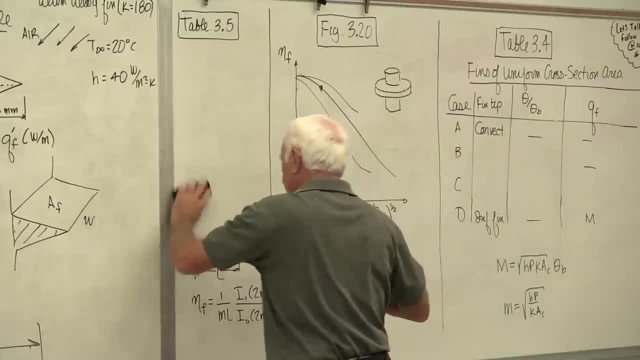 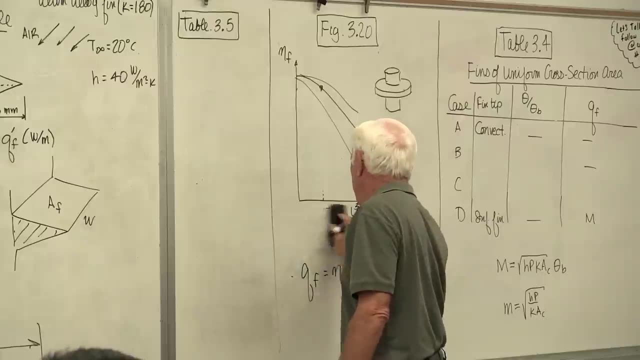 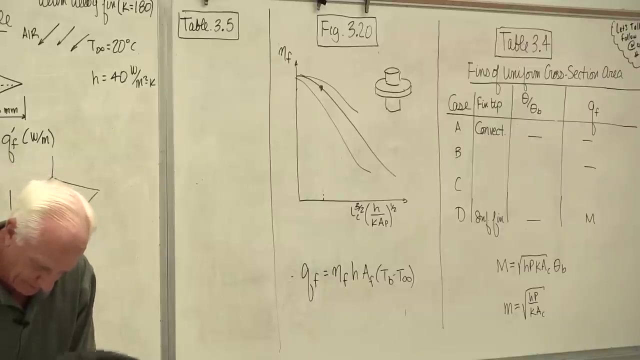 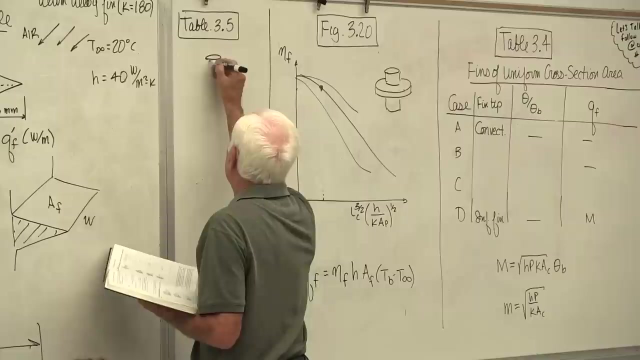 there. So you say, well, okay, but can't I just get an equation for it? Yeah, you can get an equation for it. Let's go to table 3-5.. There it is table 3-5.. Table 3-5, okay Again. 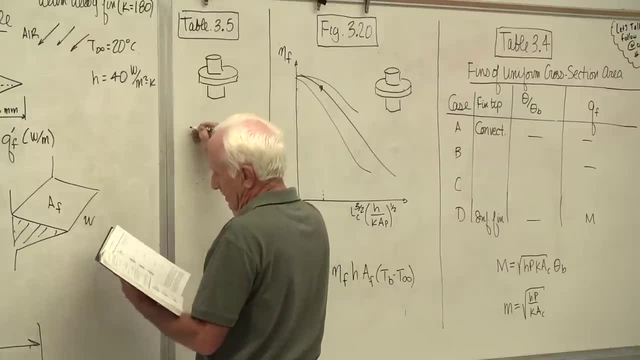 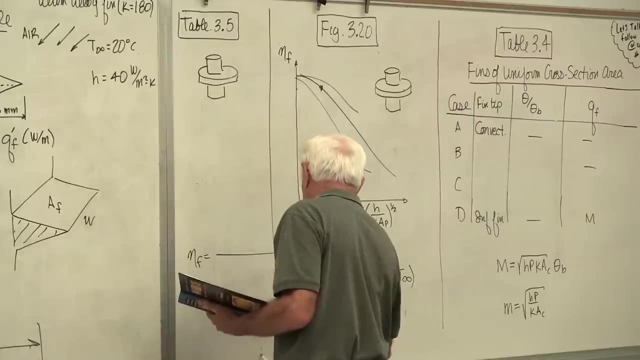 circular fin. Okay, here is the fin efficiency. Today I'm going to picturesque. We're going to draw the line across the side. See the line across the side. No, give me the line to the side. So here's the line to the side. Here's the line to the side. 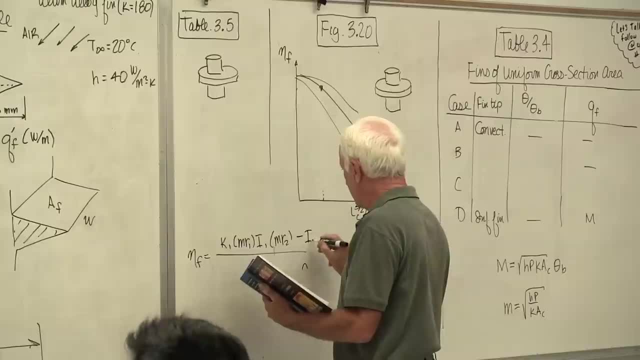 Okay, here's the line. So that's the line. so I'm going to draw the line so that the line can be edited out. I'm going to go this way. Okay, Like this. Yes, Like this, Yeah. 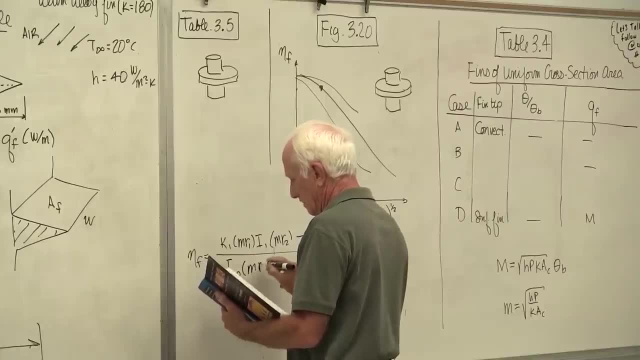 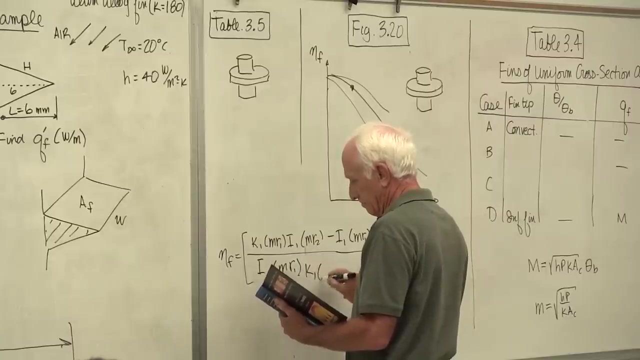 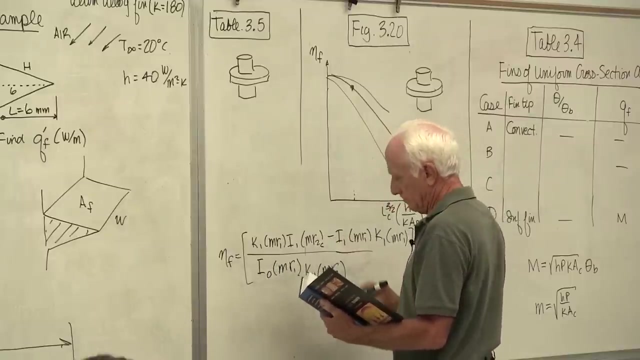 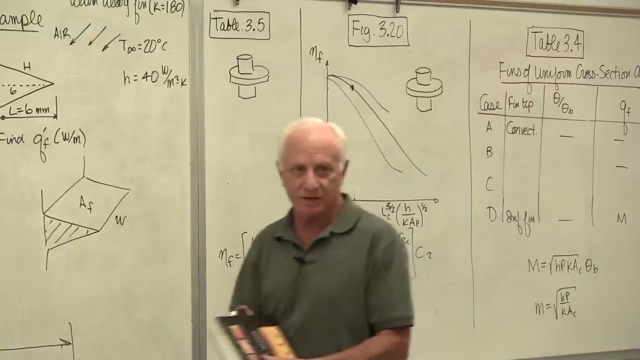 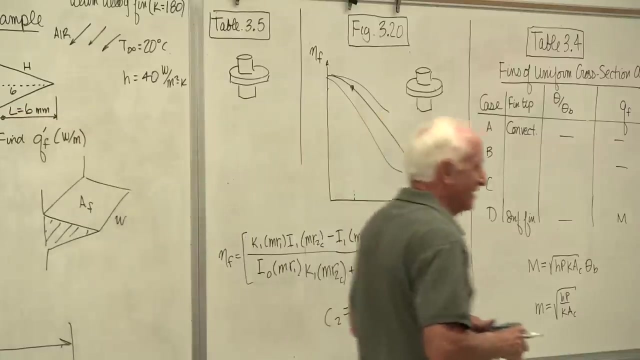 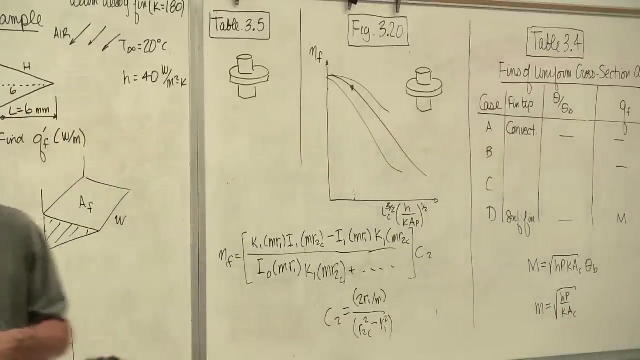 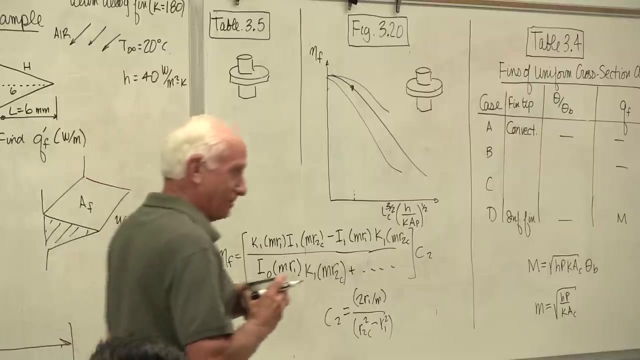 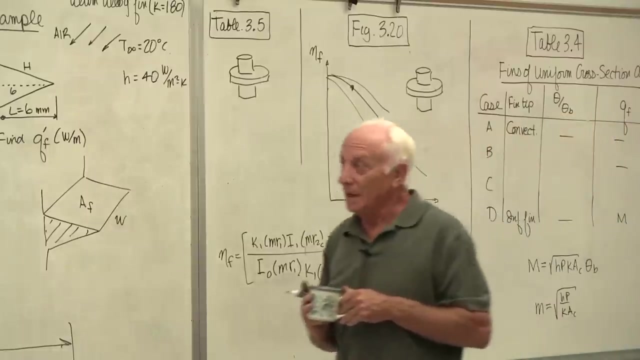 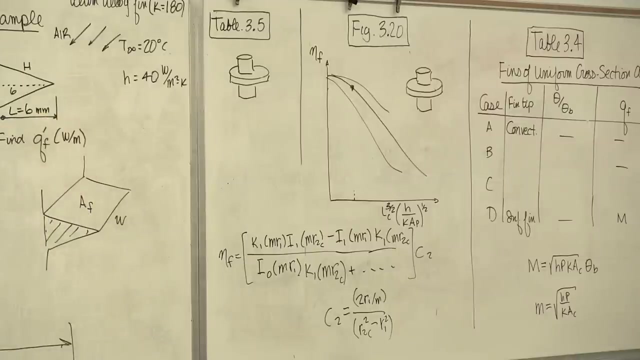 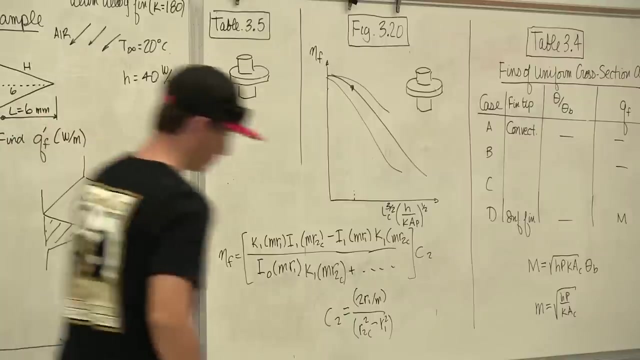 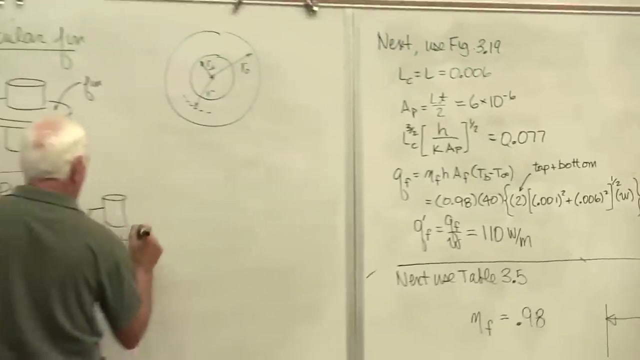 Thank you, Thank you, Thank you, Circular fin, you can use figure 320, or you can use table 35.. Now maybe you want to go to a pen fin Looks like this, Or maybe a pen fin that looks like this: 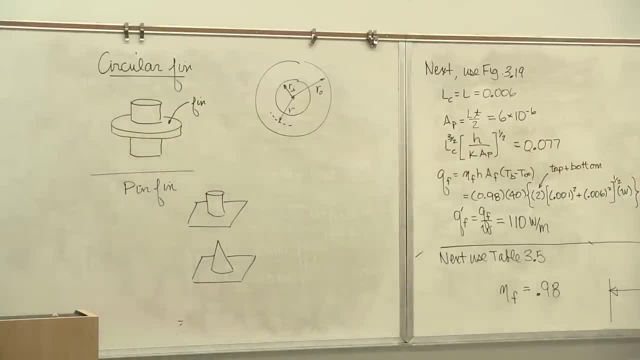 Okay, Which guy here? Do you have arm cross-section? Oh yeah, You want to This one. Slice it Pi r squared, pi r squared, pi r squared. Ah, this one, I can use table 3-4.. 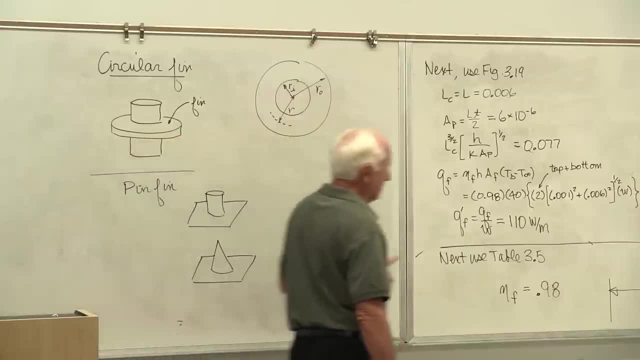 This one. I can't Okay The graph in here, the pen fin. there's no pen fin in here. okay, The table 3-5, yeah, table 3-5.. Has, Has, Has, Has. 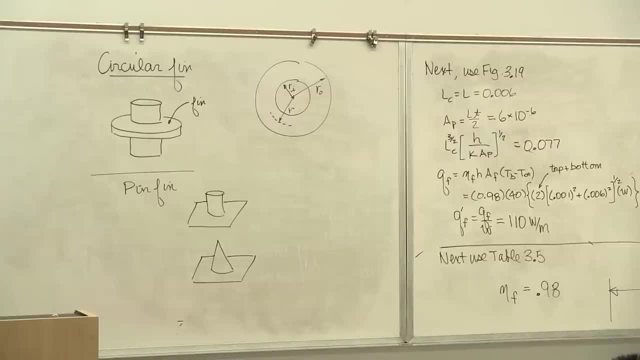 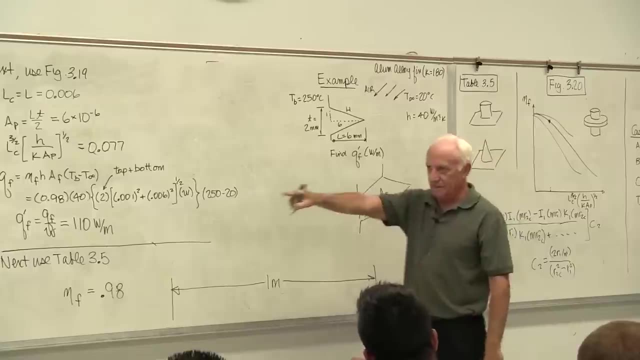 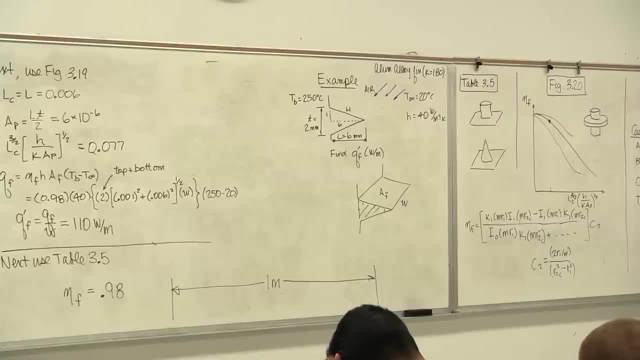 So, again see, you've got three possible resources to solve fin problems and you have to pick the one that works for that particular application. So homework, you'll get a good feeling for that now. So homework, you'll get a good feeling for that now. on homework, 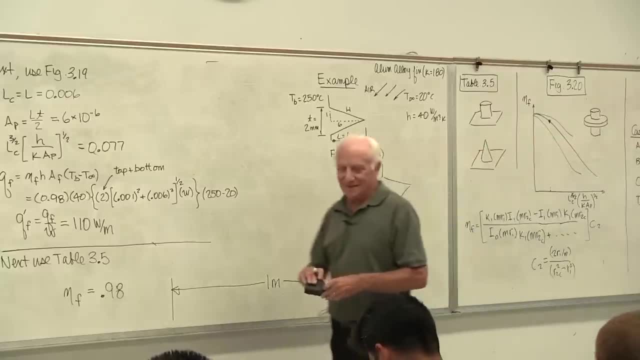 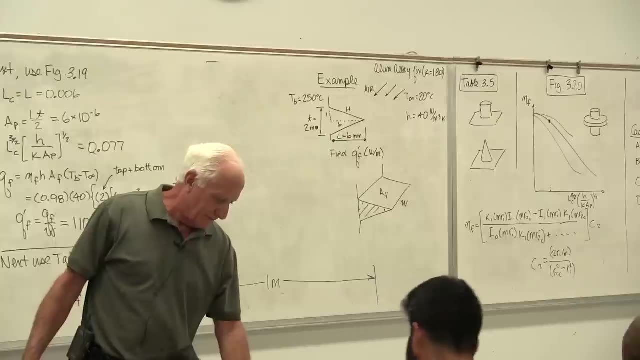 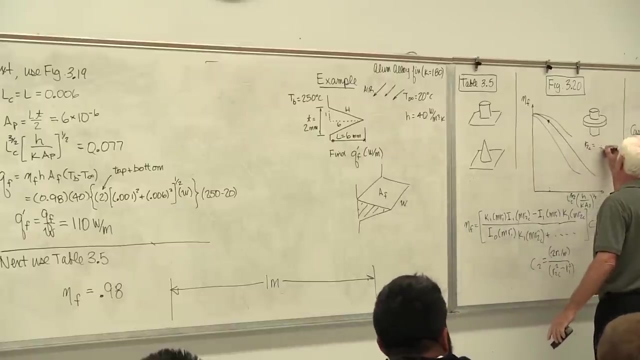 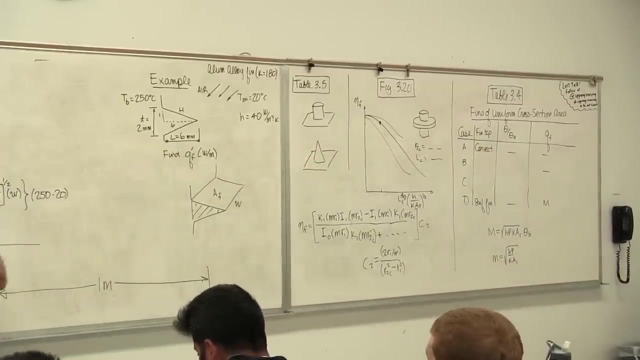 homework. Now the last topic in chapter three. anything else before I go on for the last one: Yeah, For circular pins. what would the LC and AB? just It's on the graph here. Like it says here: R2C equals so-and-so, LC equals so-and-so. on the graph. Okay, now of course, most of the 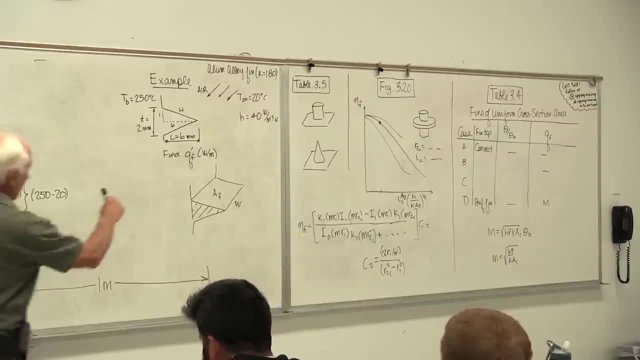 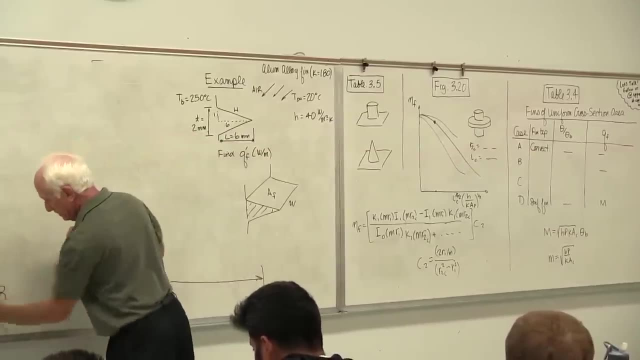 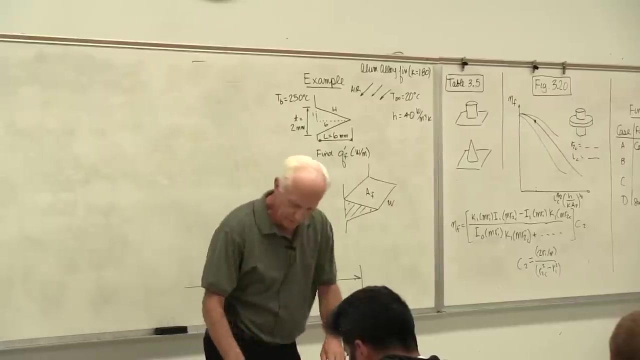 time we don't just stick one fin on a wall or one fin on a tube- There's multiple fins attached to a wall or a tube- Or we put thousands of these guys on a wall. Let's see if I've got that. Maybe I do. Let's see if I do here. Oh yeah, 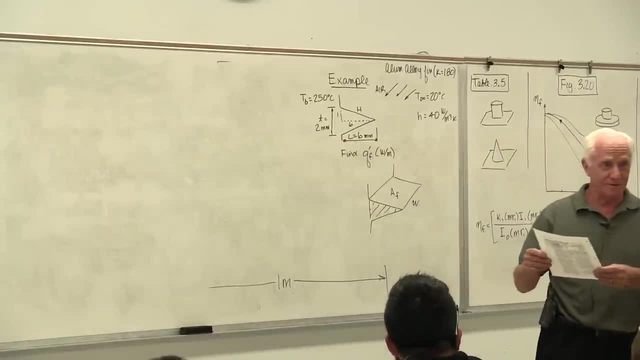 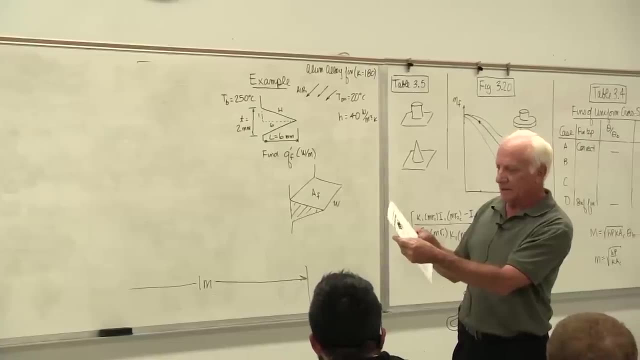 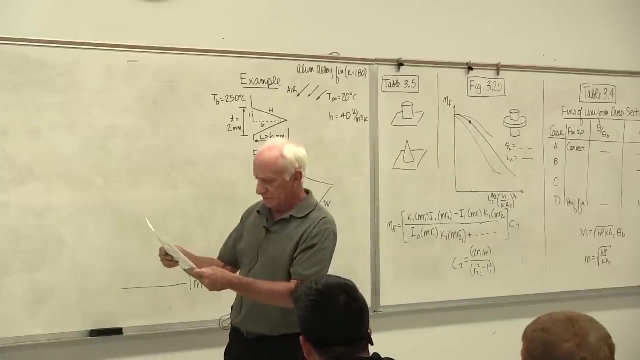 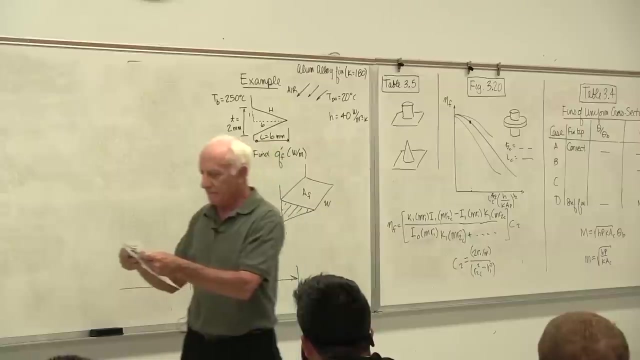 This is in Machine Design Magazine. We all Emmys know that Machine Design Magazine. okay, Cooling the pin-fin way, Electronic cooling in a small package. It's an interesting article, but I just want to tell you they're using aluminum and on this little electronic package they have the fins. 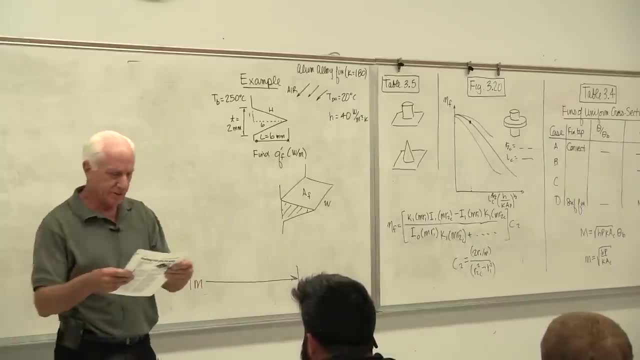 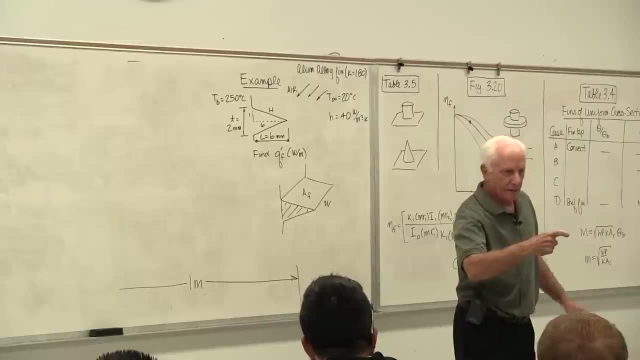 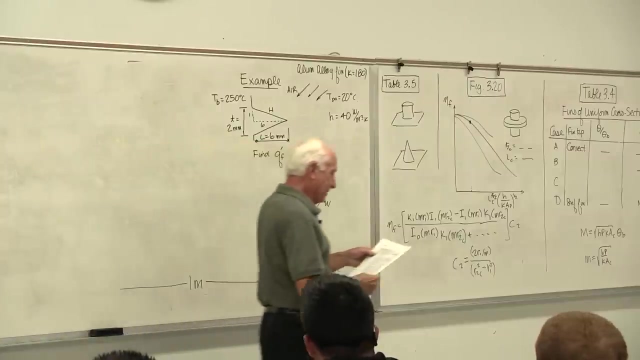 They have 619 fins on it. 619 fins, 2 1⁄2 by 2 1⁄2 inches, That big, by that big, there's 600 of those guys to take the heat away from electronics. Oh yeah, they pack them in there. So again, most of the time we don't just put one fin on something. 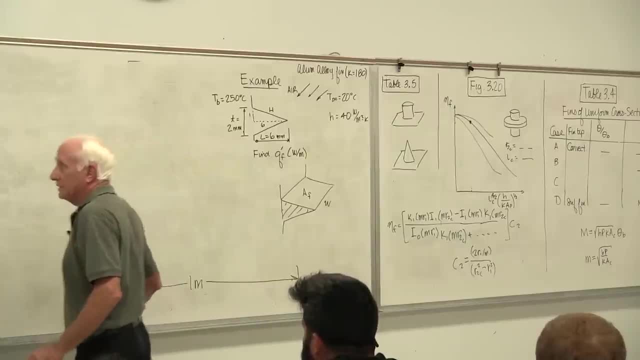 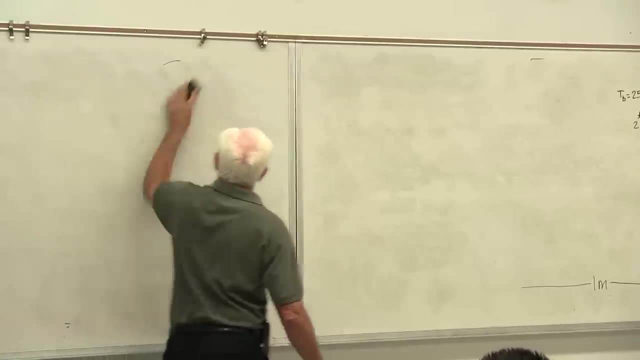 We put multiple fins on a surface. So if we look at that, how we tackle that, it's pretty straightforward, but there's a couple things you should be aware of. We'll show two cases. One is rectangular fins attached to a wall. 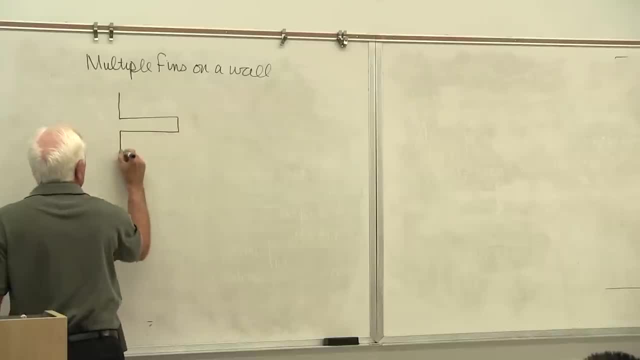 So here's some rectangular fins attached to a wall. Here's some rectangular fins attached to a wall. This is the base area, so T-base here. This is the fin area and there is some base area exposed to the ambient conditions. 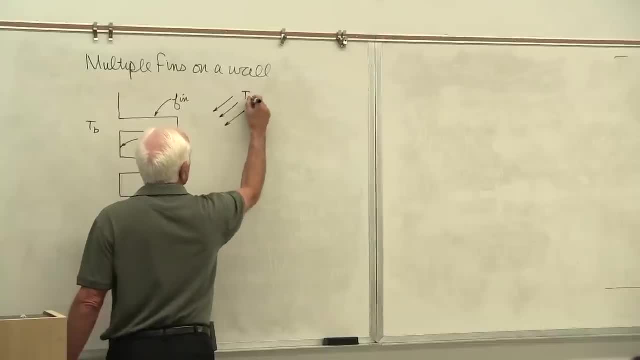 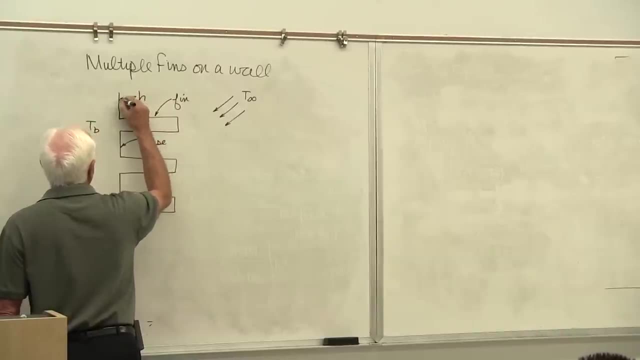 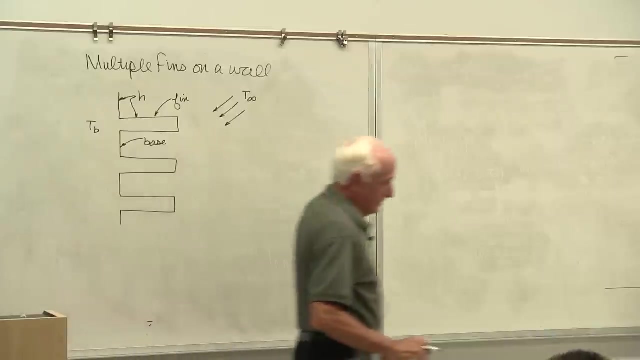 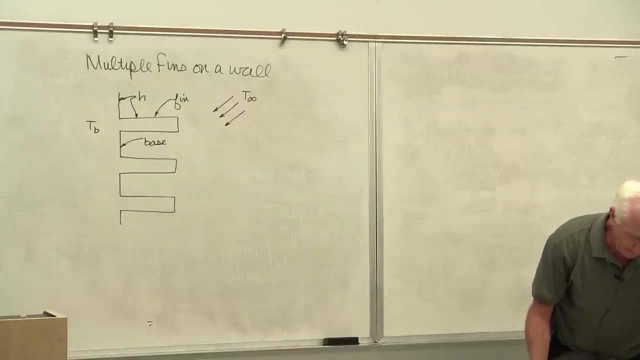 Here's a convection from, let's say, a fluid whose temperature is T-infinity and the convection coefficient on the fin and the wall is both H. assumed to be the same. So the equation that we want. And before those fin surfaces, we'll just write down the equation. 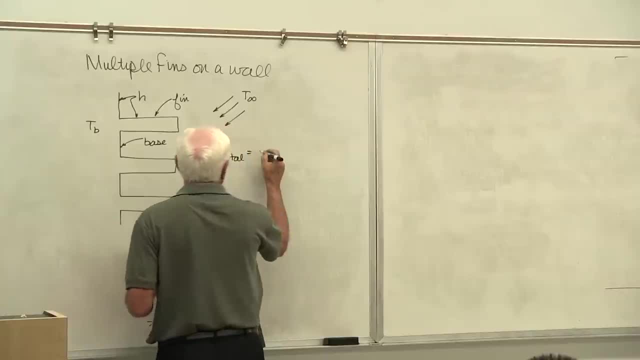 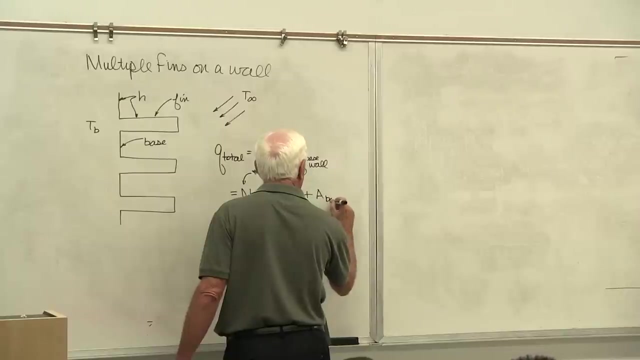 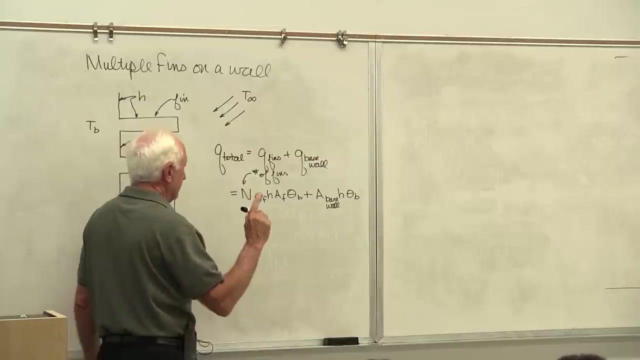 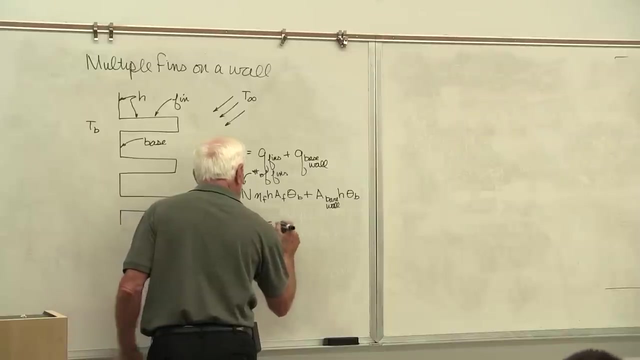 Q-total equal Q-fins plus Q-base wall. Q-fins. capital N is the number of fins times theta fin. H area of the fin times theta base plus the bare wall is the area bare wall times H times theta base. The area of the bare wall is equal to the total area. 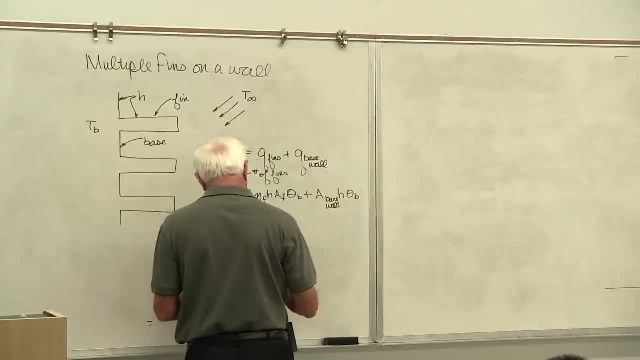 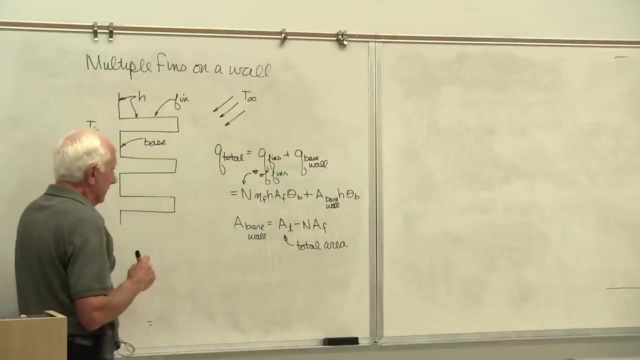 of the base area: N fins AF, the little squiggly line. that's the base area. You know the fin area. It's the top area. It's the top area. It's the top, bottom, front, back and the end for convection heat transfer. 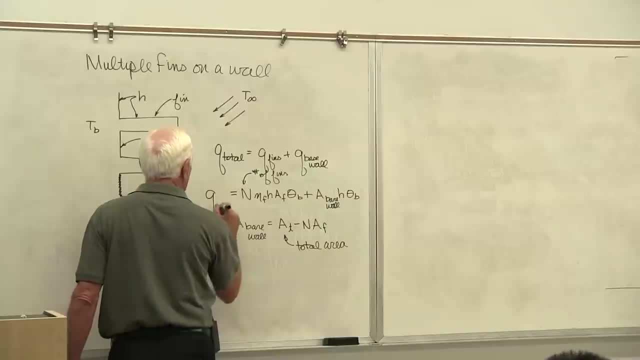 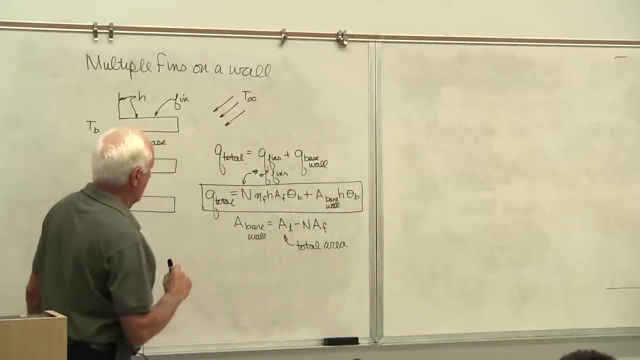 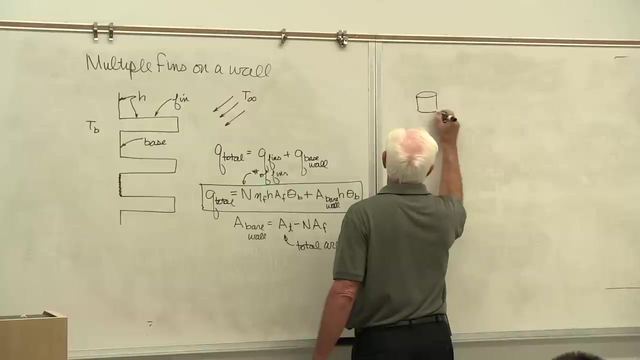 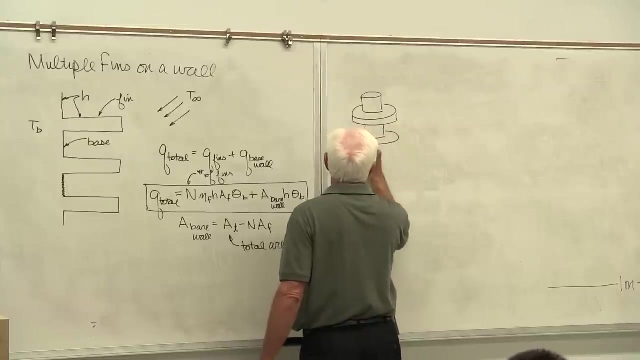 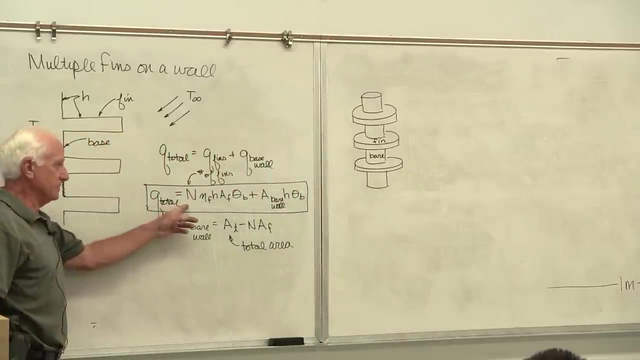 So let's put it here. Now you can do the same thing for a circular fin. This is the bare wall exposed to the convection. This is the fin surface. of course here, Just see me quick. It still holds. How many fins are there? Capital N. 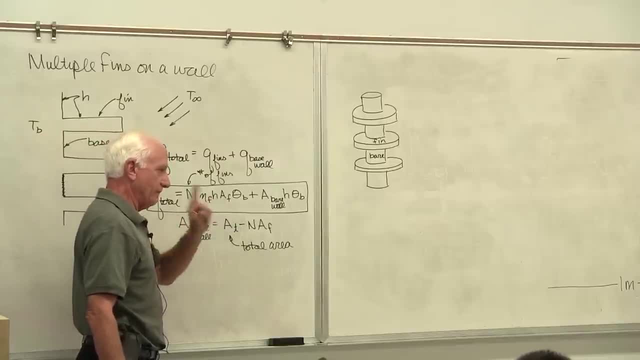 AF is the fin area of one fin. Now AF is the fin area of one fin. N takes into account how many fins there are And the bare wall is the wall between the two adjoining fins. The bare wall is the area between the two adjoining fins, So no matter what the geometry. 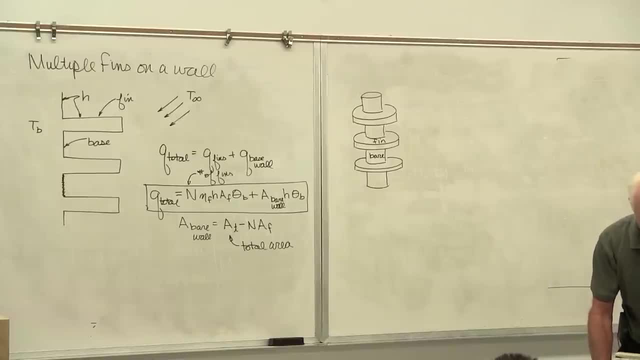 is: you go ahead and use that equation And then you go to table 3-4, table 3-5, table 3-6, table 3-7, table 3-8, table 3-9,, table 3-10,, table 3-11,, table 3-11,, table 3-12, table. 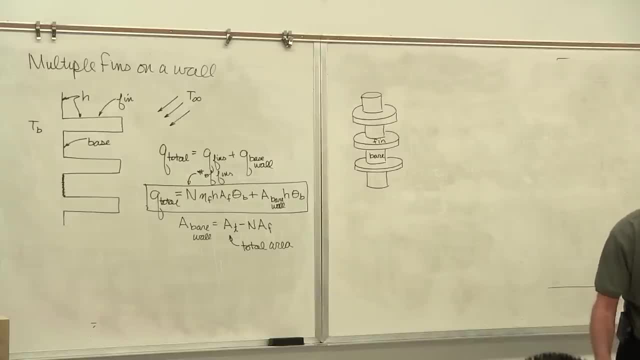 3-13,, table 3-13, table 3-14,, table 3-14,, table 3-15,, table 3-16,, table 3-17,, table 3-18,, table 3-19,, table 3-20, and either get the efficiency or the heat loss by one fin. 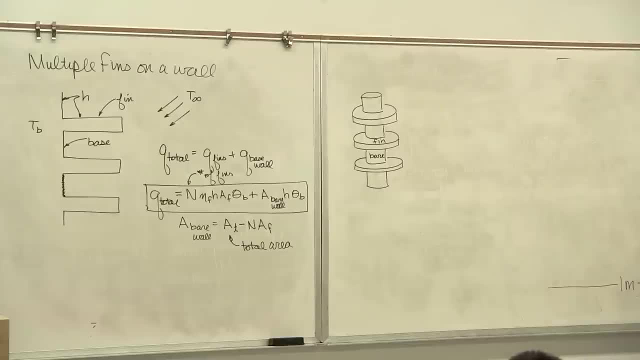 Okay, any question on that? And you've got. I'll give you one problem for homework. One involves circular fins and one involves rectangular fins for homework. Okay, now, that pretty much ends up our chapter 3.. I'm going to start chapter 4 right now. 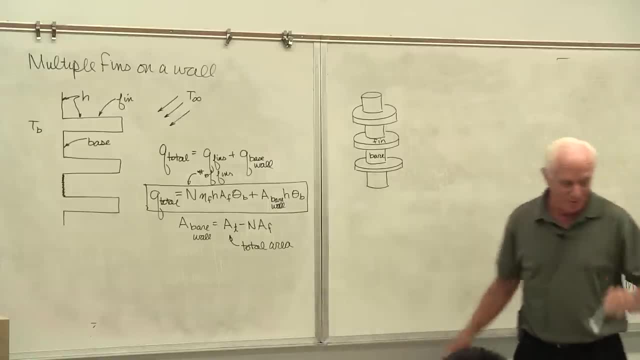 for about 10 minutes. But I'm just telling you that anything I do this week on chapter 4 is not going to be on that midterm next Monday. So you know what I do now, today and the rest of this week in chapter 4, keep it in your notes. but nothing on the first. 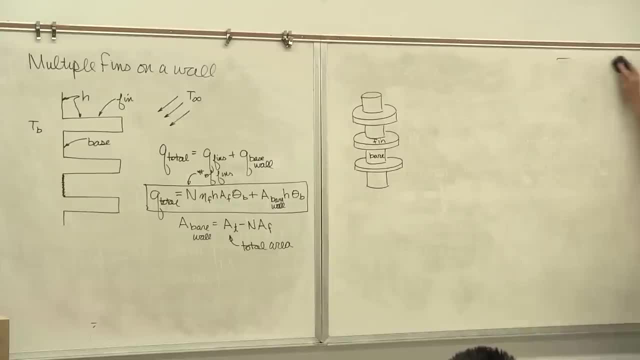 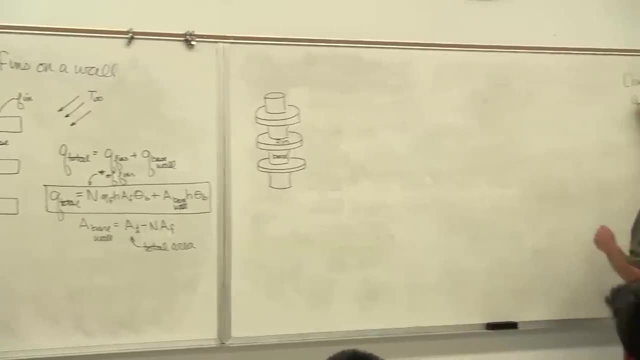 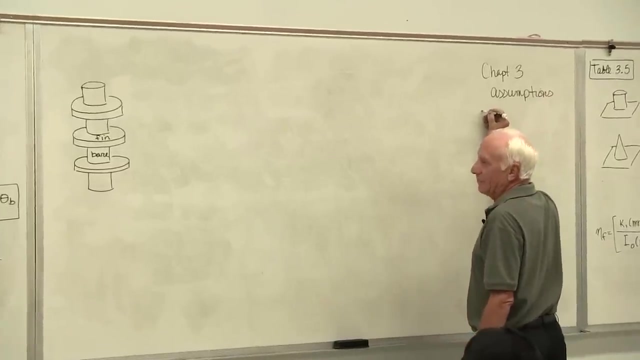 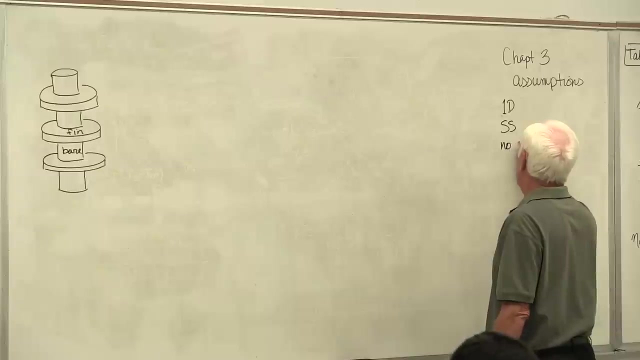 midterm from chapter 4.. Alright, so let's go back and look at chapter 3, what we assumed. So chapter 3, assumptions: Okay, first of all, we had 1D heat transfer, Then we had steady state, Then we had no. 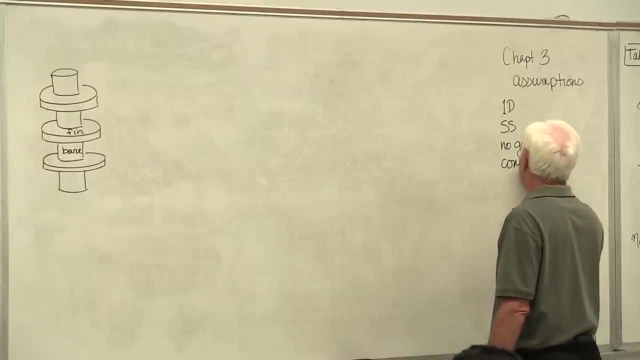 generation. Then we had constant properties. When we get to chapter 4, we start relaxing some of those assumptions. Now we say What? Most things in the real world are 2-dimensional, not one-dimensional. So we're going to say: 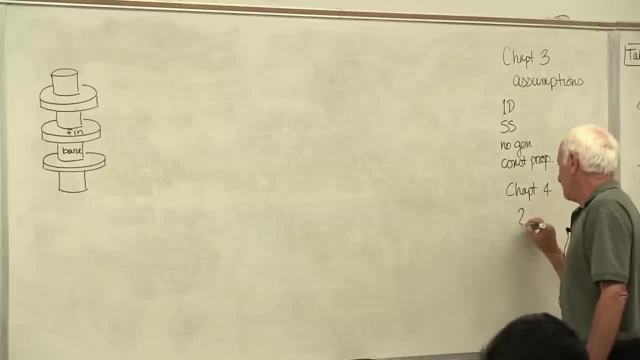 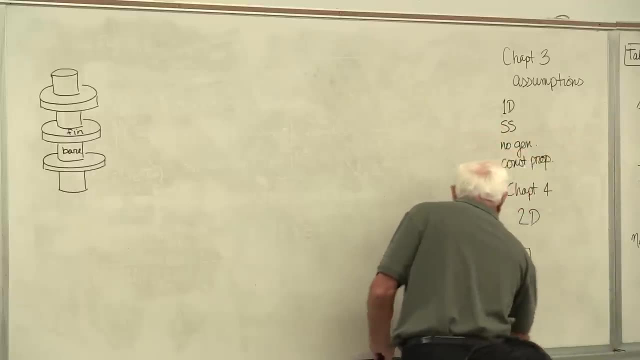 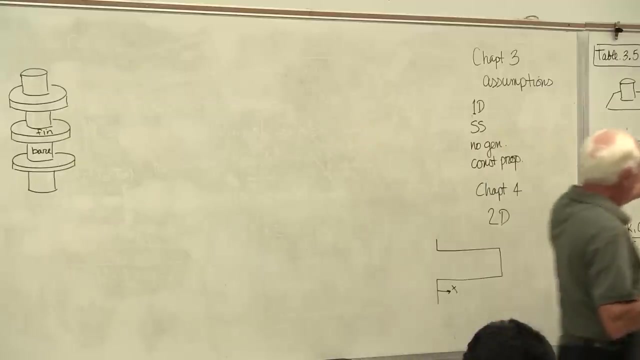 in chapter 4, now we're going to study 2D heat transfer. You know, in chapter 3 we had a fin And we said that, and that's right up here. We said that the temperature, this is T minus T infinity over T minus. 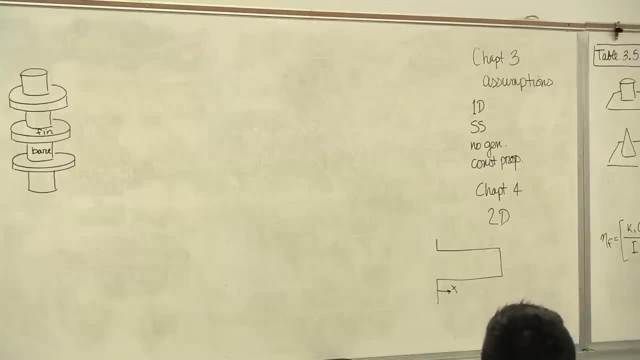 base minus T infinity. We said this gives us a temperature as a function of X. X is in the equations. So we're assuming 1D heat transfer. Well, you know that can't really be true. Sure, there's going to be heat transfer that way, but do you think there's going to 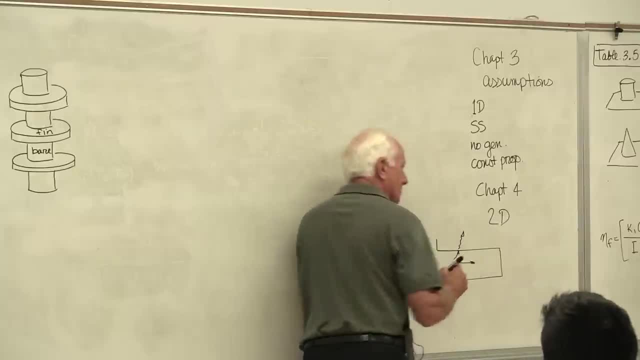 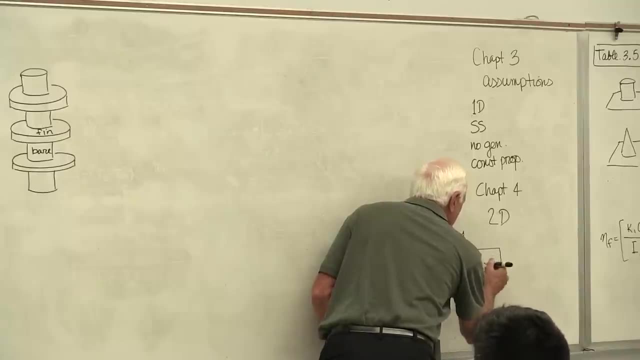 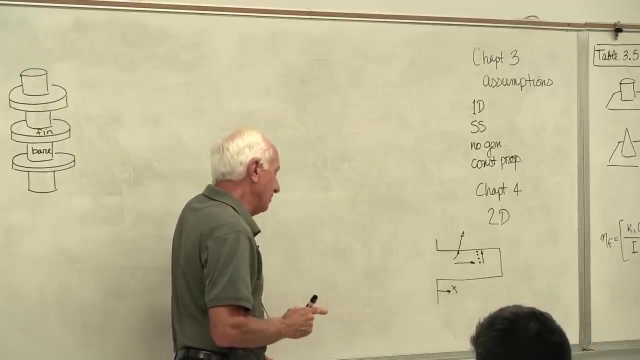 be some conduction this way and gets out by convection? Of course there will be. If it goes out that way, there has to be a temperature difference as you go towards the outside edge top of it. There has to be a temperature difference or there won't be any heat loss. 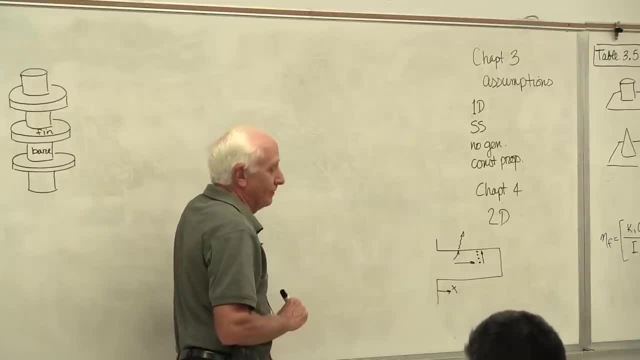 out of that top edge Conclusion: Oh okay, T must vary as a function of X and also maybe of Y. Right, exactly. But in Chapter 3, we make a good assumption for fins that generally we can assume fins to behave in a one-dimensional conduction, But in reality it's 2D conduction. 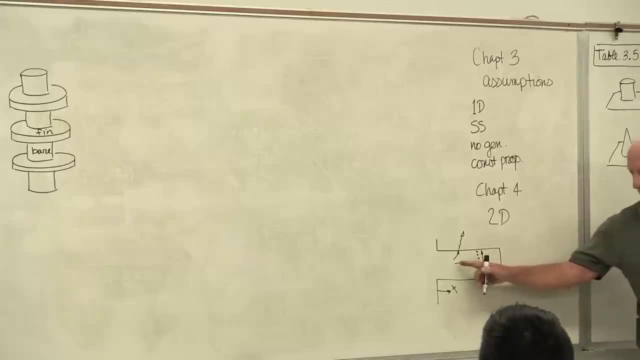 As a matter of fact, when you do your first computer problem, I'm going to tell you that you're going to have to get the temperature as a function of X and Y in a fin, which is a Chapter 4 type problem. So here's what we're looking at in Chapter 4.. We're going to look. 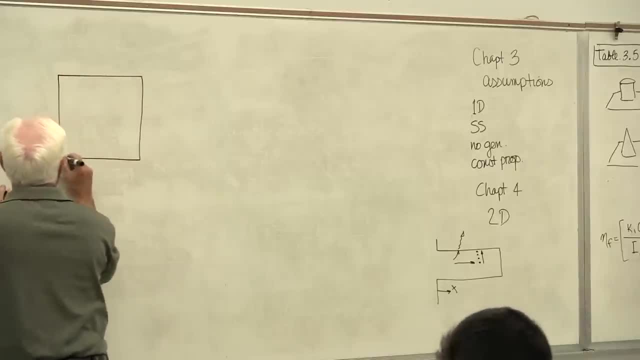 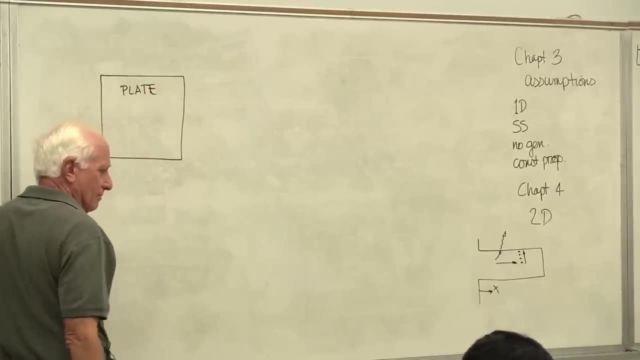 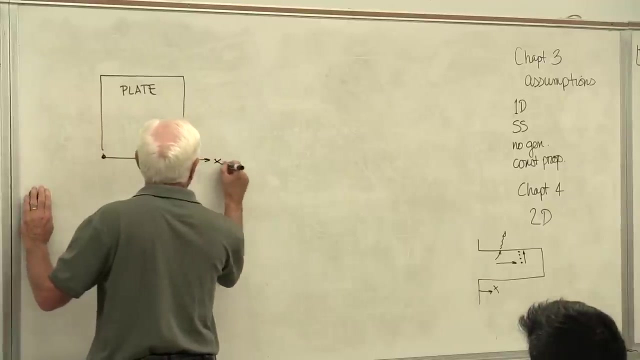 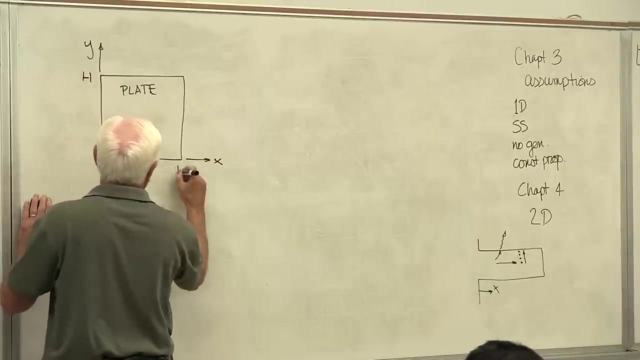 at, for instance. this is just an example. Here's a plate. It might be copper, it might be aluminum, one-eighth inch thick, quarter-inch thick. whatever It's a plate, We'll call it a plate. We'll call it a plate, And this is the quarter-inch thickness of a plate. 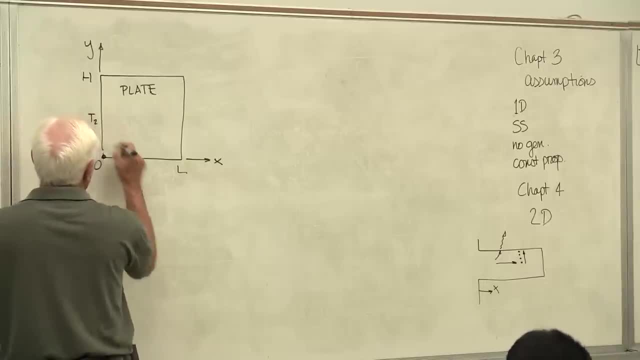 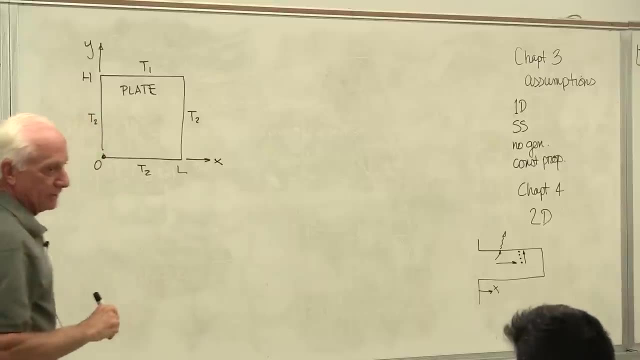 Now what do we have there? So this is an X and there's a quarter-inch thickness here. this will be the height of this plate, or this will be a quarter-inch thickness. Now I'm going to call these point lengths. I'm going to say, for example, I'll say let's let the left-hand side be T2, the bottom of the plate T2, the right-hand side T2.. The top T1.. I don't care which one's hotter or colder, If you want to say T1's hotter than T2.. That's fine, All right. 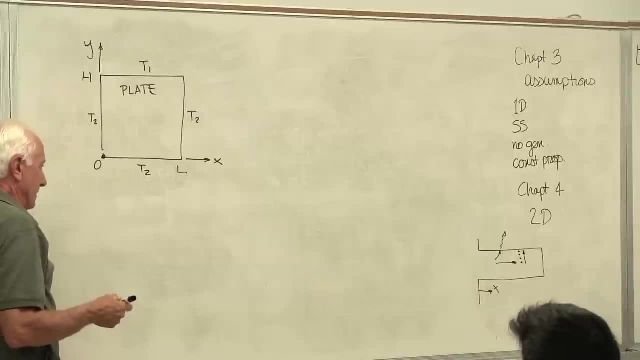 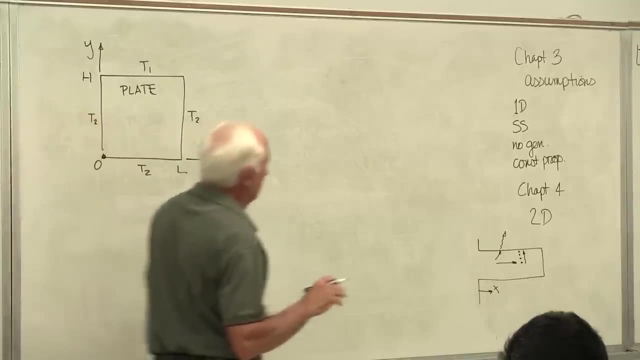 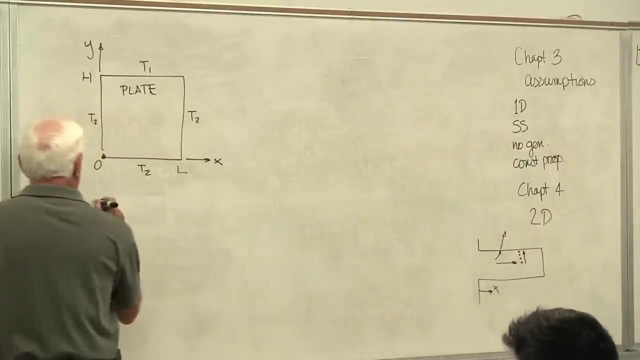 Go back to Chapter 3.. All right, go back to chapter 2, the heat conduction equation in rectangular coordinates. Get rid of everything. Steady state, no generation, constant properties, but let it be 2D What you're left. 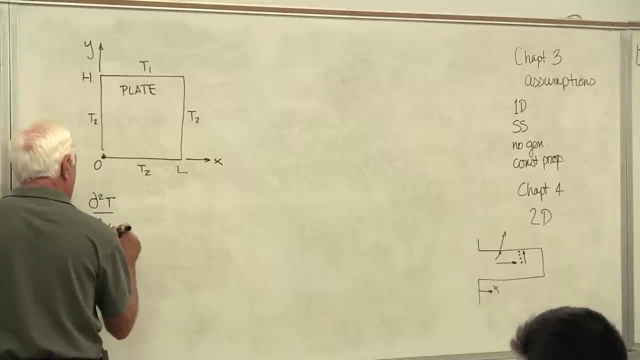 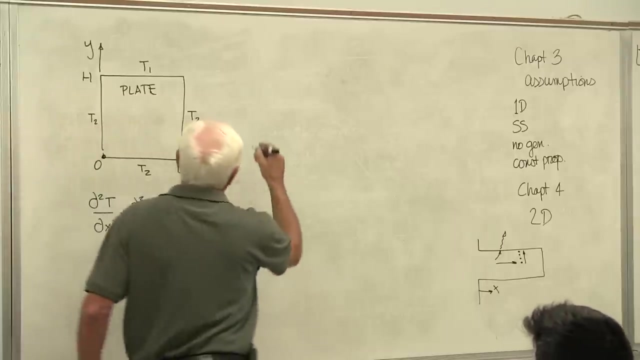 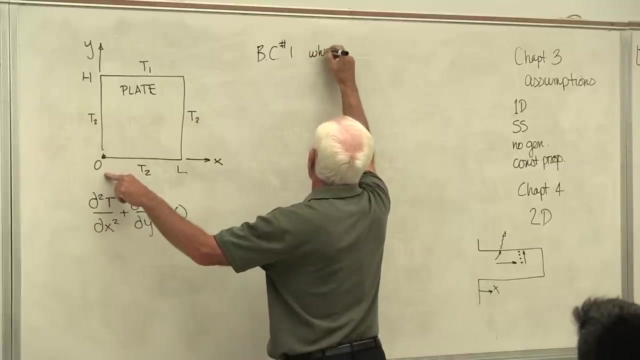 with is the classic Laplace equation. There it is, chapter 2.. Now we want to solve that, but before we solve that we need to get two constants, two boundary conditions: 2 in x and 2 in y. Okay so, BC number 1. When x equals 0, the temperature for any y is T2.. 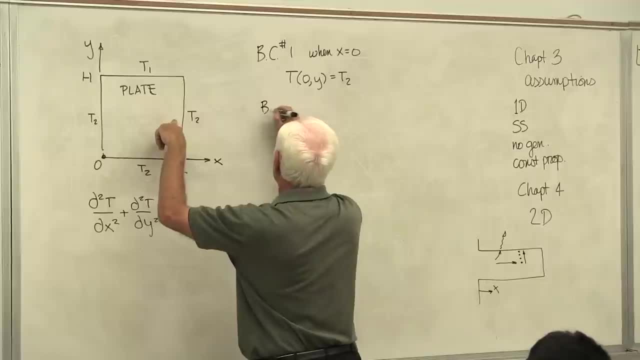 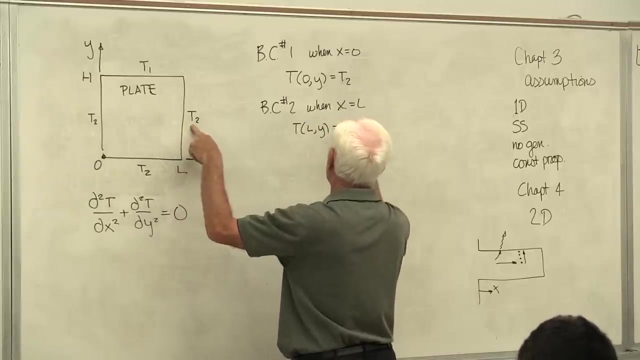 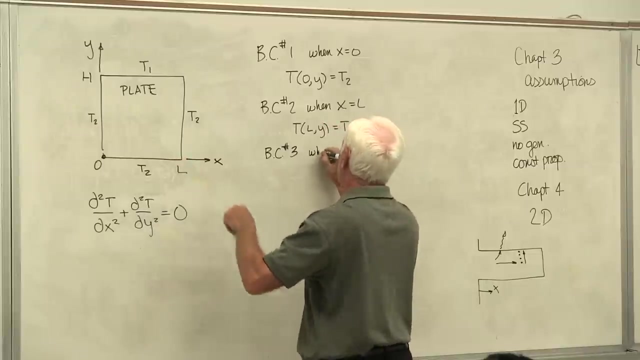 Okay, Other side, right side, BC number 2. When x equals L, T, x equals L for any y, T2.. BC number 3. When y equals 0, put your finger on it, temperature is T2.. 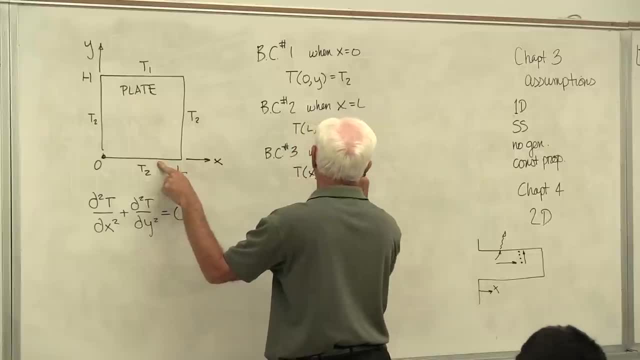 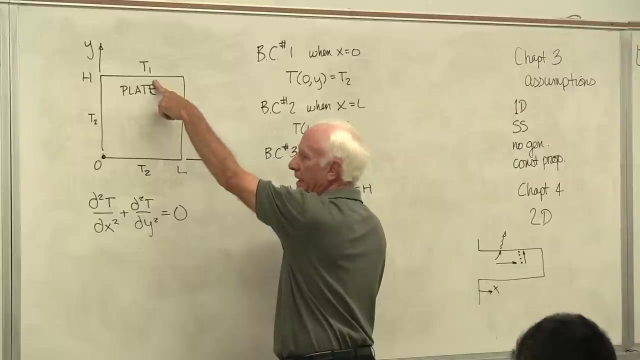 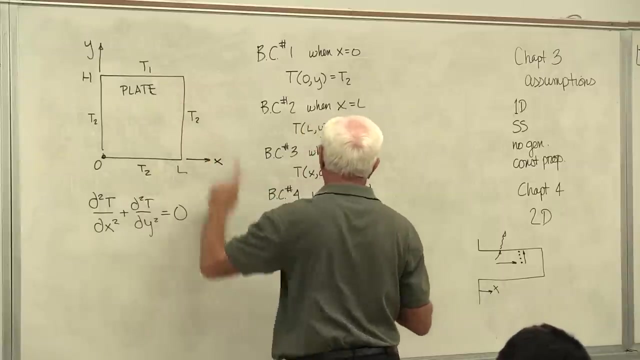 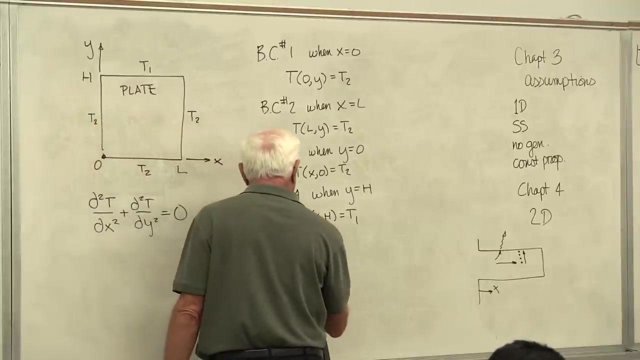 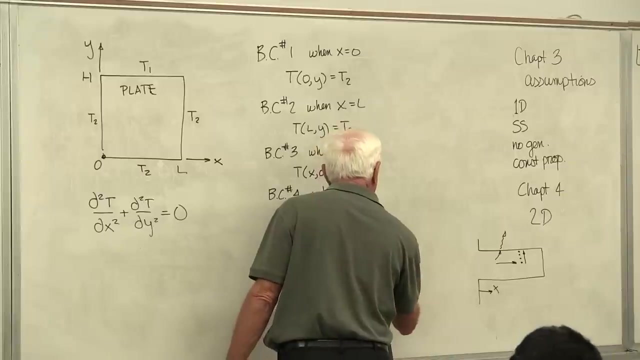 BC number 4.. When y equals H, put your finger on it. T is T1 for any x. There's the 4BC. There's a partial differential equation. It can be solved. For what's the idea? Get the temperature as a function of x and y. 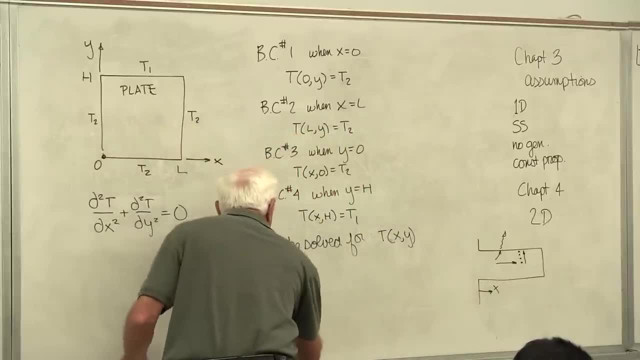 That's what you want to do Now to solve that in general. maybe you want to do it analytically, Or maybe you have to do it analytically, Or maybe you have to do it analytically, do it numerically, And maybe it's possible to get a real rough estimate graphically. 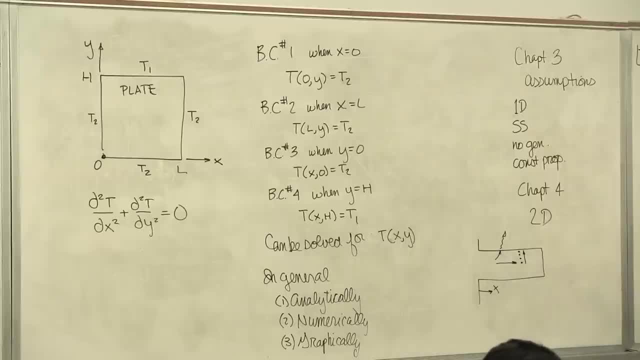 So there's different ways to solve that. We're not going to do any of the analytical ways. They're restricted to simple geometries and even for simple geometries it's not always possible. You do that in the graduate course here at Cal Poly in conduction heat transfer. 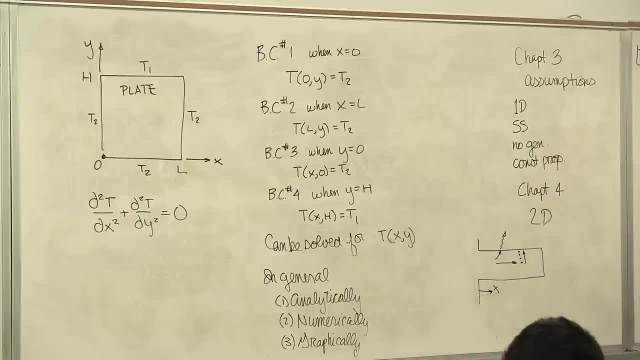 Numerically. yeah, that's probably a lot of the preferred way nowadays. We're going to do one. I mentioned the fin. We're going to do one at the end of Chapter 4 for a fin numerically And we're going to look briefly at what the graphical solution can tell us. 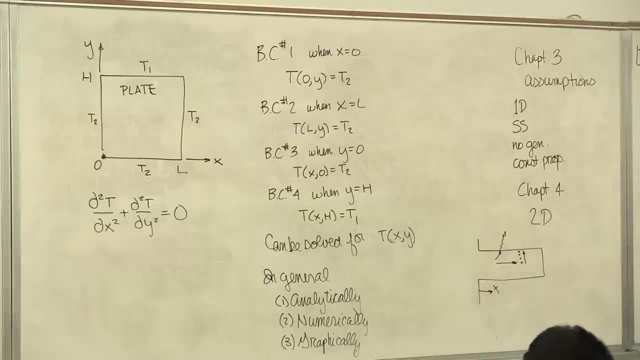 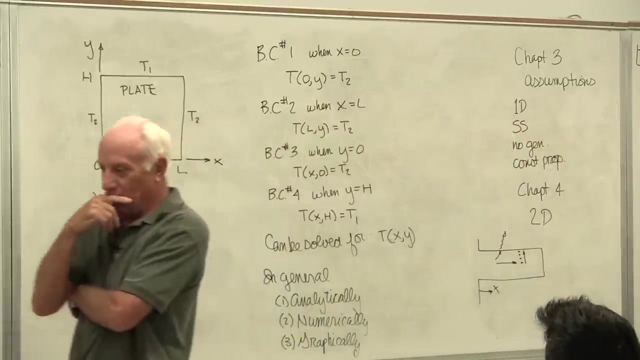 or help us understand the problem. So three possible solutions, Three possible ways there. If you take the graduate course, you spend a lot of time on numerical methods and you do go through some of the analytical methods, and that's four hours a week, times ten weeks, roughly 40 hours, And we spend what? two class meetings, two. 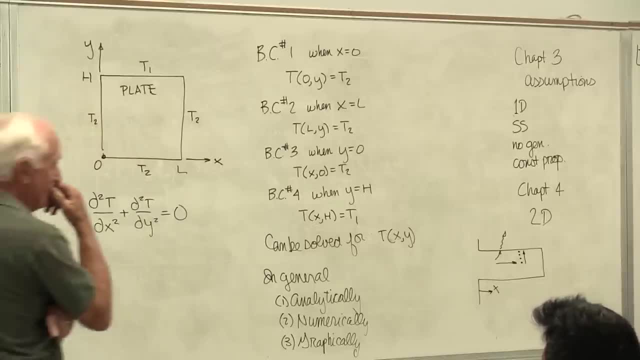 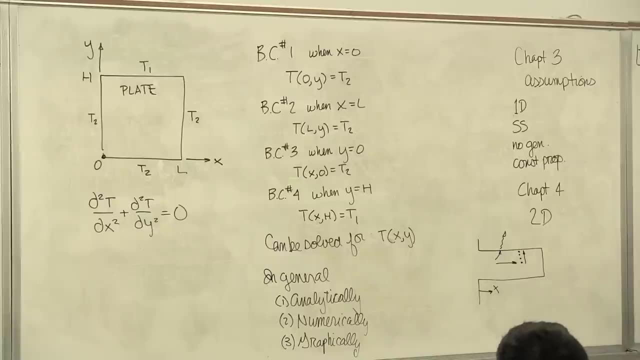 times 65, you know an hour, two hours and ten minutes on this stuff. So, oh yeah, we're just barely scratching the surface. If your area of interest is in thermal sciences, as in me, oh, you take a ton of stuff in the 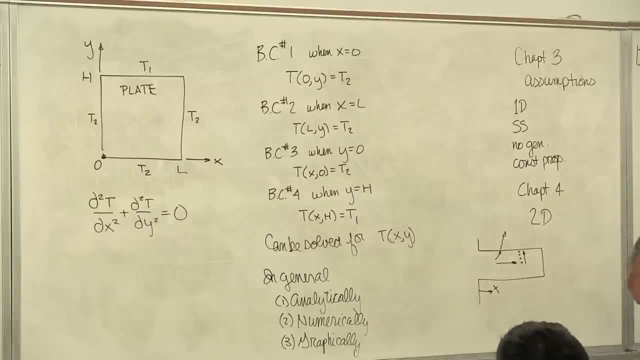 graduate courses. There's a course in conduction, heat transfer, one in convection, one in radiation. Okay, That's 120 hours. right there. You take advanced fluids, advanced thermal, You take boundary layer, You take potential flow. Oh wow, viscous flow. There's another 120 hours. 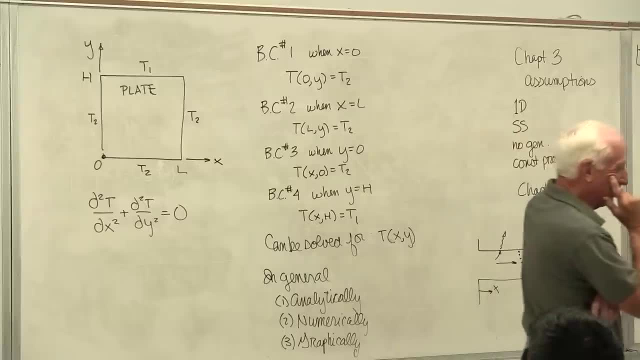 240 hours now of your life. Yeah, So, and how long are we spending? Oh, we're spending ten weeks, you know, three hours a week. So no, we're not almost four hours a week, We're just scratching. Take, 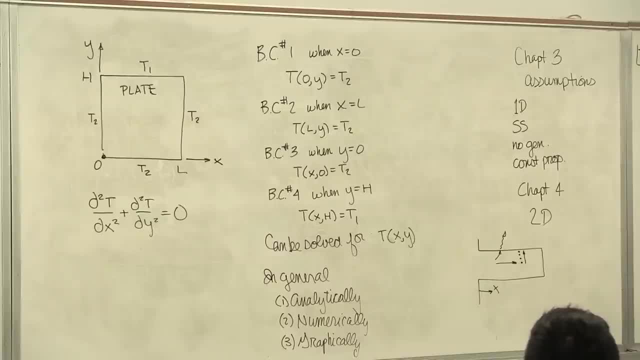 off two holidays, Take off two exam days. What are you left with, My gosh? you're down about eight weeks now, and the first day isn't that much. So you know, we're barely scratching that, So that's, we can't get into depth there. Okay, Now, that's probably a good stopping. 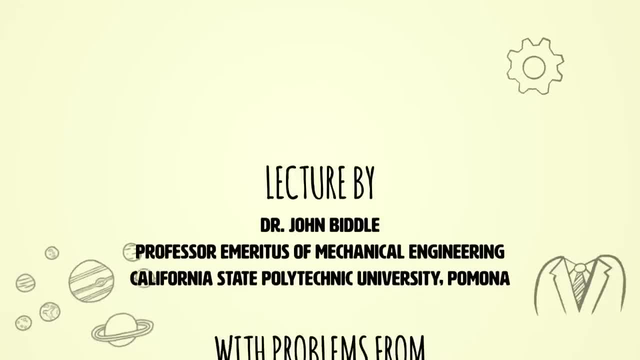 point for right now. We started chapter four. Okay, All right, Thank you, Bye-bye, Thank you, Bye-bye, Bye-bye. 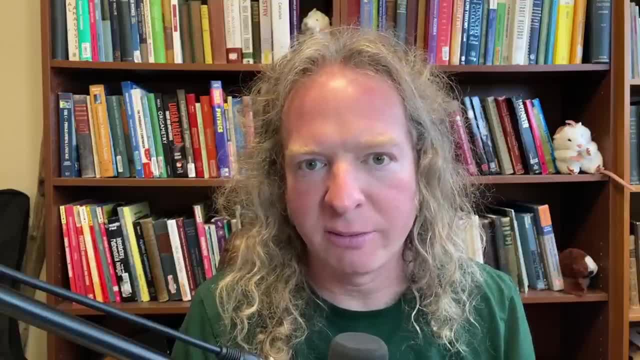 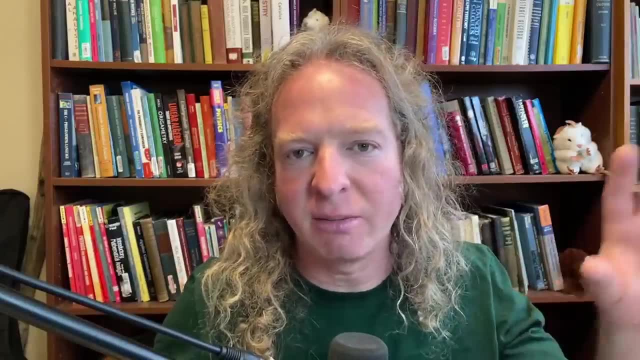 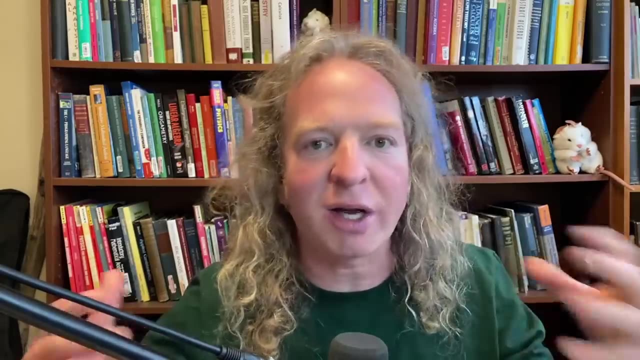 Math does not prepare you for the real world. This is something that people always say. I hear it so much. I used to see this little thing pop up on Facebook. It was a picture of an older gentleman and he was sitting back in some rocking chair and it said something like: 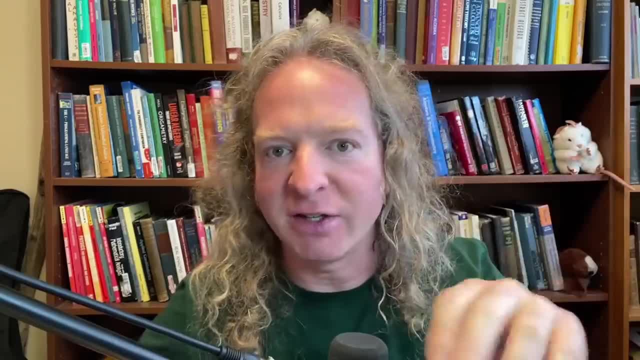 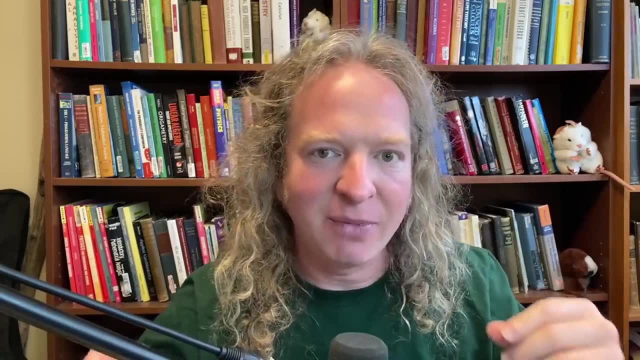 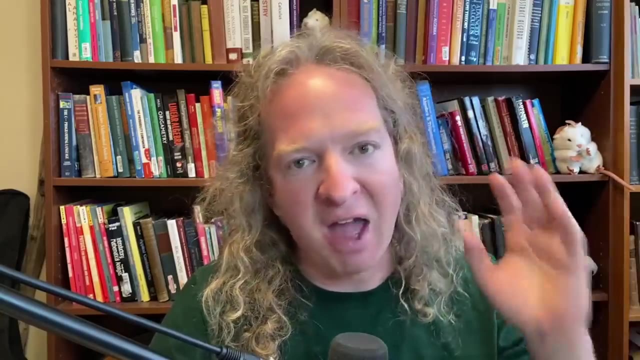 why teach algebra when you can teach finance and real life skills? And the guy was older and he was a little bit overweight And I guess that was like trying to indicate that he has some special knowledge, because he's older, that other people don't have. I hear it all the time: Math. 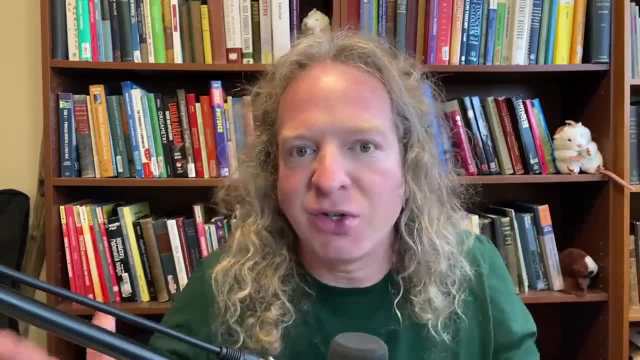 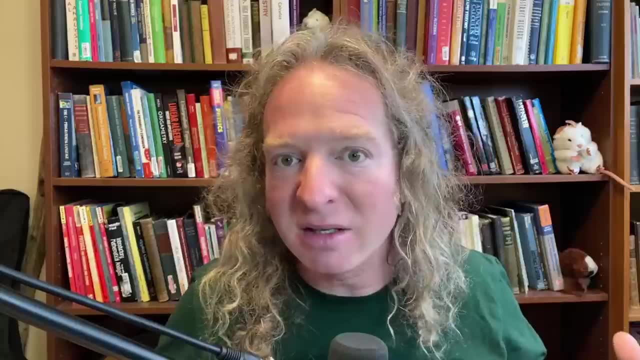 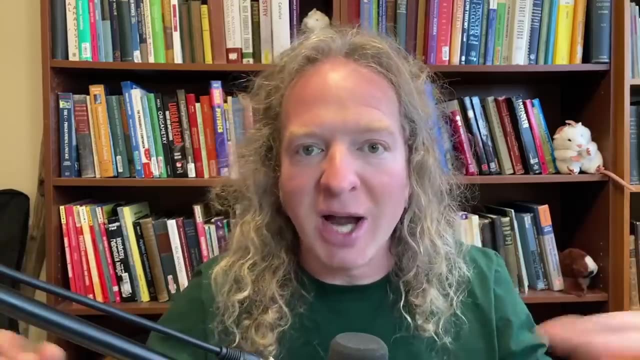 does not prepare you for the real world. Instead of teaching math, you should teach real world skills, Teach job skills. So let me say this: What is the real world? What is it If you get a math degree and you get a job, say, as a middle school teacher or a high school teacher? 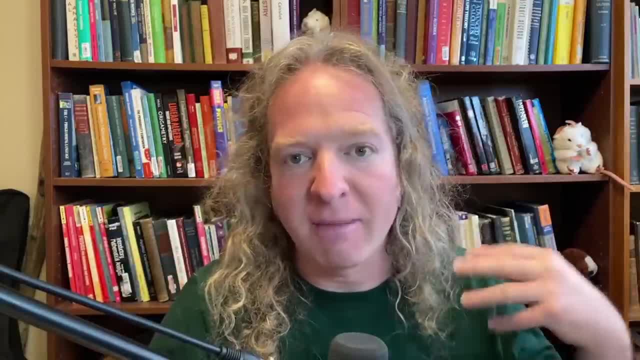 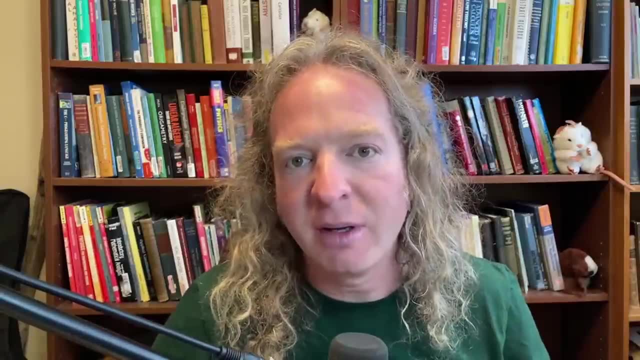 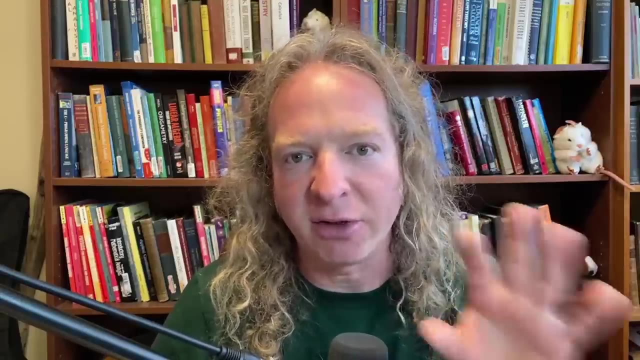 that's your world. That's what you do If you get a math degree and you get a job working at a bank. that's what you do. That's your real world. So people saying that math doesn't teach real world skills- I think the argument is completely flawed, Because what is the real